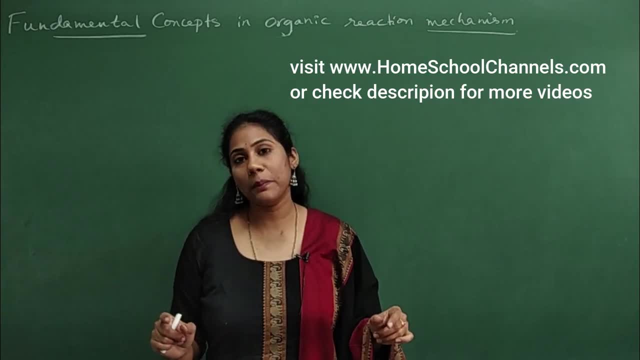 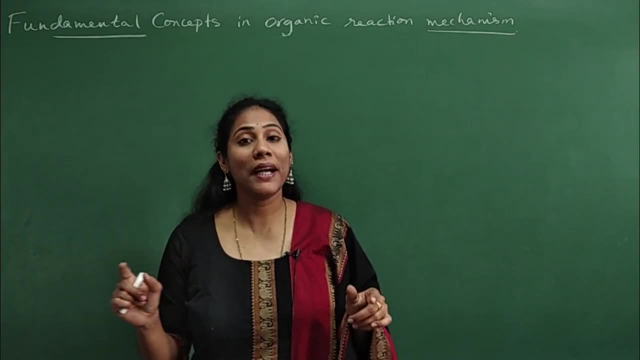 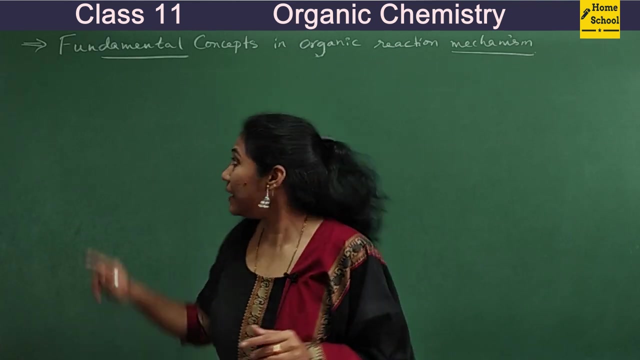 branches: nomenclature of unsaturated hydrocarbons. nomenclature of organic compounds with functional group. nomenclature of aromatic compounds, alicyclic compounds, right. So now I have come to a topic very, very important to understand, that is, fundamental concepts in 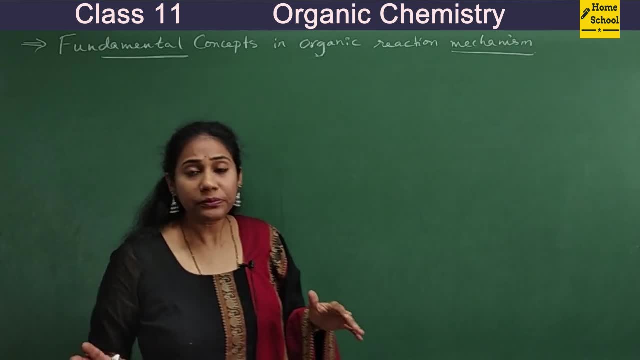 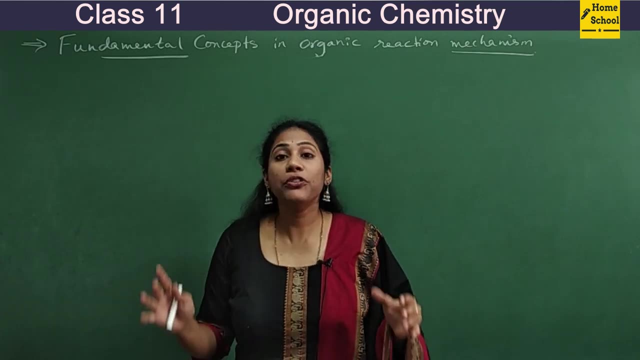 organic reaction mechanism. See, organic reactions are very, very important and they do happen in a certain way. So I am going to talk about organic reactions. So I am going to talk about organic reactions in a certain way. You need to understand the logic behind the reaction, right? So there are. 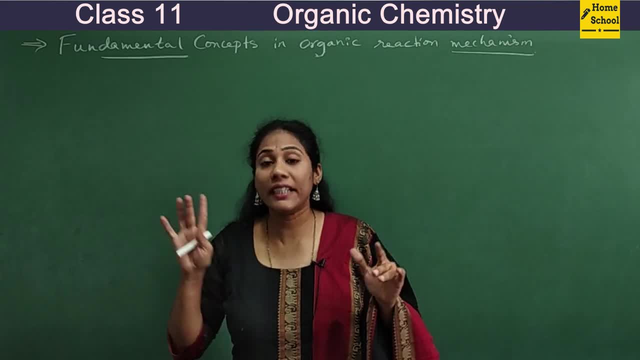 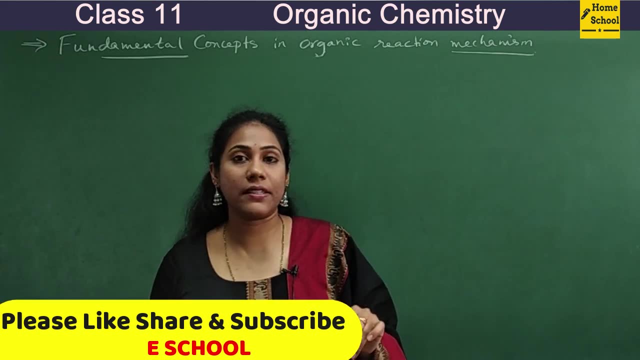 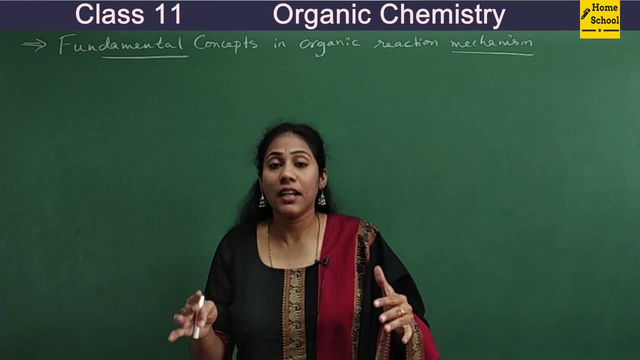 many basic, fundamental things that you have to understand before we actually study organic reactions and organic reaction mechanism. okay, So reaction mechanism is nothing but a step-by-step process, that a reaction takes place in a certain way. okay, So that is what we mean by reaction. mechanism. So we need to understand the logic behind the reaction. So there are many basic, fundamental concepts that you have to understand before we actually study organic reactions. So I am going to click into the people and the factors involved in what we are waiting to understand and create a reaction. 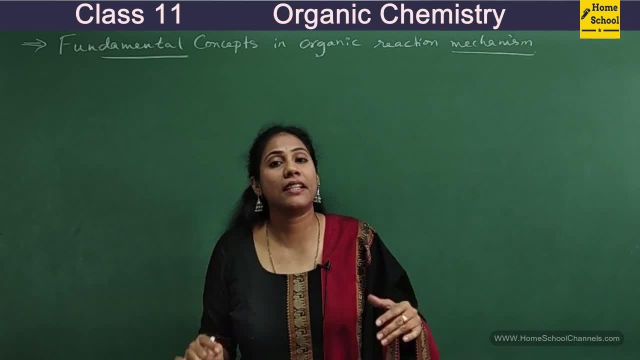 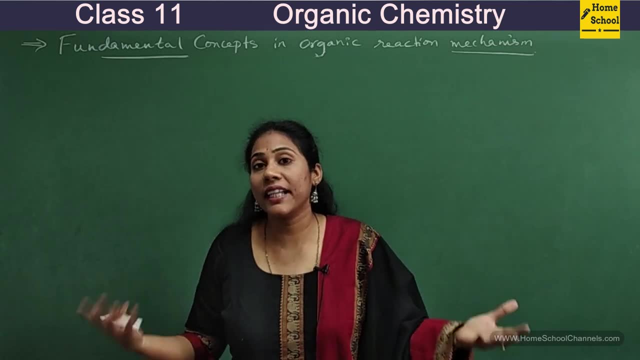 mechanism. So then I want to give you an example of the mechanism you can follow. So in the basic, Four- artificially complex reaction box, there is simply a mechanism, a reaction mechanism. step by step learning of reaction is the reaction mechanism. So here I am going to talk about a general idea: how. 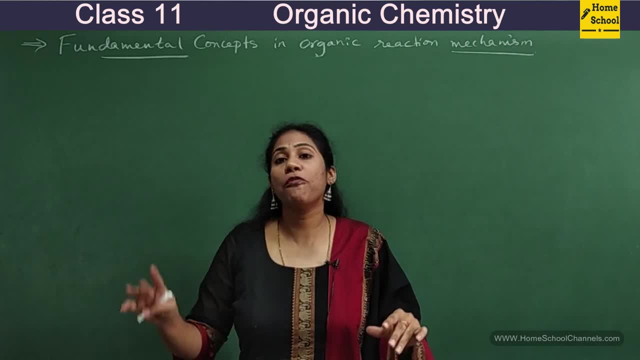 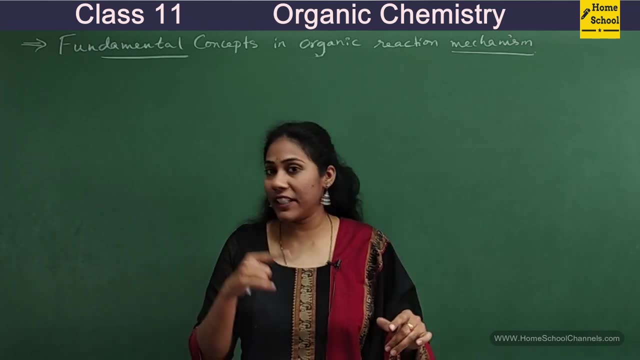 an organic reaction takes place, and there are two types of bond cleavages during organic reactions. One is homolytic cleavage, the other one is heterolytic cleavage. So let us understand these two types of cleavages first, and later we will talking. 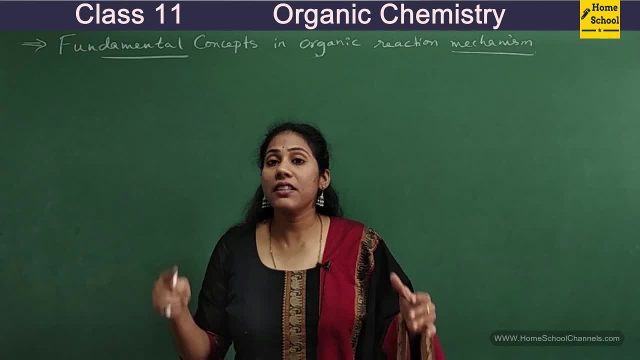 about the alleinic cleavage, and this is known as Transeswaric Cleavageer. yeah, let is. conversations is important, and later we will try to understand something about intermediates like carbocation, carbanion and free radical and, most importantly, we will also try to understand so called nucleophiles. 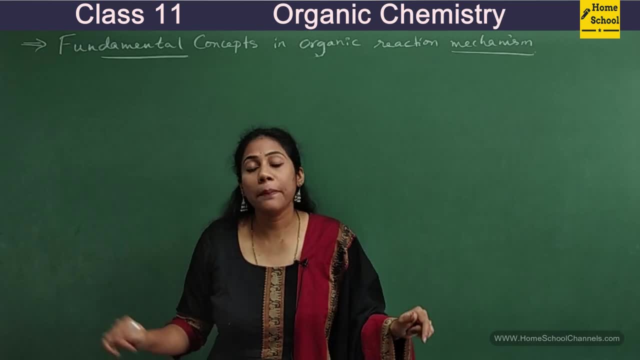 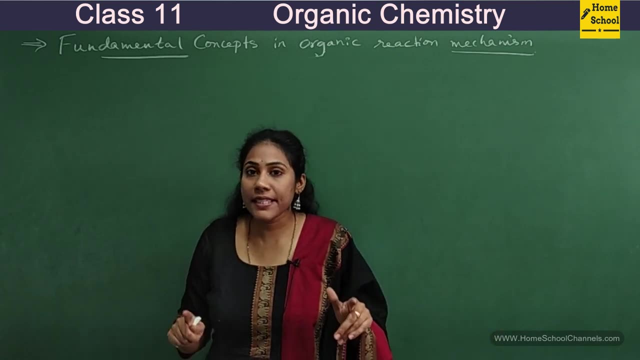 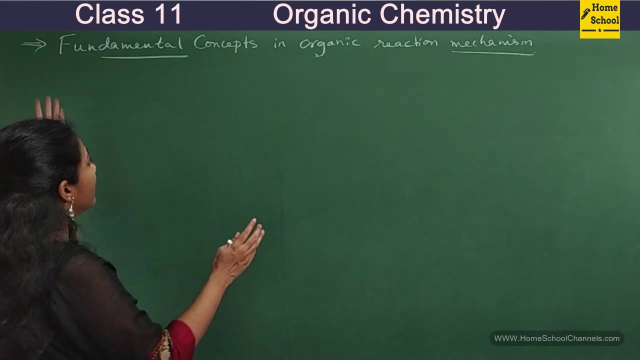 and electrophiles. okay, so this much is the concept i am covering in today's class, so do watch the video till the end. definitely all your basics regarding organic chemistry will become clear. okay, so coming to the organic reaction mechanism, this is, a certain way, the organic 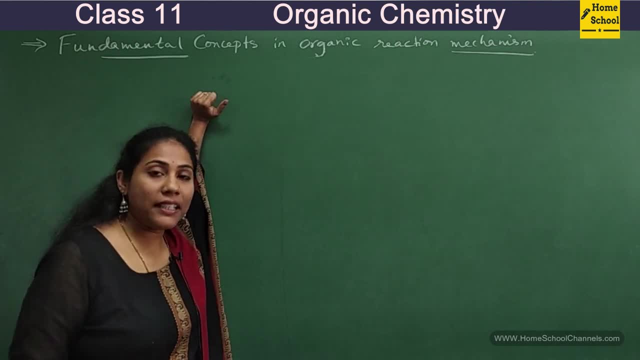 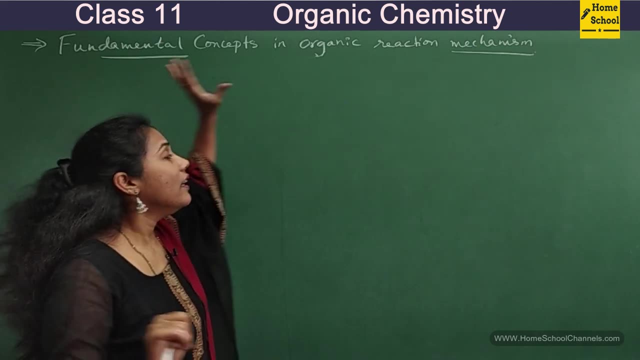 reaction takes place right. see, whenever you expect the chemical reaction, you have something in your left hand side that we will call it as reactants, and, and, and they react and you get a new substances which we call them as a free radicals. so this is the concept i am covering in today's class. 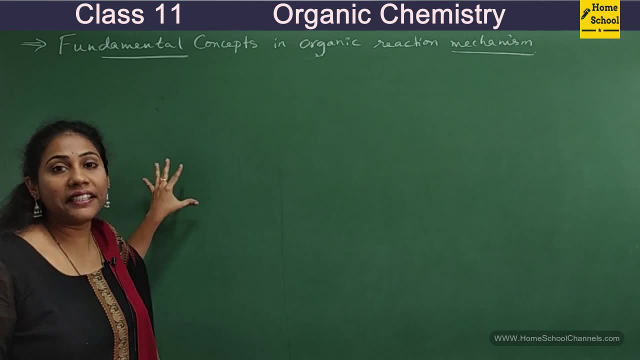 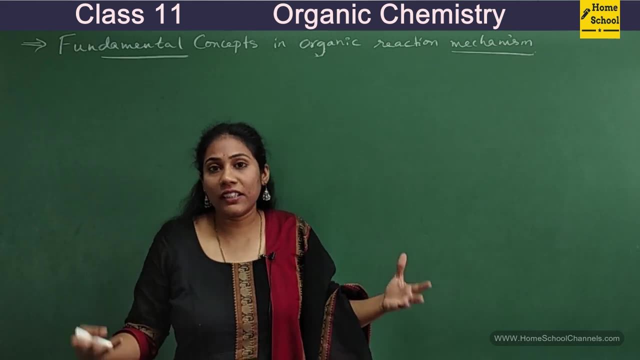 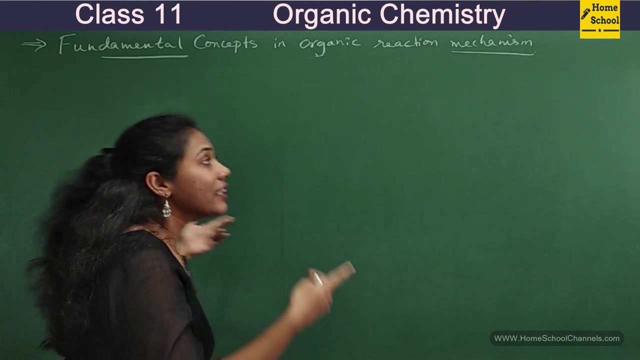 product right. so here also you have a reactant. there is a certain organic molecule that is going to be reactive or that is ready for the reaction. so such organic molecule, the main molecule that is going to react, is called with the name substrate. so here substrate is nothing but. 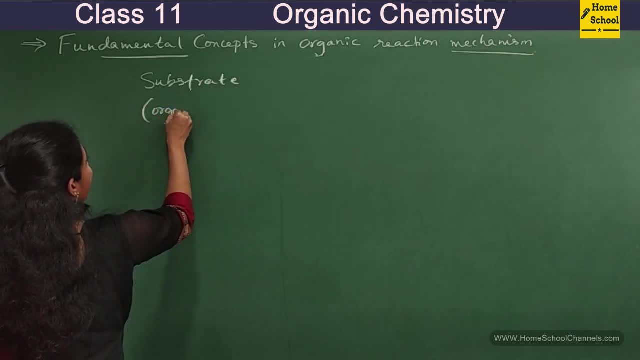 an organic reactant. okay, so organic reactant. one of the organic reactant is called as substrate. so this substrate is always, uh, you know, carbon containing compound. so organic compound when i say definitely do contain carbon, right? so, uh, some carbon containing compound which is ready for the reaction is called with the name. 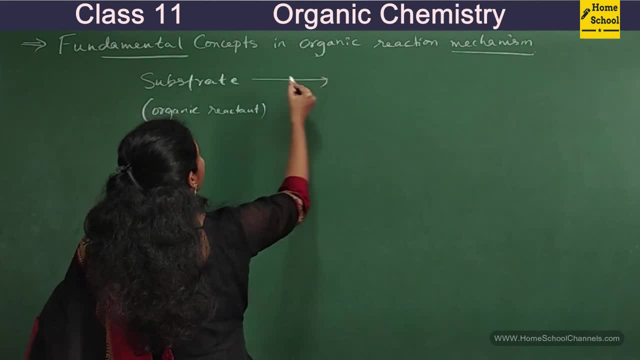 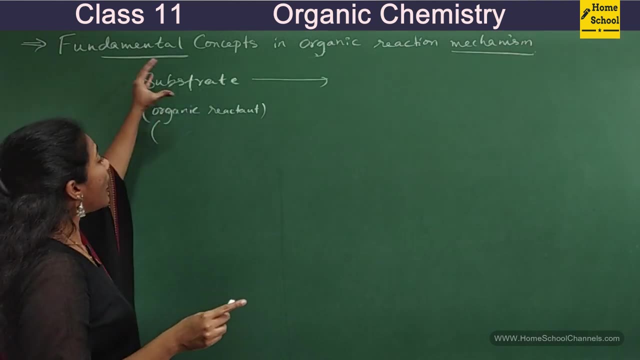 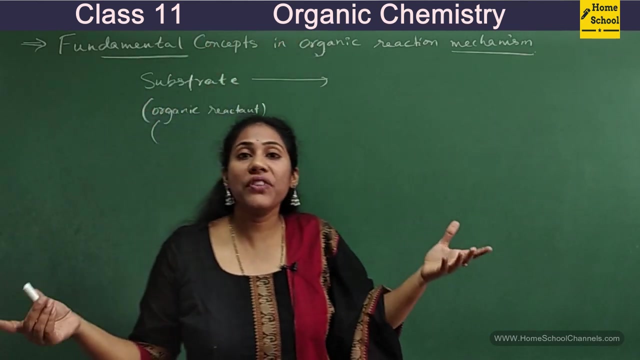 substrate right and then something must react, something must combine with substrate. only then you will get product right. so when do you observe a change in a substrate? when you add some other reactant. so reactants, most of the time you will expect two. there will be two reactants. 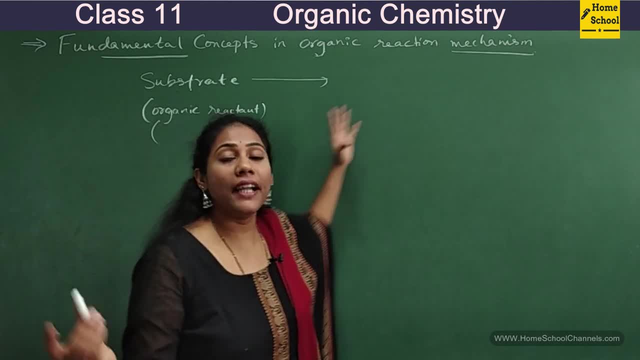 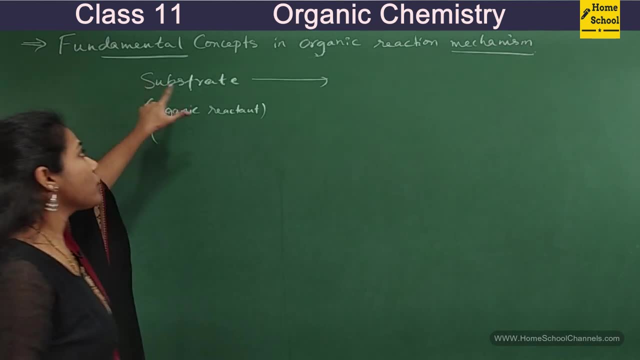 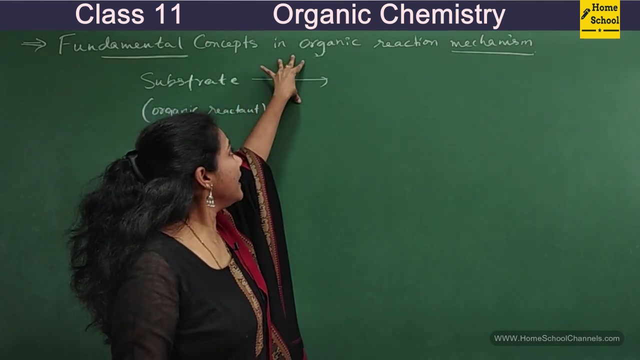 uh, this side, i mean in the left side- uh, they do combine and you get a product right. so, similarly, one of the reactant which is made organic compound was called as substrate, and the other reactant that you are combining with this, so the other reactant that is bringing some structural changes in the substrate, the other 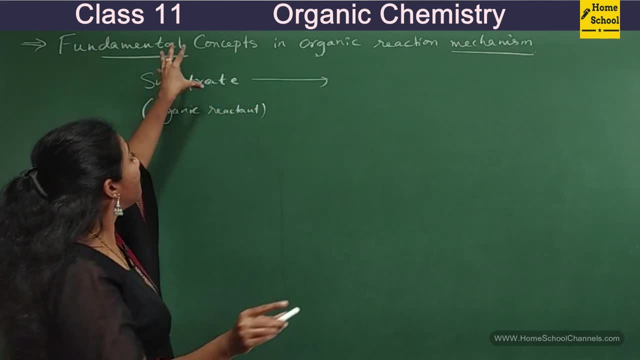 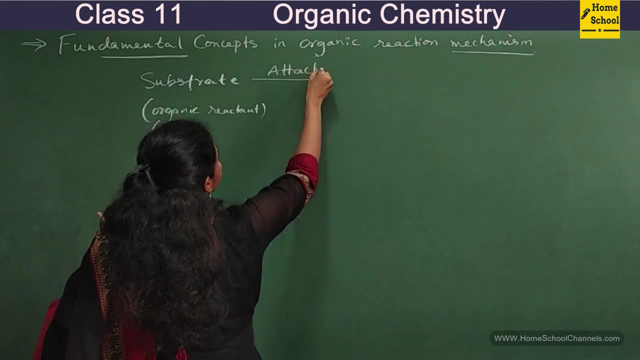 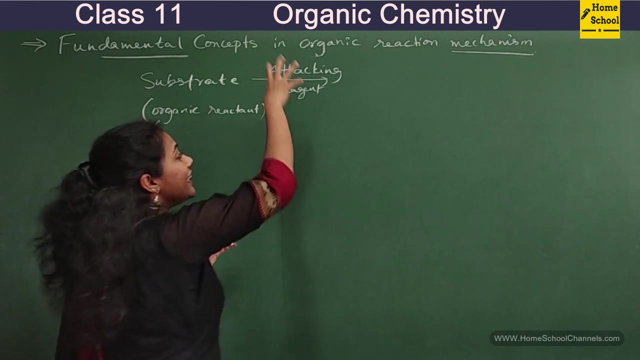 reactant that is responsible for the breaking of bonds in the substrate is called with the name attacking molecule. so this i will call it as attacking reagent. so there is some attacking reagent. so there can be two types of attacking reagent. we call them as nucleophiles and 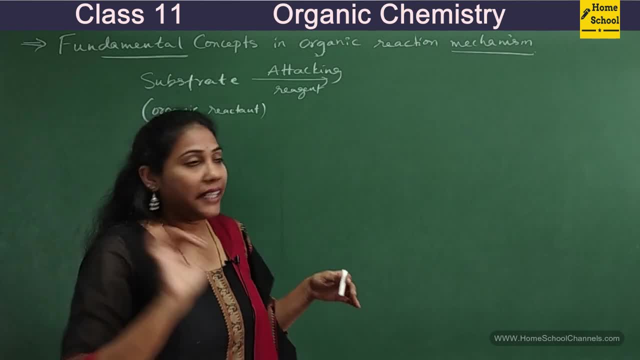 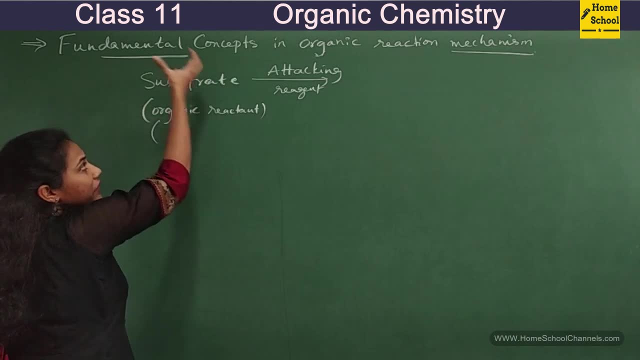 electrophiles. so this idea also i'll give at the end. okay, so when you add an attacking reagent there, you will expect- i mean where in the substrate? you will expect certain changes in the substrate and you will expect certain changes in the substrate and you will expect. 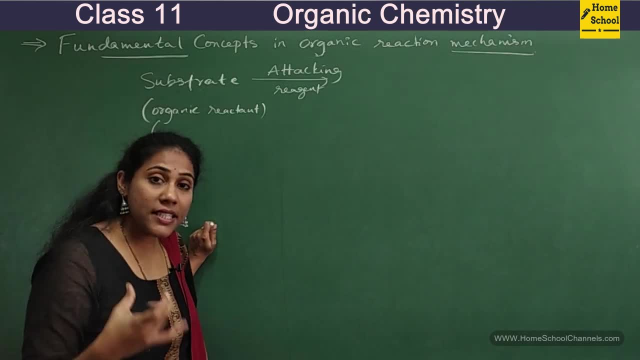 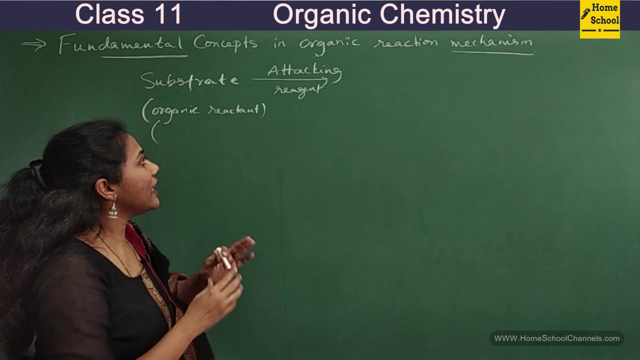 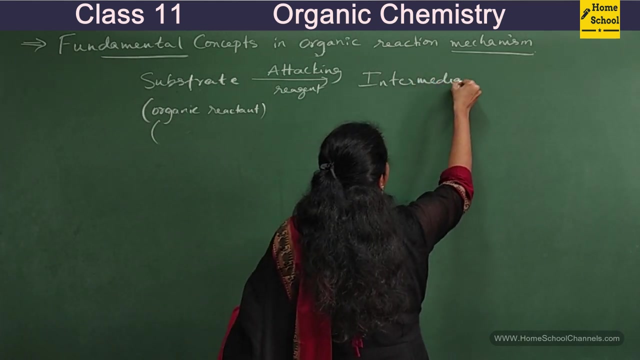 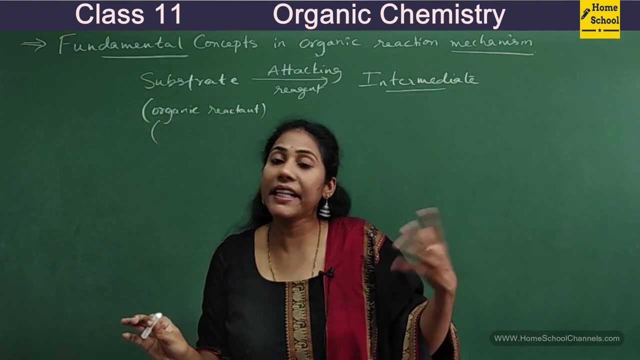 in the structure, you may observe certain bonds getting broken up right. so attacking reagent, so substrate combines with attacking reagent and you will observe the formation of intermediate intermediate, so organic reactions always involve one or the other intermediate formation. okay, so there are many types of intermediates actually. so all these 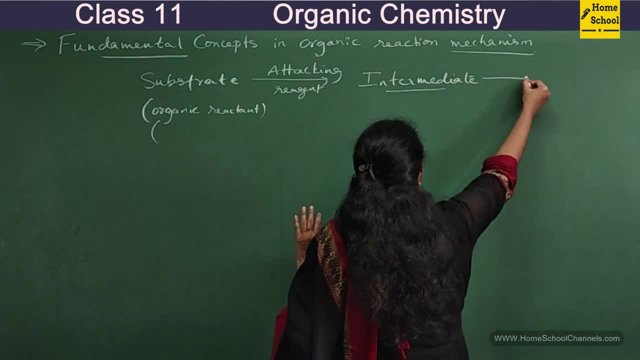 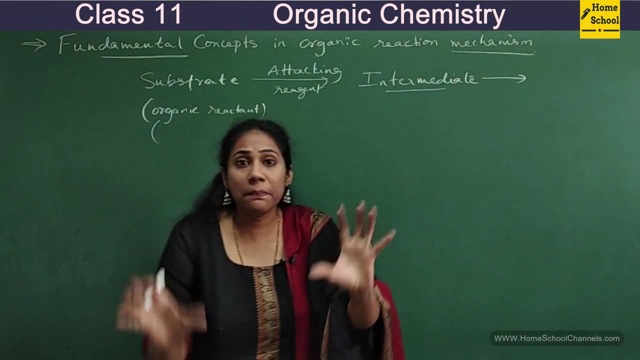 all these are the types of intermediates that are involved in the structure, so you can observe certain bonds getting broken up right, so attacking reagent, so substrate also we are going to discuss now. and intermediate undergoes some level of changes. okay, some bonds may break, or intermediate undergo some structural changes, or it may combine with other substances. 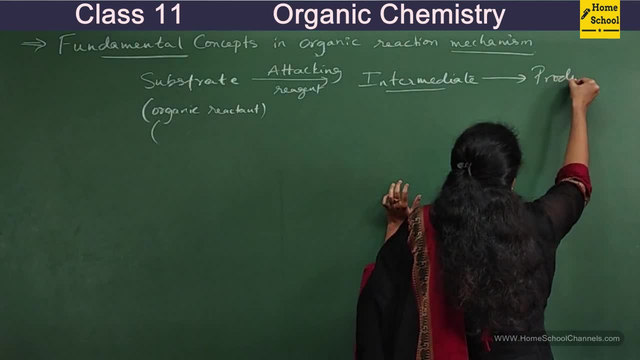 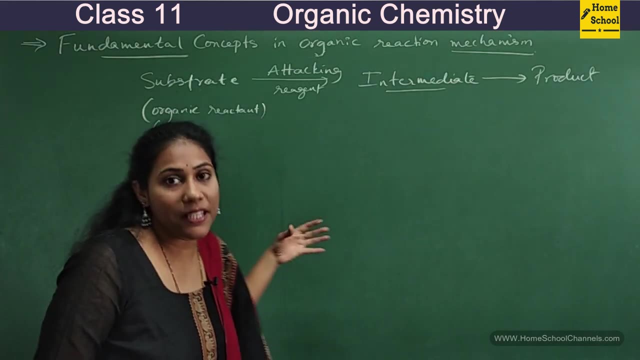 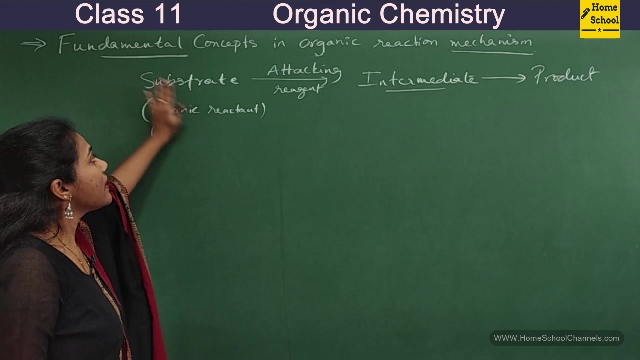 to give a final product, to give a final product. so this is, uh, the core idea how an organic reactions can takes place. so you have your main carbon containing compound, which we call it as substrate. so you will observe some bonds breaking up in a substrate or the 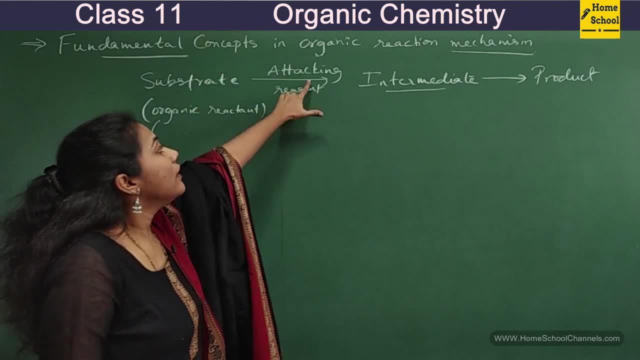 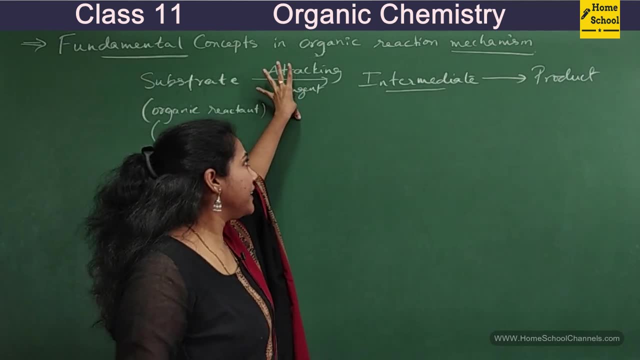 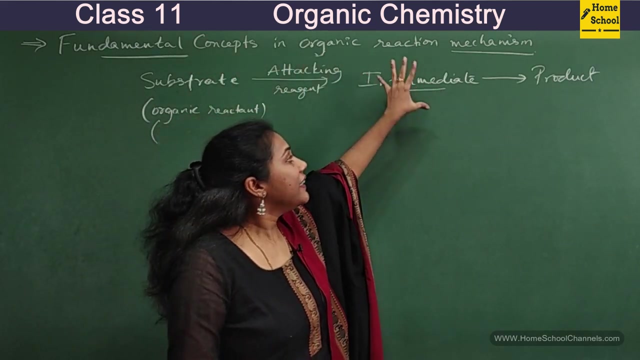 structure would change. uh, you know, when you give attacking reagent for this to react, uh, so attacking reagents are of many types, we will discuss that later- and uh, both of them, when they combine or when they react, you get so-called intermediate, and then this intermediate further undergoes. 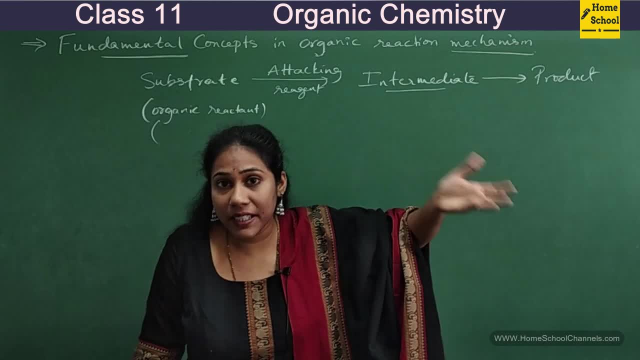 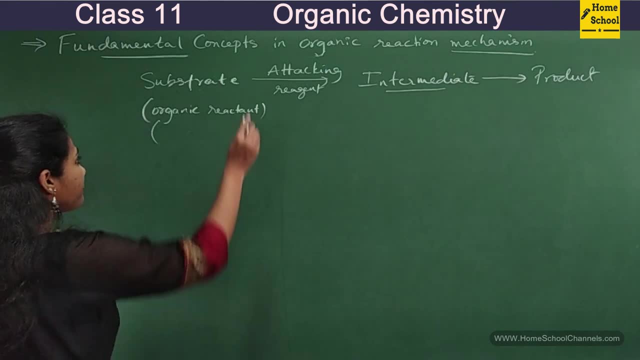 changes in their structure, or it may react to the structure and then it may give a final product which we call it as substrate. so you will observe some bonds breaking up in a substrate or the structure with some other stuff, and you will end up finally in getting product right. okay, so now, whenever you 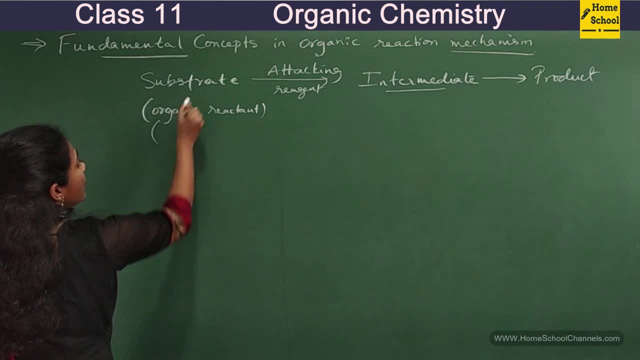 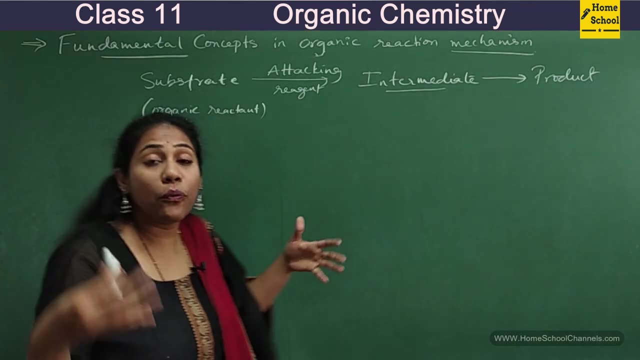 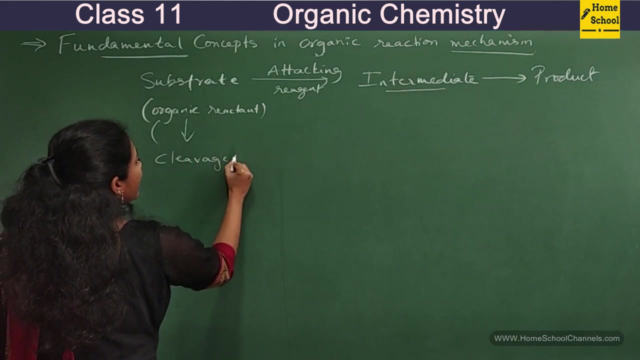 give attacking reagent for a substrate what I told you. substrate undergoes some breaking. you know some bonds in a substrate will break, okay. so you will observe certain cleavages- cleavage or cleavage of bonds in a substrate. when do you observe cleavage of bonds in a substrate? when you 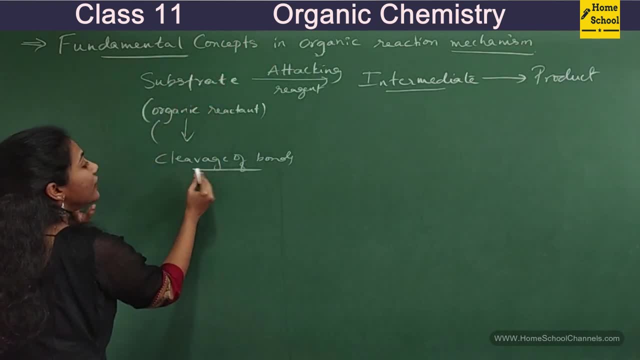 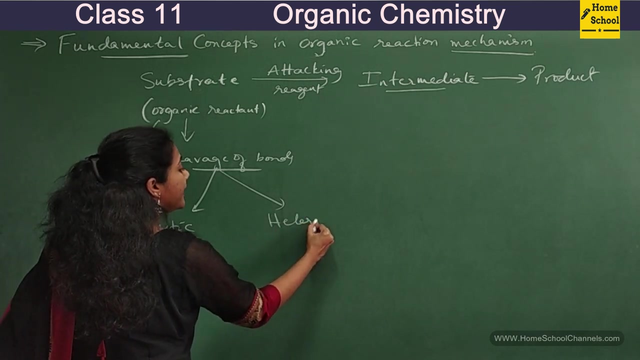 supply some attacking reagents. so there are two types of cleavages. usually, you will observe, with organic substrates they are homolytic cleavage, homolytic cleavage, and the other one is heterolytic cleavage. okay, so homolytic cleavage is the cleavage of bonds in a substrate. so you observe. 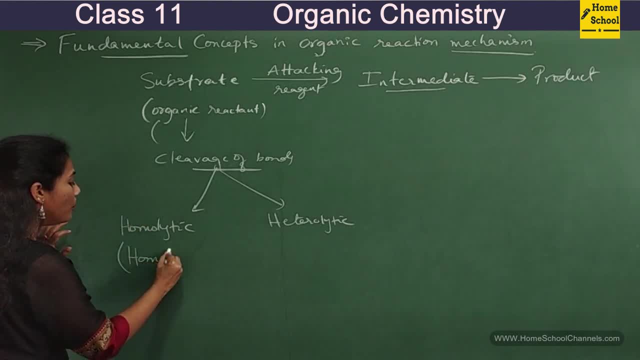 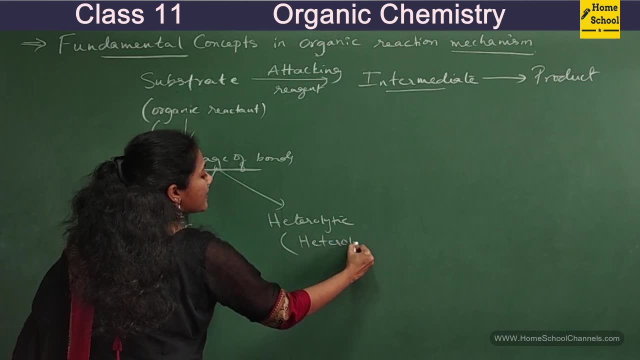 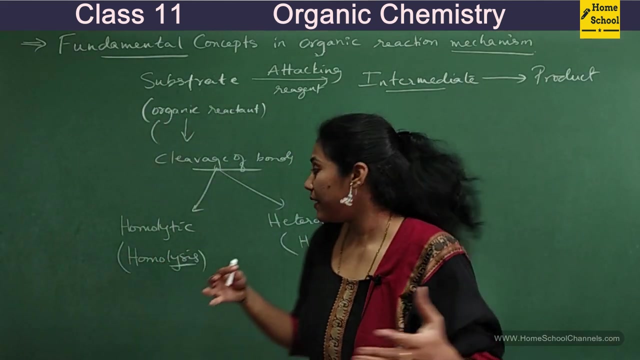 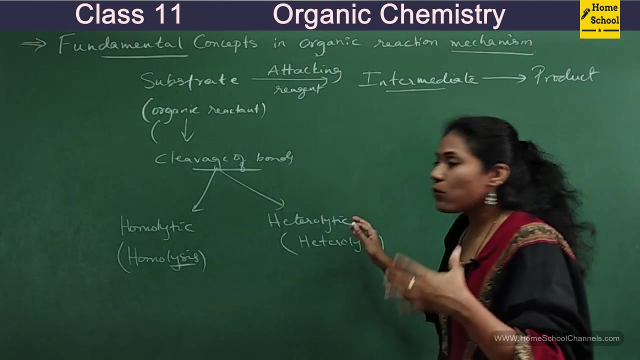 cleavage is also called with the name homolysis and heterolytic cleavage is also called with the name heterolysis. so we know the meaning of the word. lysis right. lysis itself means breaking right. so homo in the sense what equal? homo is always equal and hetero is what different. okay, so let 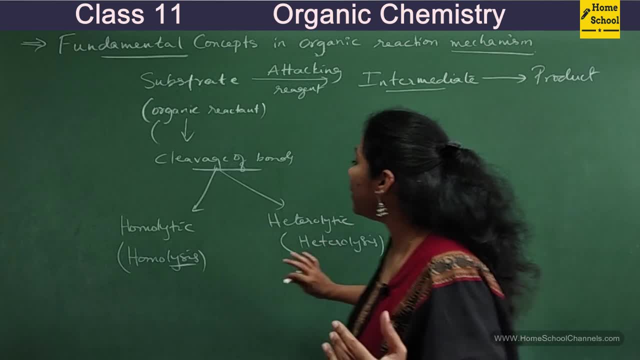 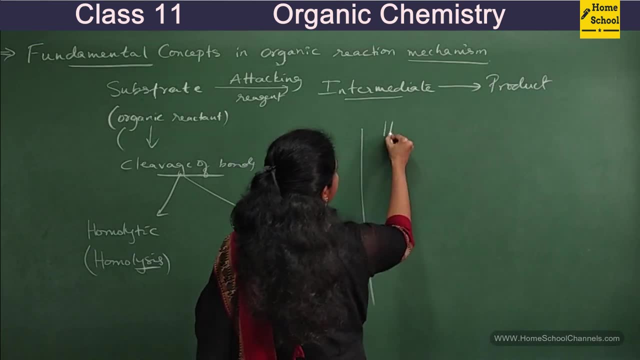 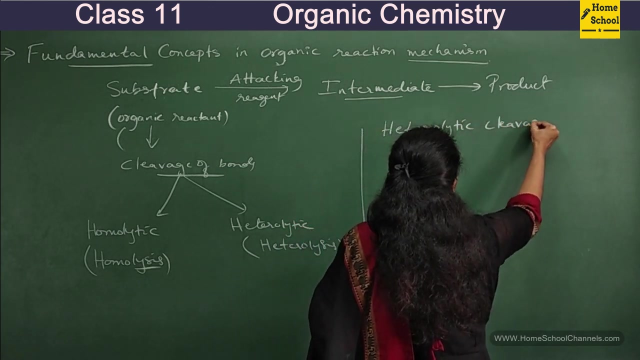 us understand what actives are called homolytic cleavage and heterolytic cleavage is also called by homolytic cleavage and heterolytic cleavage. okay, fine, first and foremost, let us understand everything about heterolytic cleavage. heterolytic cleavage: right, suppose you have an organic. 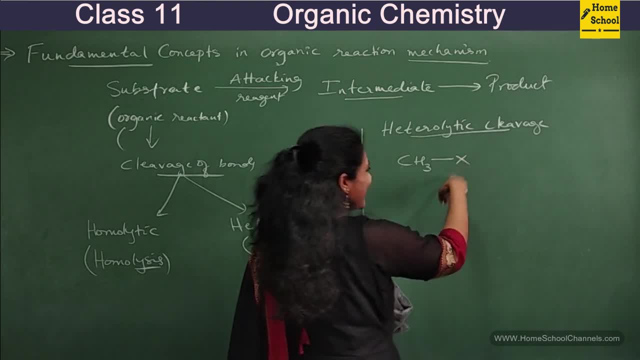 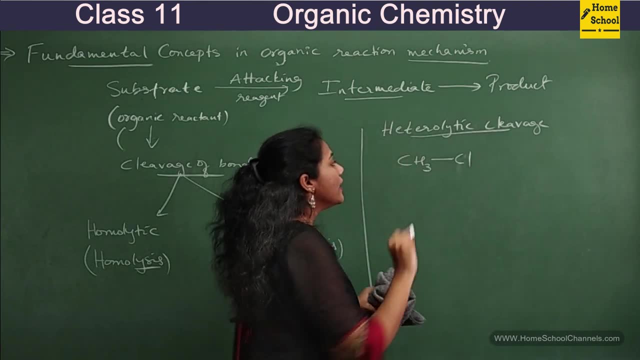 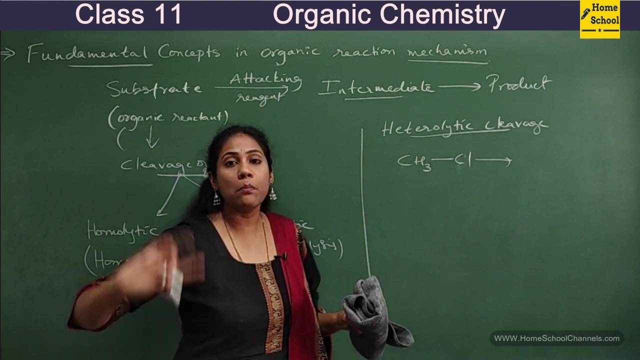 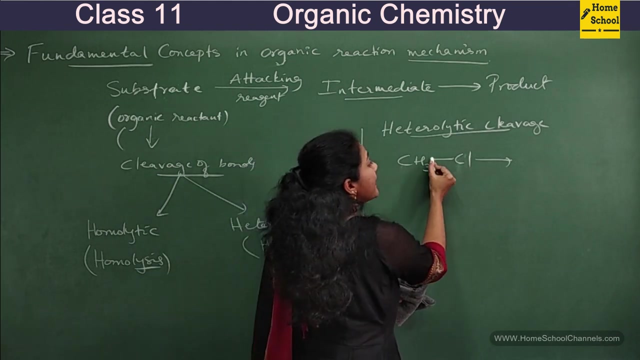 substrate: ch3 x. x can be any halogen. okay, let me take a specific halogen here: ch3 cl right. say: whenever there is an attacking reagent for this substrate, say this is the main organic molecule that is undergoing a reaction. so whenever i supply an attacking reagent, what would happen? this bond, 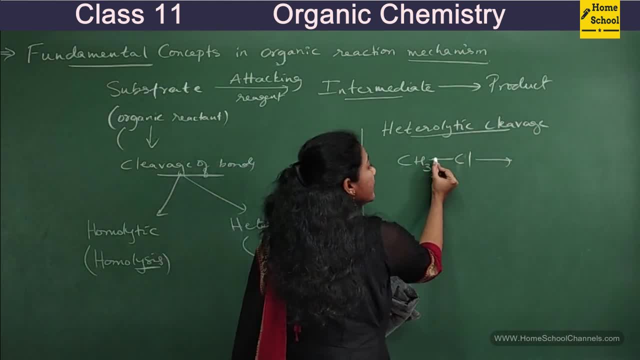 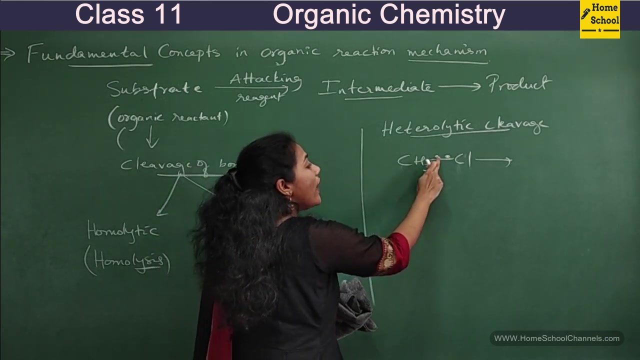 is going to get broken up and we all know this is a covalent bond and this is a single covalent bond. bond itself means that there are two electrons in a bond, isn't it fine? in these two electrons, we all very well know that one electron belongs to ch3 group, the other electron belongs to cl atom. 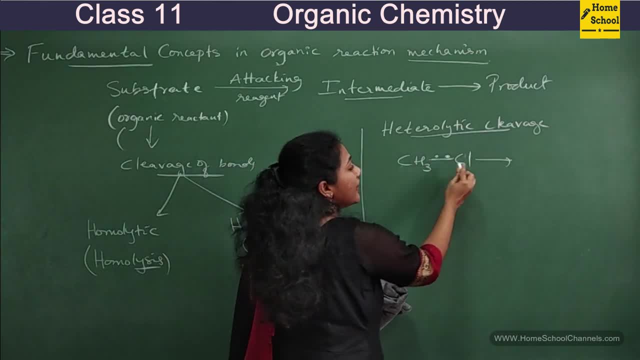 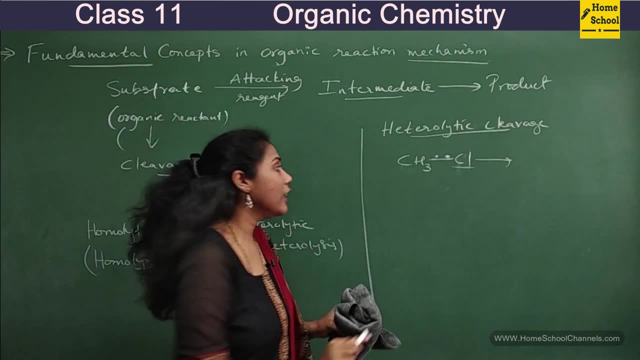 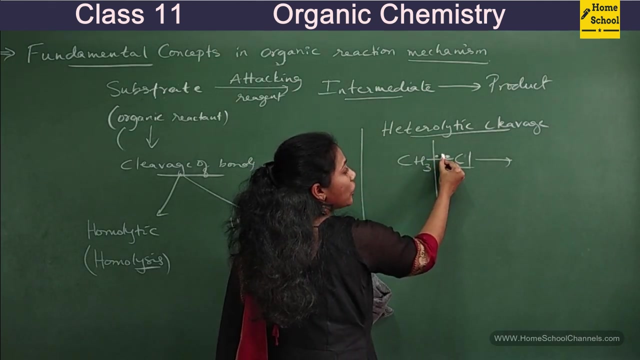 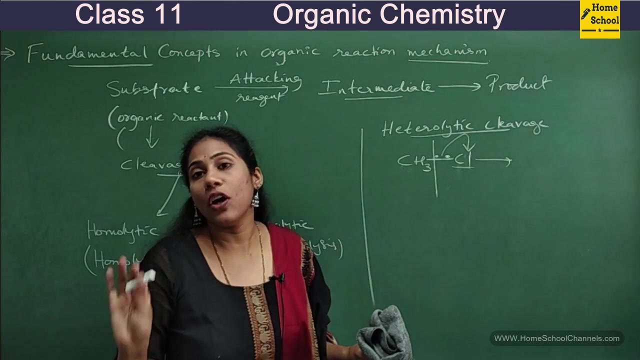 okay. and here you can observe one thing: cl atom is more electronegative compared to carbon of ch3, right, so here bond breaks in a such a way that both the shared pair of electrons move towards cl. okay so. So such a cleavage of an organic bond, I mean a covalent bond, is called as heterolytic cleavage. 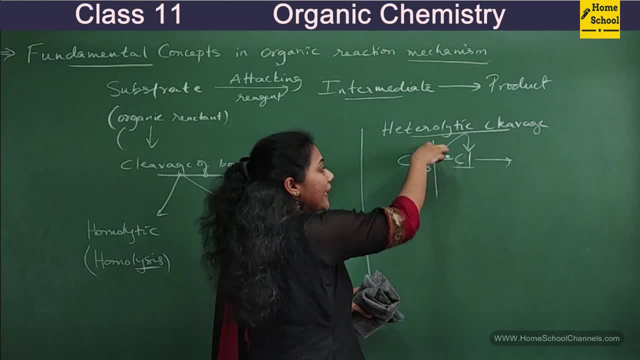 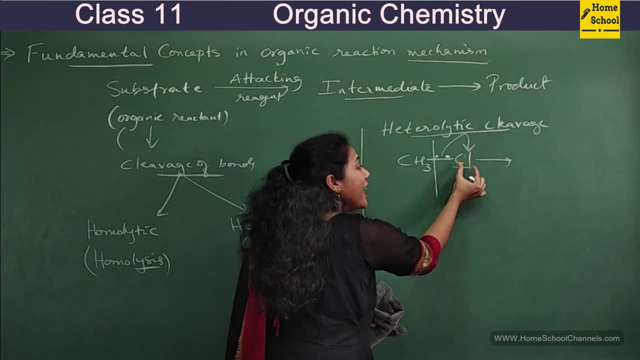 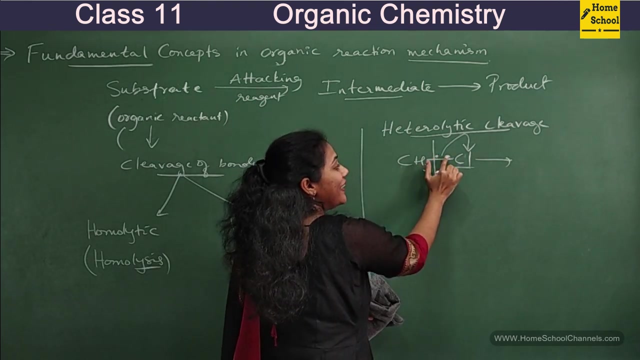 So how is the bond getting broken up here? It breaks in a such a way that both shared pair of electrons will move towards one of the atom. So here, both electrons, electron from methyl group and electron from Cl- that made a bond right. So both electrons are actually moving towards Cl. 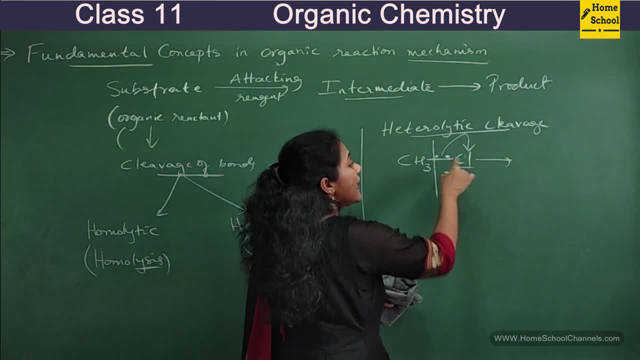 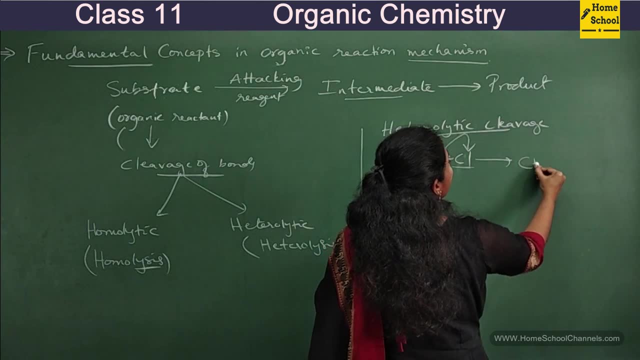 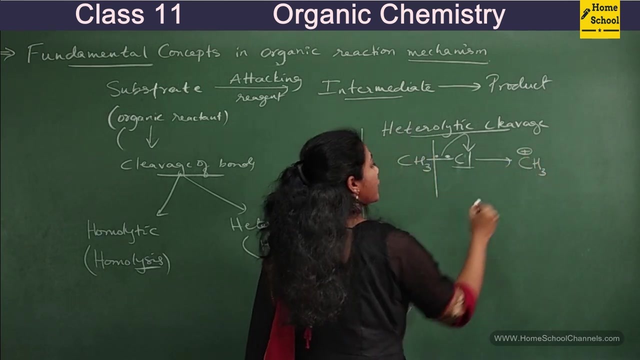 Why are they moving towards Cl? Because Cl is more electronegative atom clear. Okay, so now what do you get? Bond will break and both electrons are moving there, So you will have a positive charge on CH3 and our Cl will get a negative charge. 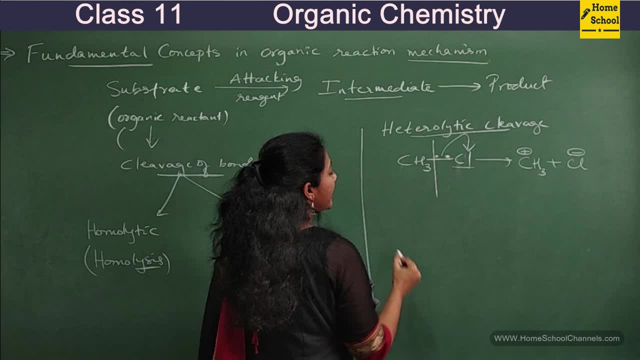 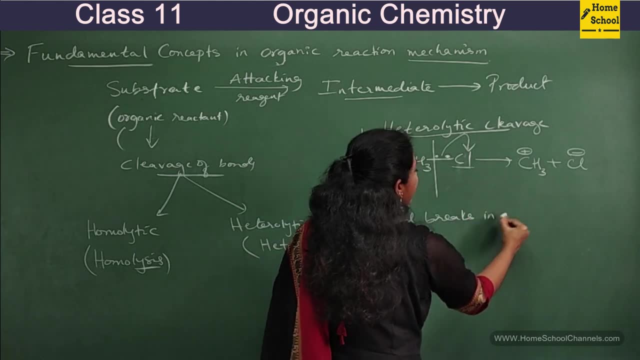 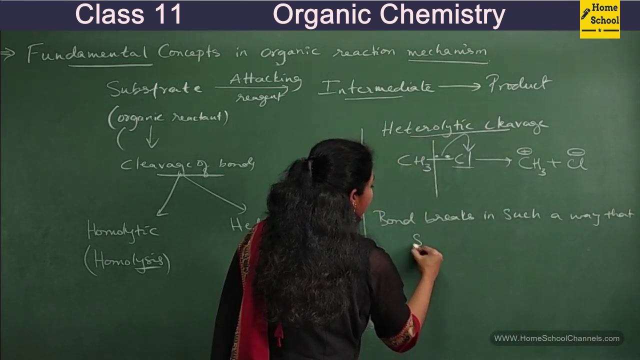 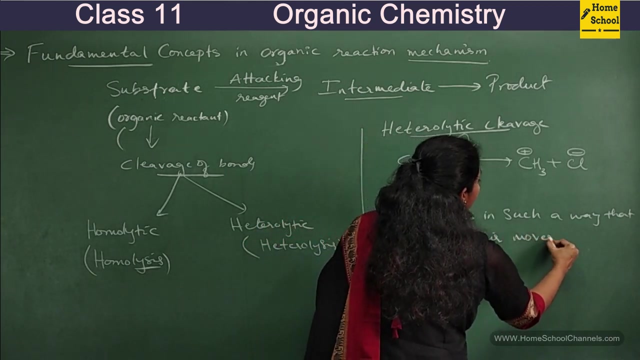 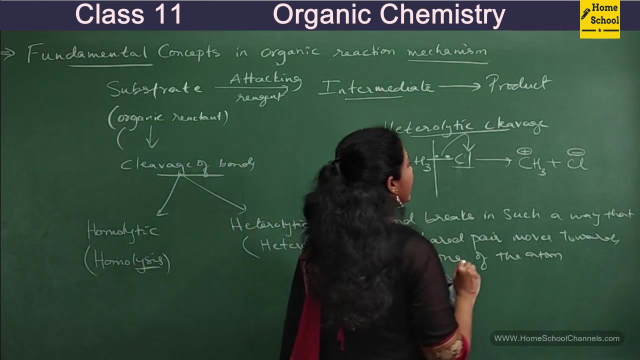 Okay, so what I can write as a definition for heterolytic cleavage: Bond breaks in such a way, that bond breaks in such a way that, such a way that shared pair of electrons, shared pair, moves towards, towards one of the atom. Okay so this is the definition of heterolytic cleavage. and here you observe one thing after: 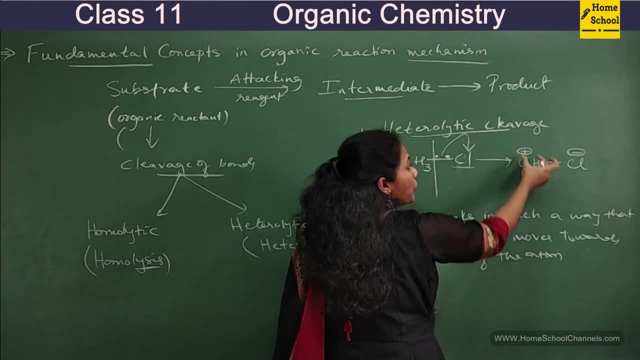 heterolytic cleavage, one atom or a group will have a positive charge. the other atom will have a negative charge. Okay, see, if the positively charged group is a carbon group, say CH3, it's a carbon group, right? So this positively charged carbon group will have a positive charge. So this positively charged carbon group will have a negative charge. 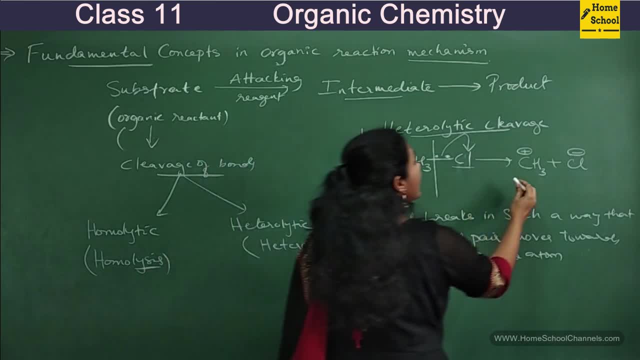 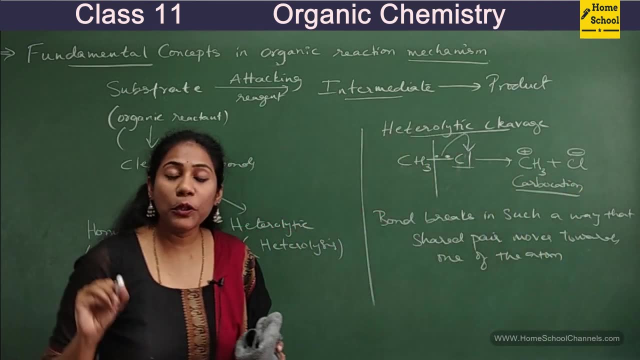 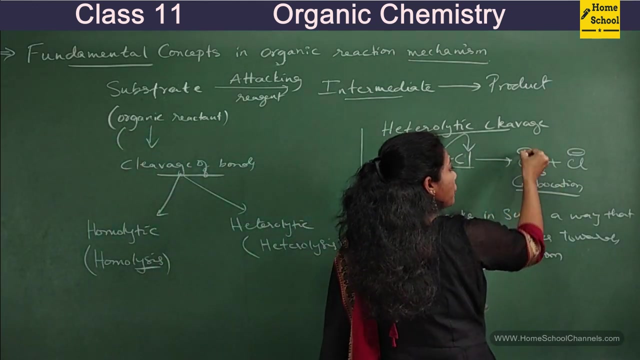 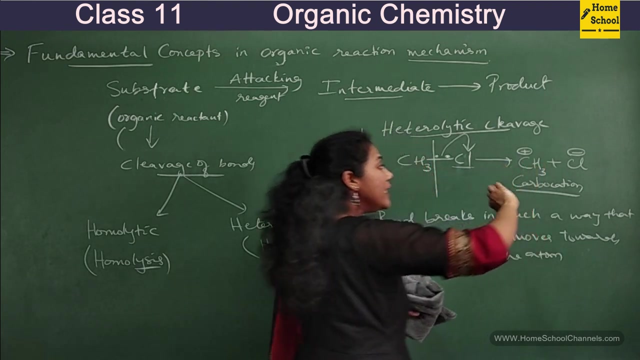 Carbon groups, carbon species, are called with the name Carbocation. So this is called with a special name Carbocation. So why we are calling this as Carbocation? Because it is a carbon species and this positive charge is there on carbon. okay, So if you look at CH3 plus, you will see there are only 6 electrons around carbon. 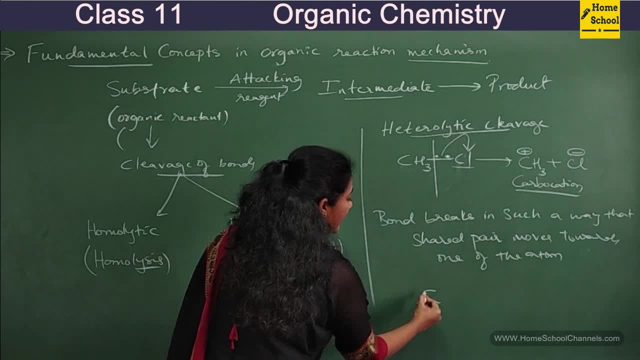 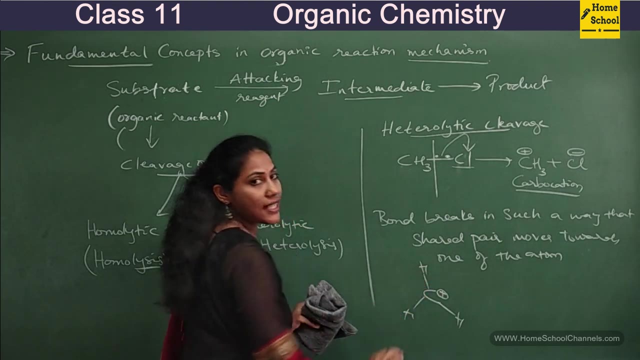 Right. So if I put CH3 structure to it elaborately, how do i put it? so h 3, h is positive charge. why do i put positive charge? you see how many electrons are there around carbon. one bond means two electrons, two, two, two, only six electrons. 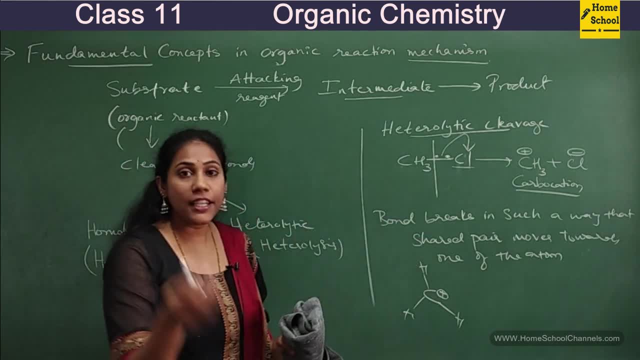 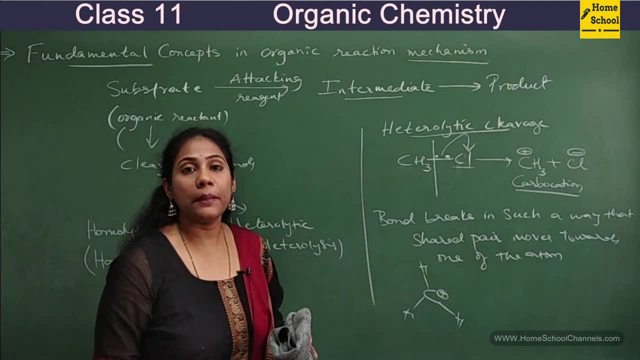 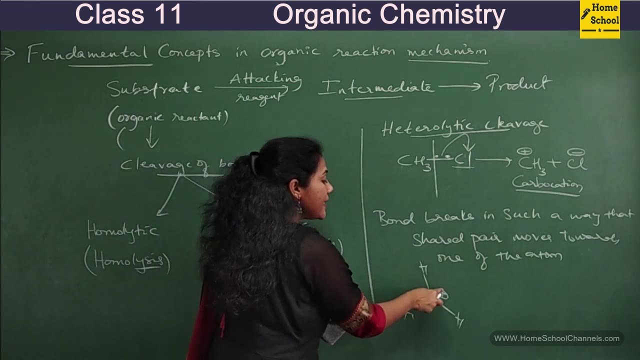 are there, okay, so it is there in a deficiency of two electrons. it want two more electrons for its stability. that is why, plus charge we have put on carbon, it has lost its electron. to whom to cl right? so carbon species with positive charge is called as carbocation. so carbocation is one of 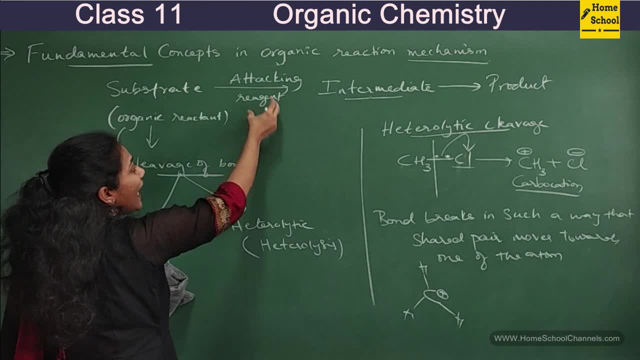 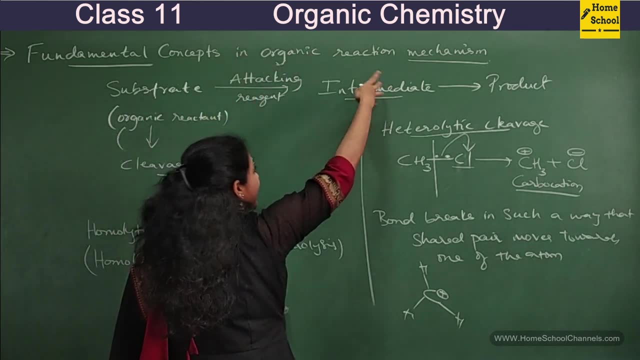 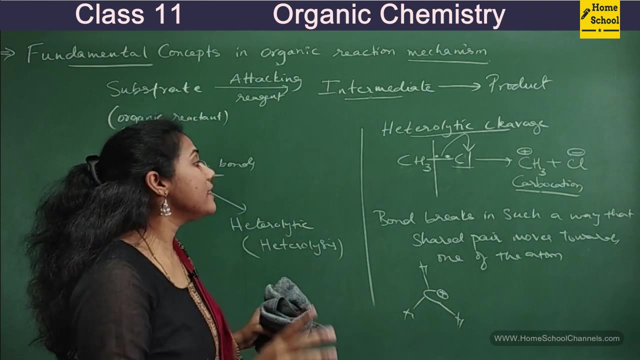 the intermediate. what did i tell you? whenever you add attacking reagent to a substrate, some bonds who some bonds would break down and you will end up in getting intermediate. so here, carbocation is one of the intermediate. so now let us learn about the other way of. 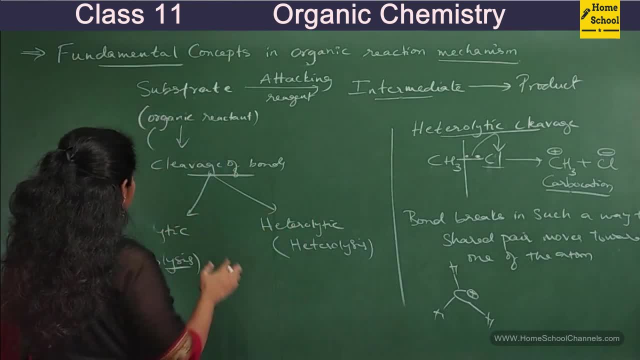 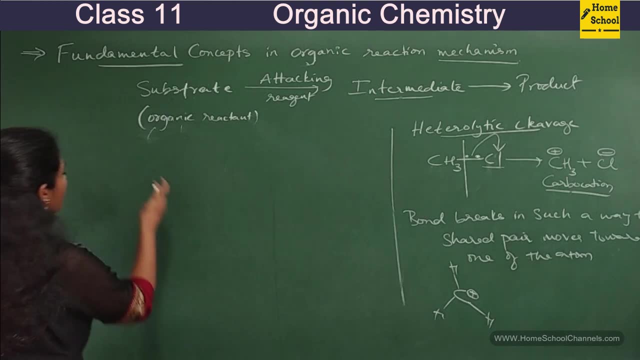 heterology cleavage, right, fine. so observe this type of heterolytic cleavage, suppose. suppose, if we have a molecule, ch3 say, some electropositive element is there. okay, cu is there. so we all know cu is more electropositive than ch3. so here, in presence of some attacking reagent, if this bond have to be, 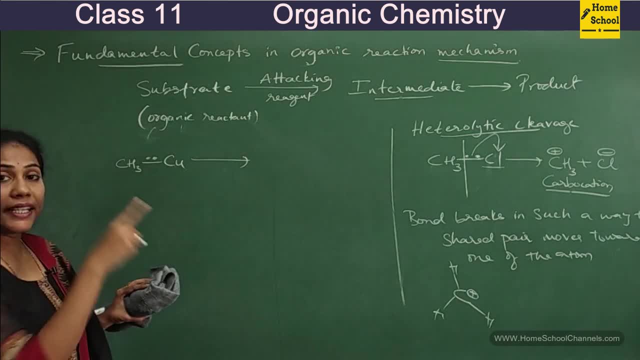 here we can apply heterolytic cleavage, okay. so what happens here? since carbon is more electronegative than copper, both bonded pair of electrons or shade pair of electrons will move towards ch3 group. so what are the ions you will get? you will get ch3 with minus charge and cu plus. 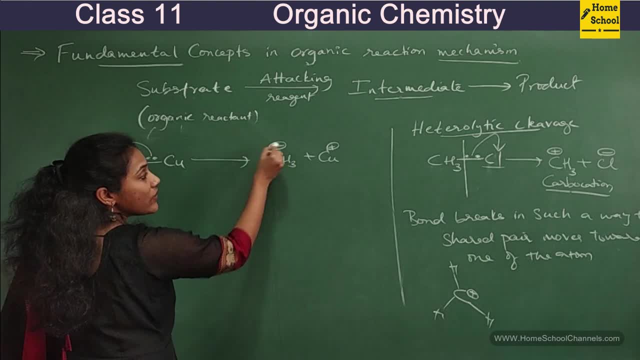 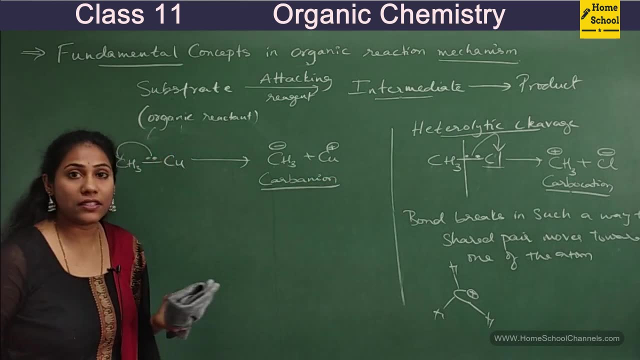 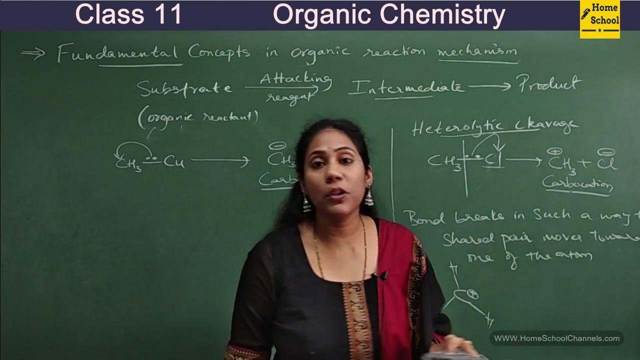 right, and carbon species with a negative charge is called with ch3, so here we can apply heterolytic cleavage to the name carbanion. they are called as carbanions. okay, so you must understand the two situations, like in which situation you are getting carbocation and in which situation you are getting 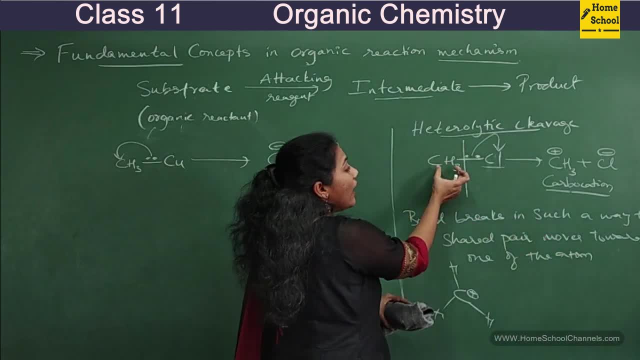 carbanion. okay, so whenever carbon groups- i mean organic groups- are bonded with the most electronegative element, both bonded electrons will shift on to electronegative element and you will end up in the situation where you are getting carbon ion and in which situation you are getting 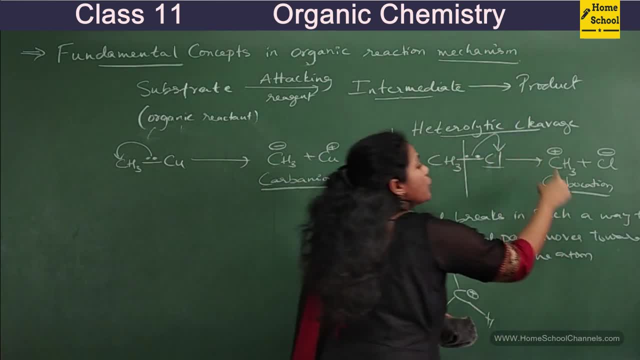 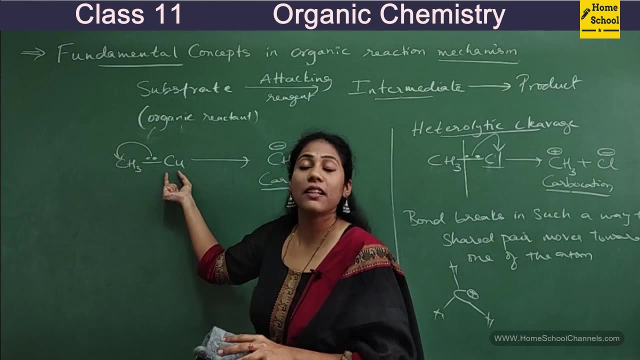 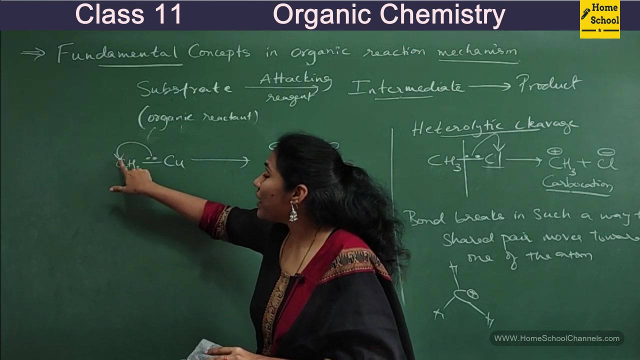 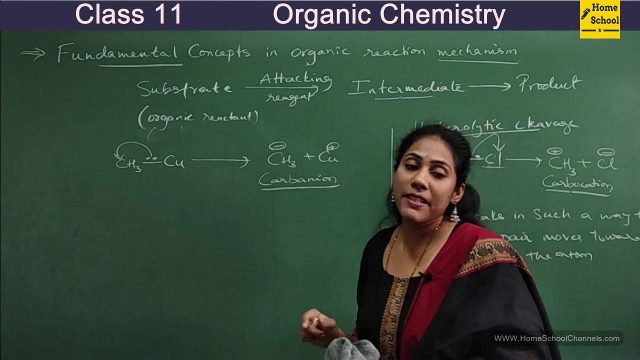 getting positively charged carbon species, which we call it as carbocation. But when organic group has a bonding with some electropositive element- electropositive than carbon- then shade pair of electrons will move towards CH3, you will end up in getting negatively charged carbon species. 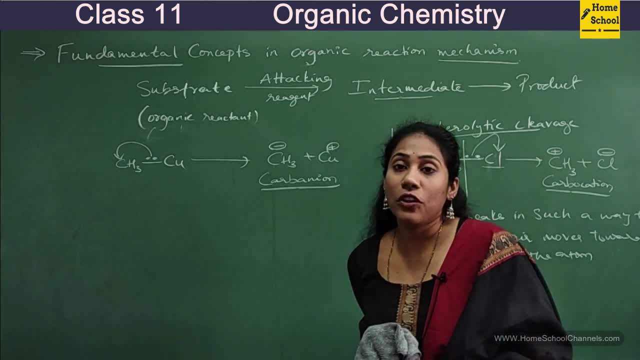 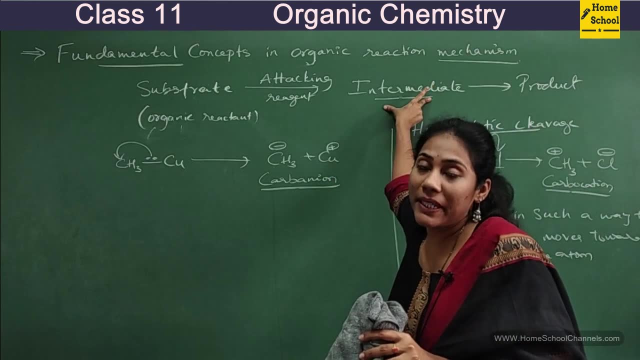 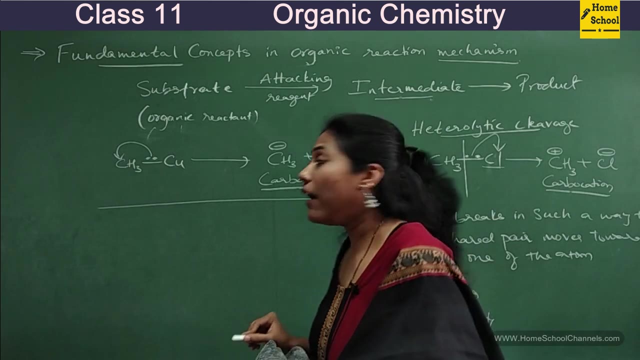 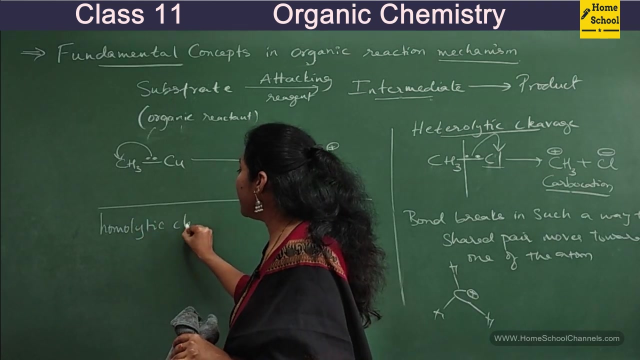 which we call as carbonyl ions. Okay, so here both carbocations and carbonyl ions can be called as intermediates. Okay, fine, So that is all about heterolytic cleavage. So now we will learn. what do we mean by homolytic cleavage? So this is very simple. In heterolytic, we observe: 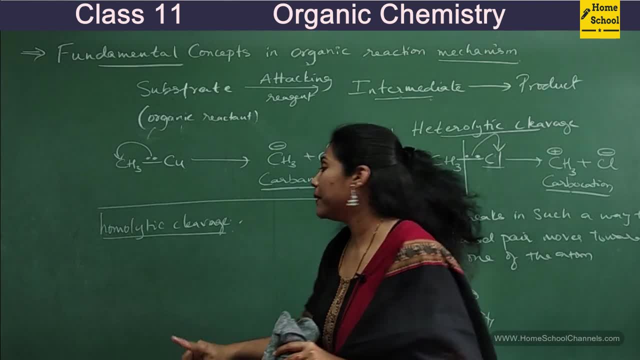 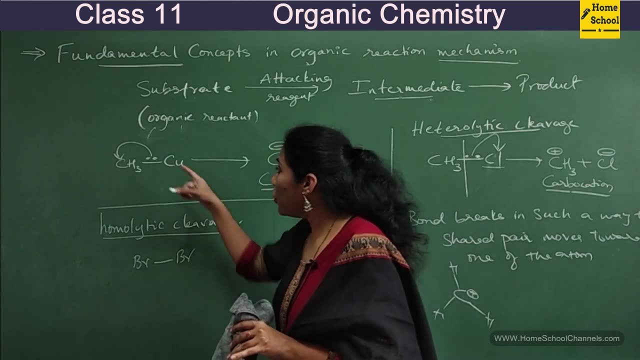 both carbocations and carbonyl ions. So this is very simple. In heterolytic we observe both carbocations and carbonyl ions, both electrons moving towards one of the atom. But here you observe Br bond Br. You will observe. 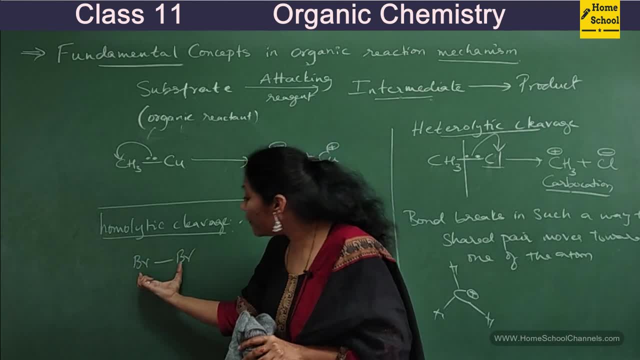 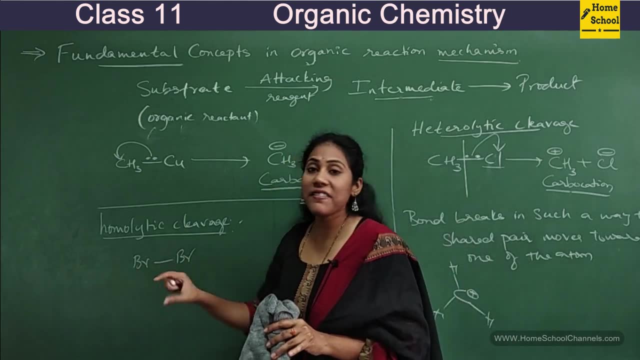 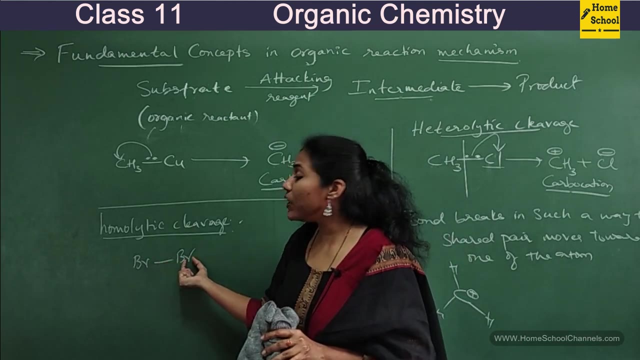 homolytic cleavage when there is equal electronegativity difference between the atoms or group. Okay, see Br, Br. both have same electronegativity value, So here bond will not go. I mean, both electrons will not go towards one of the atom. They are equally distributed. 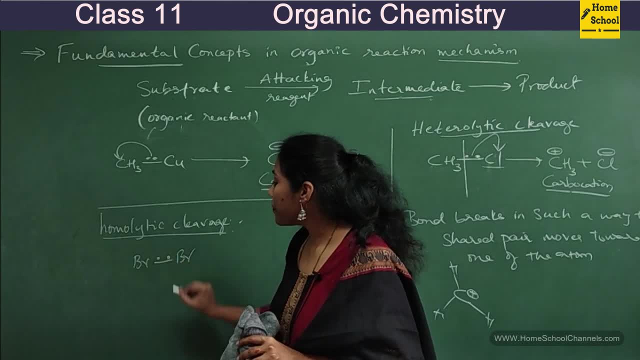 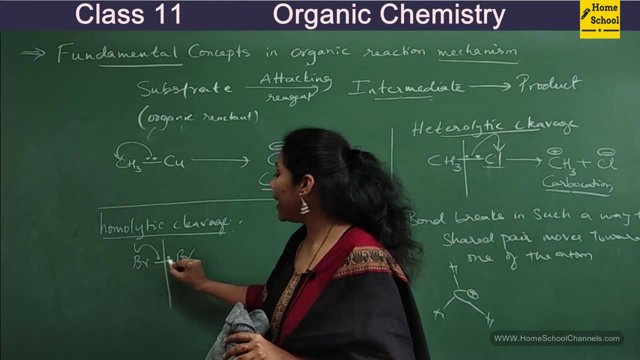 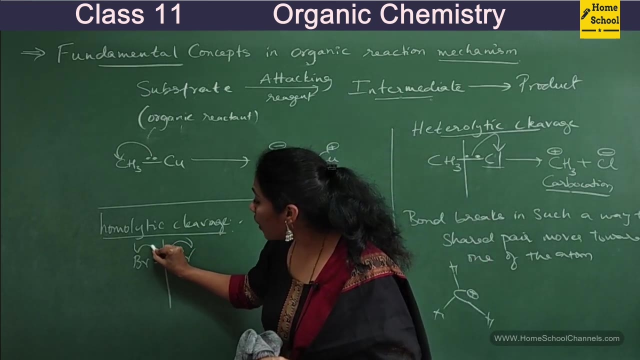 Okay, observe here. So these are the two electrons of a bond. Bond will exactly break in such a way that one electron moves to one atom, the other electron moves to another atom. Single electron transfer is always indicated by this type of arrow mark. You know if a bond is moving that. 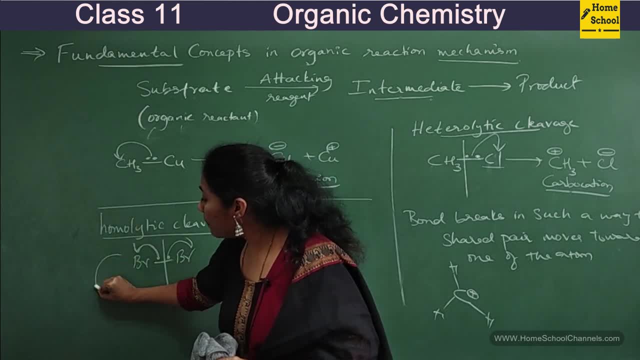 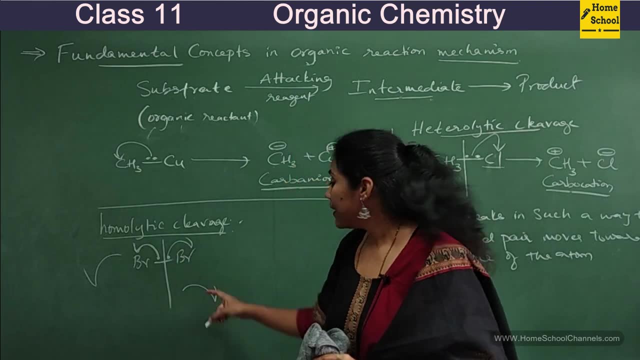 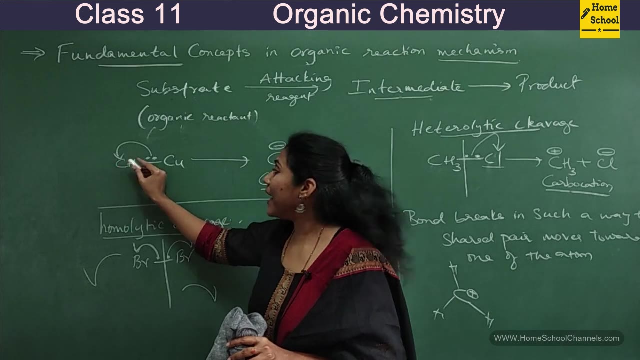 side. I mean if an electron is moving that side, you will put the arrow mark like that. If an electron is moving this side, you will use the arrow mark like this: This is single headed arrow mark. If both electron movement, if two electrons are moving towards one of the atom, then double headed. 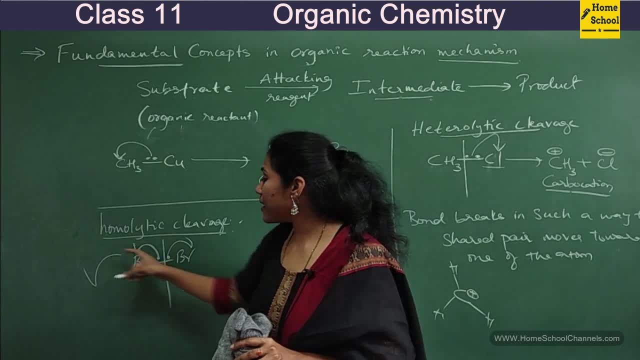 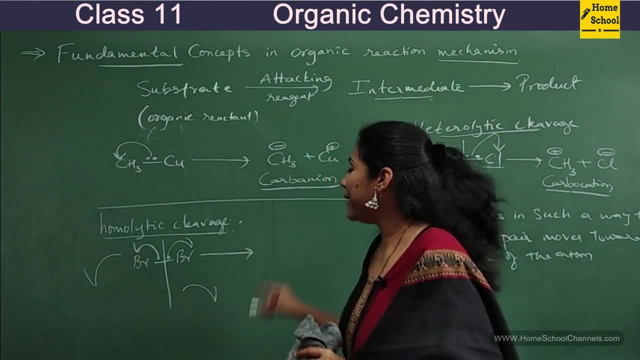 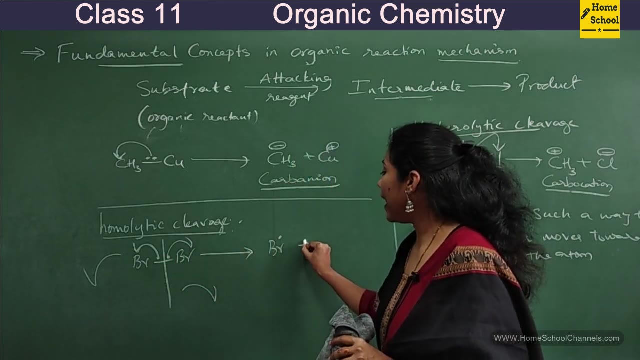 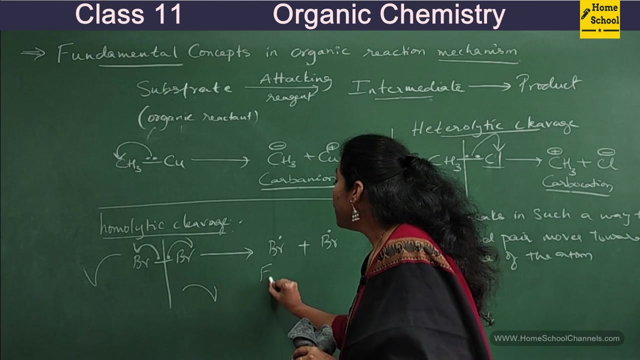 arrow mark we will use. Okay, so these arrow marks are used to show single electron transfer. So what are the intermediates? I mean, what are the species you will get? So one Br has one electron, the other Br has the other electron. So such species are called with the name free radicals. 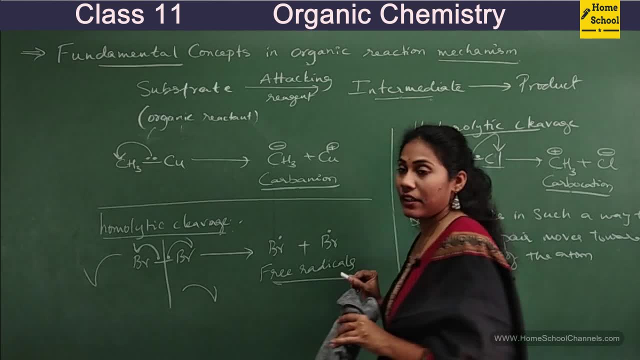 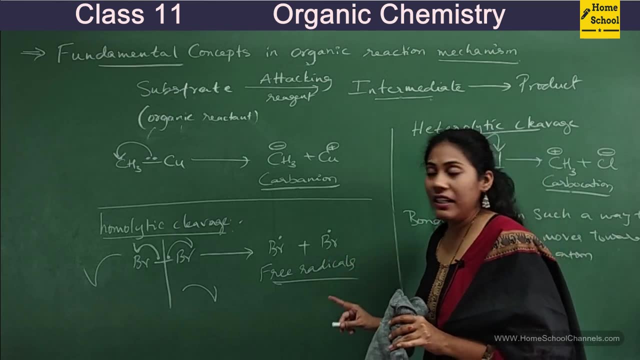 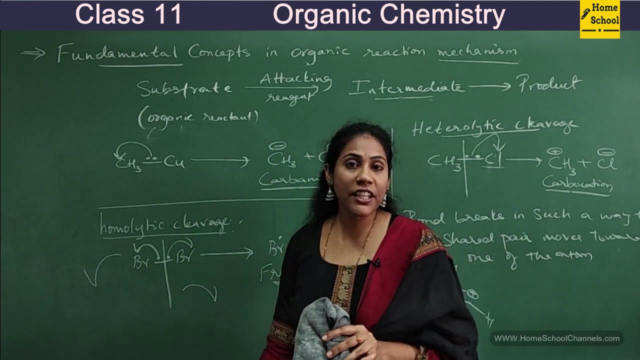 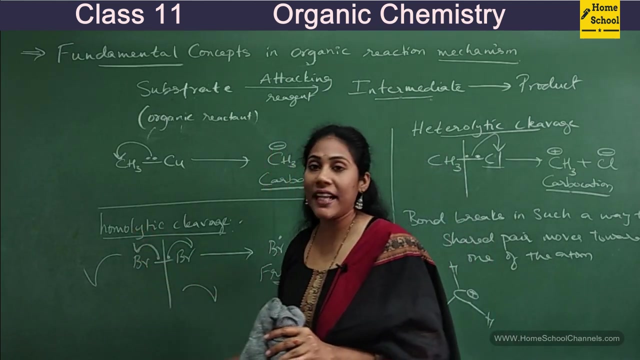 Free radicals very, very important. So these are the third type of intermediate that you can get. So when do we get free radicals? When a bond undergoes homolytic cleavage. So what is homolytic cleavage? Cleavage of bond in such a way that one electron of the shared pair goes to one atom. 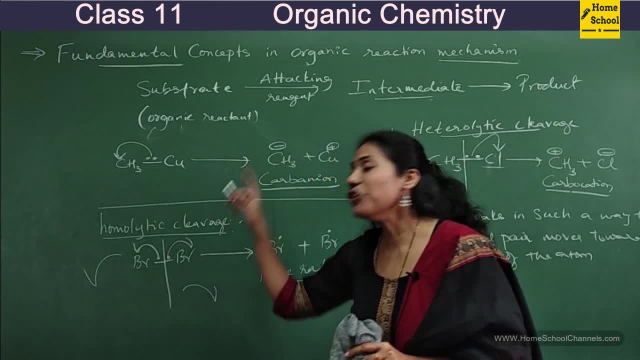 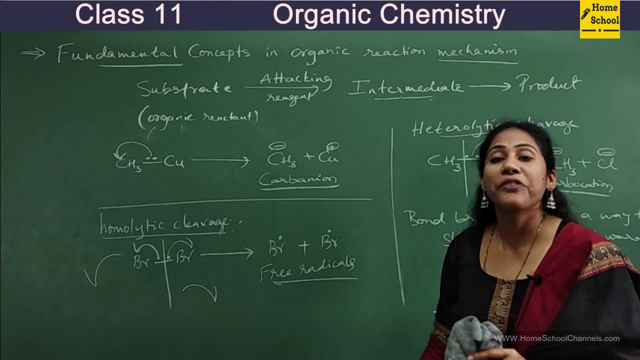 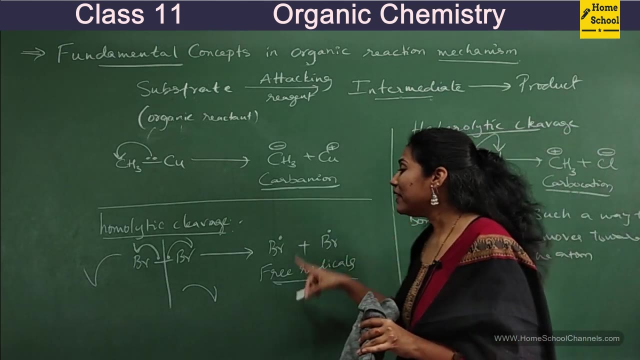 the other electron of the bonded pair goes to another atom. So single electron containing species you will get, and we call them as free radicals. So hope you understood the difference between carbocation and free radicals. So think carbocation, carbocation, carbocation, carbocation and free radicals, right? 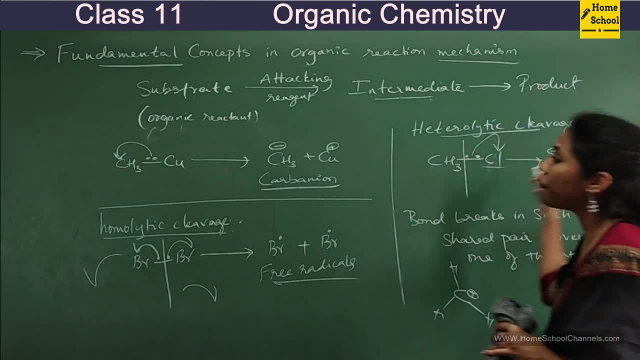 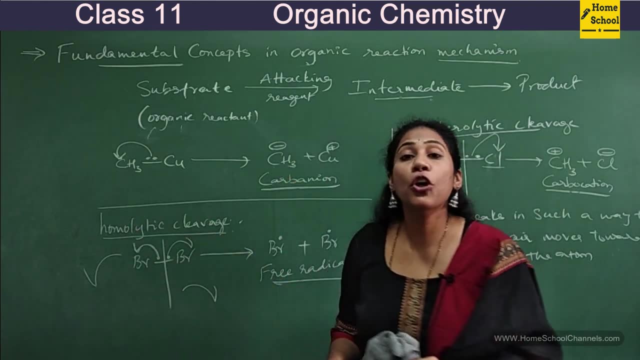 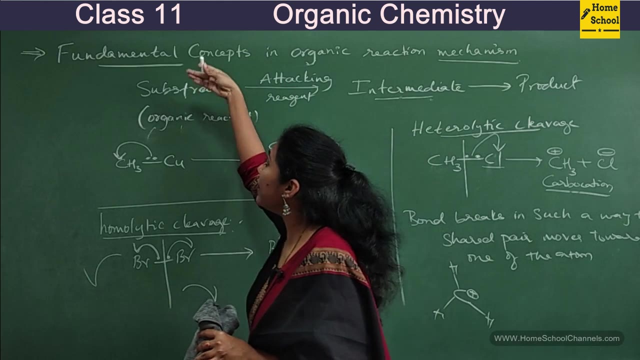 Carbocation. and carbocation are formed by heterolytic cleavage. Free radicals are formed due to homolytic cleavage. Okay, so these are the two types of cleavages that you can observe in a substrate when you add an attacking reagent. 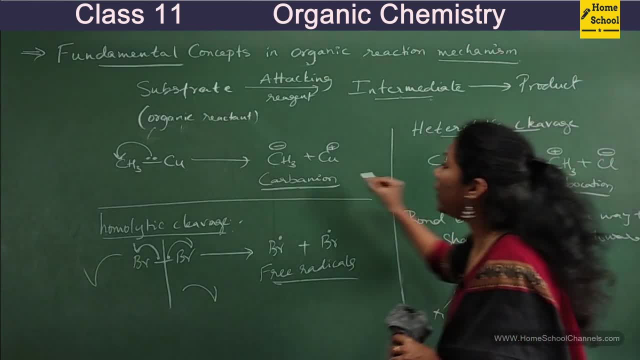 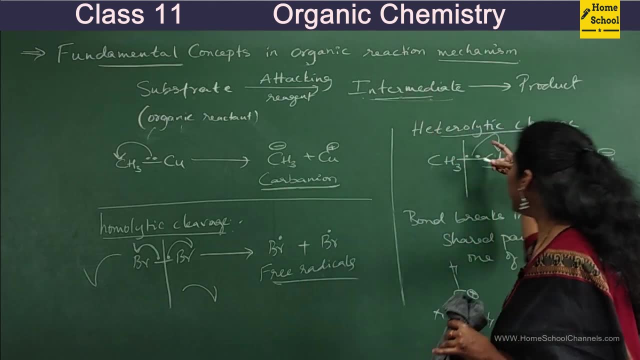 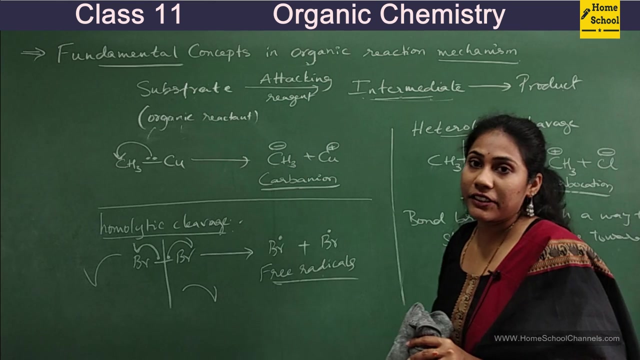 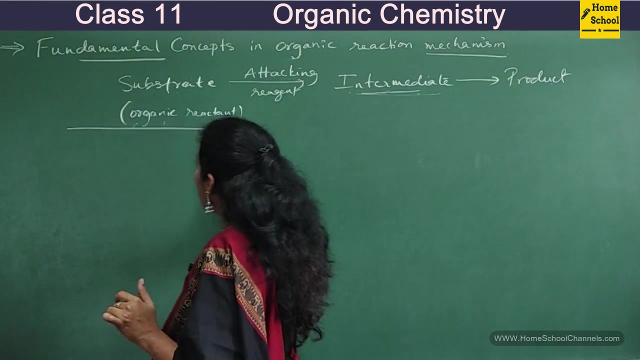 So now I told you that carbocation, carbocation, free radicals are called as intermediates. okay, now these guys, when they undergo certain change or when they react with some other substance, you will end up in getting product. okay, now, let us understand more things about these free radicals. so, guys, now let us learn about more things on. 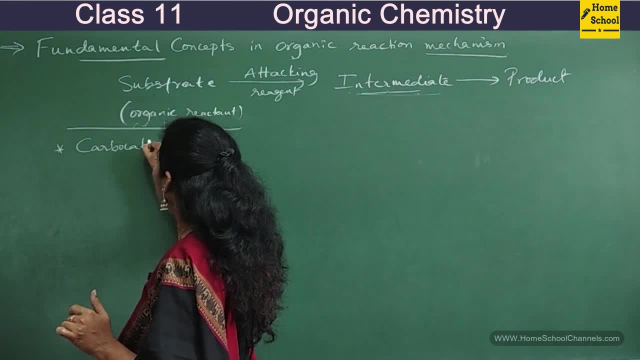 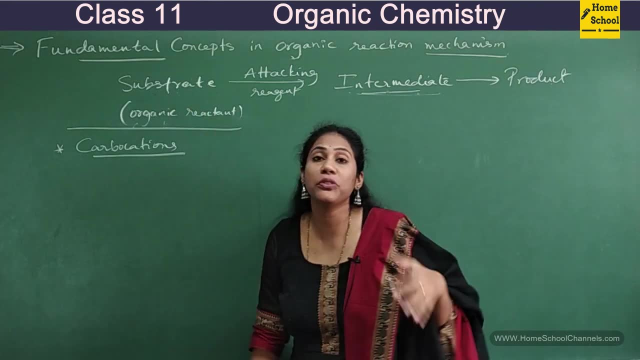 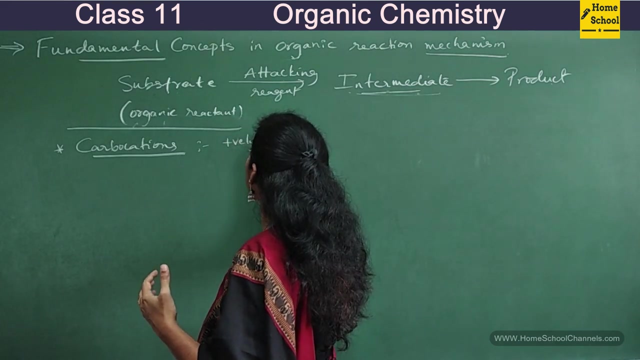 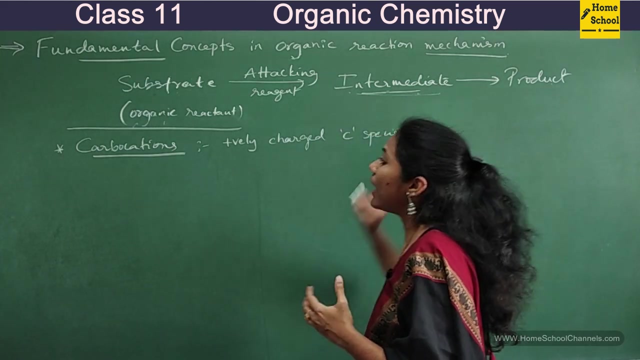 carbocations. carbocations, so these are the very, very first major type of intermediates that can be formed during organic reactions. okay, fine. so what are carbocations? positively charged carbon species? positively charged carbon species are called as carbocations. you know how and in which situations they are getting formed, right? 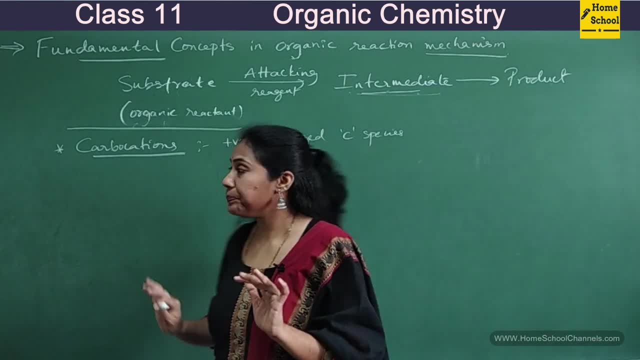 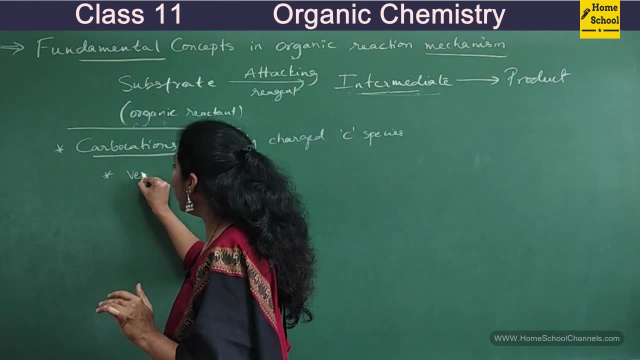 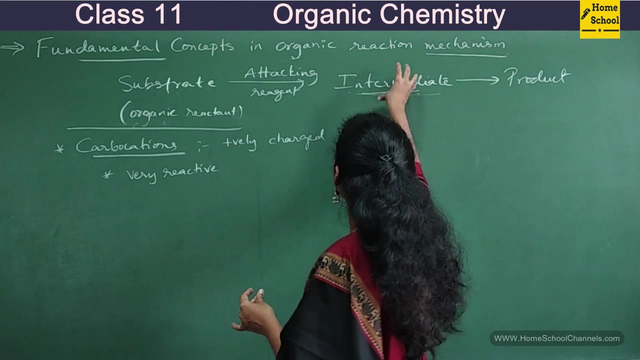 so they are formed during heterolytic bond cleavage. okay, so now if i have to talk about the reactivity, they are very, very reactive. you know they are not stable in a nature, right? so the moment they form, they should react with someone else to give a product, or they should 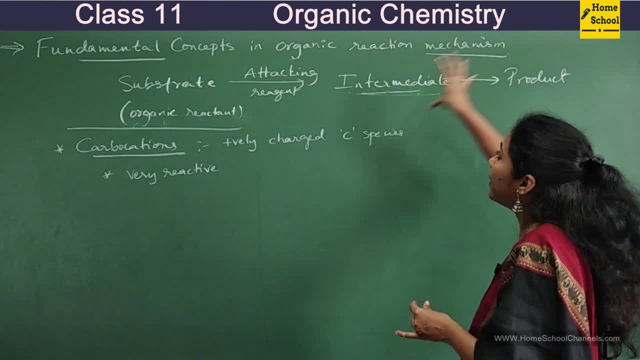 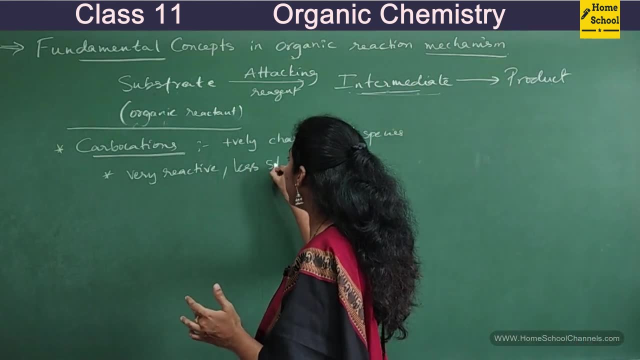 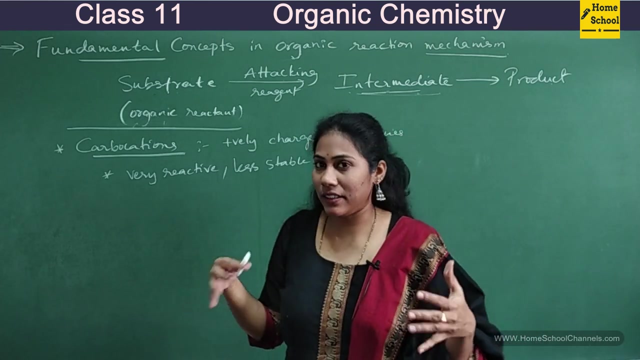 undergo some change in a structure to give a product right. so they are very much reactive and they are very, very you less stable. okay, less stable in the sense they cannot stay for a longer time during a reaction. the moment they form, they quickly die. in a layman language i can use that: the moment they form, they 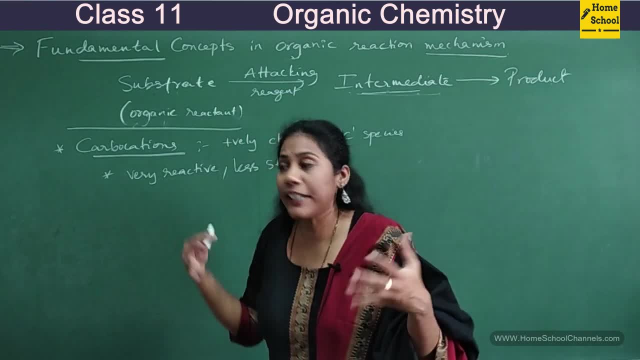 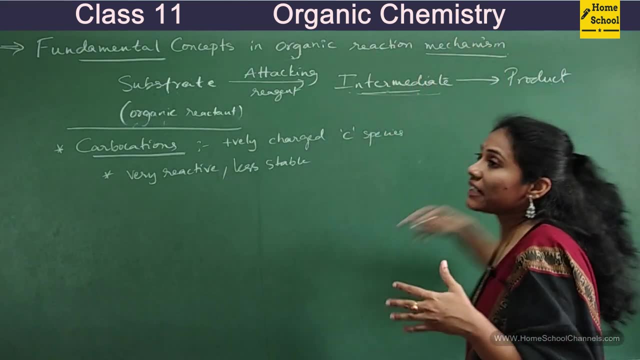 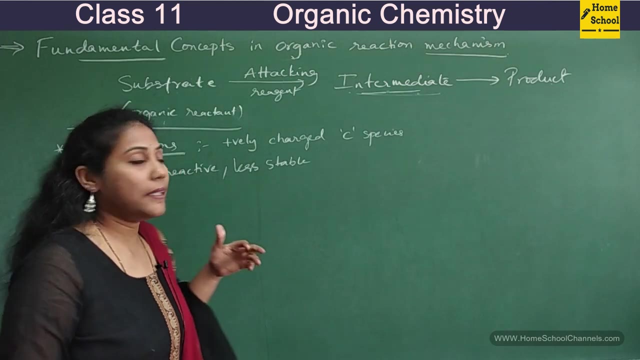 will like to die. i mean to say they eagerly wait for some reactions to happen with them or they eagerly wait for some structural changes in them ultimately end up in giving product okay. so that is the reason we say they are very, very reactive and less stable. and you know what? the carbon atom. 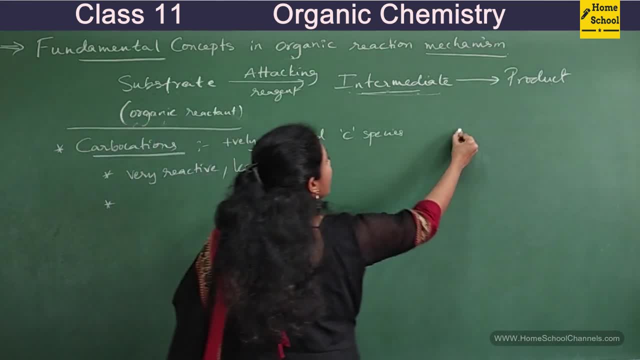 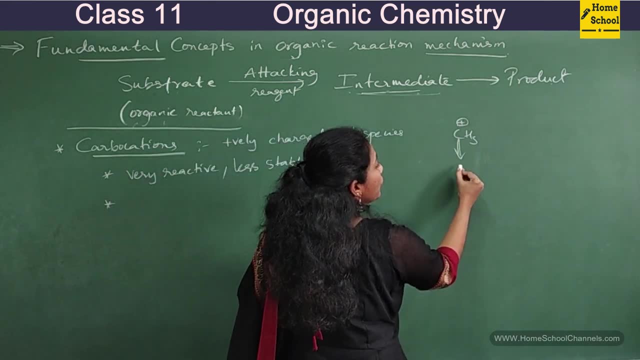 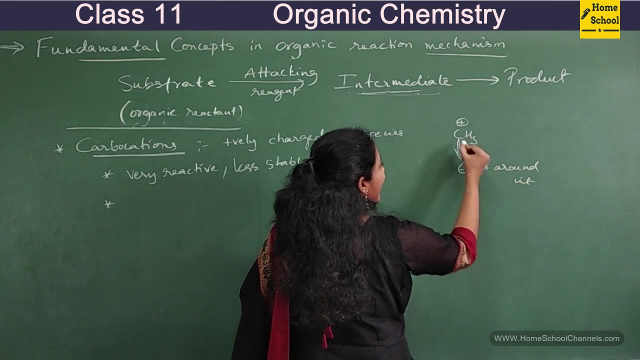 uh in carbocation say, for example. uh ch3 plus is the example for carbocation. i said right. so this particular carbon, if you look at it, has only six electrons around it. only six electrons around it. so i can say they are electron deficient species. so they are. 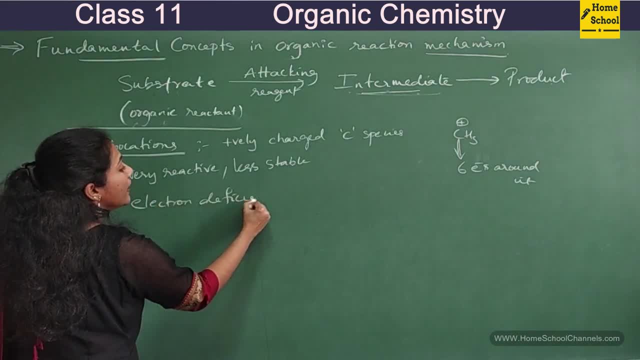 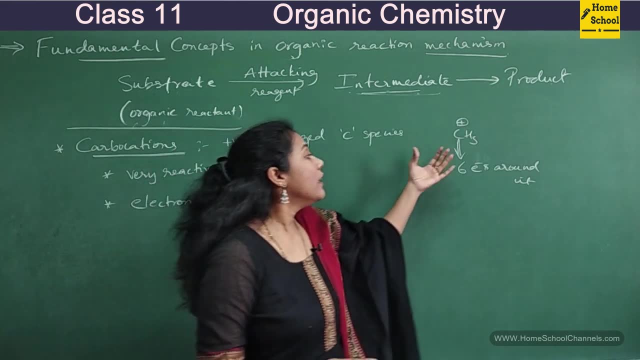 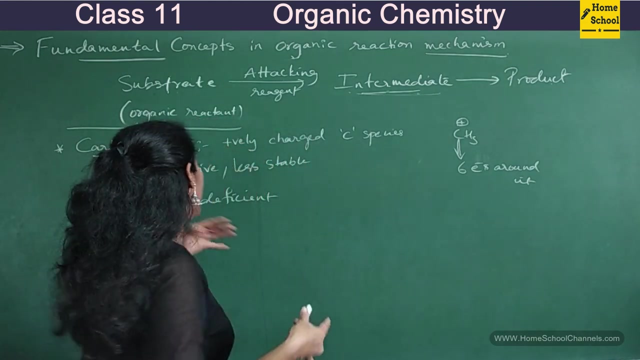 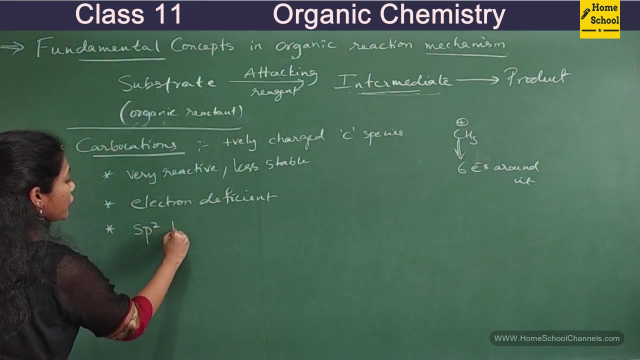 electron deficient. so we all know, if there are eight electrons around any atom, then it is most stable one, right? so, uh, you know, they have only six electrons, so they eagerly wait for the reactions to happen with them. so they are electron deficient also, okay. and they have sp2 hybridization. so carbocations have sp2 hybridization. i mean to say this carbon in carbocation has sp2 hybridization. so if anything has a sp2 hybridization, it will show what type of structure. trigonal planar structure. trigonal planar structure. okay, say how these hydrogen atoms are arranged around that positively charged carbon in a trigonal planar. 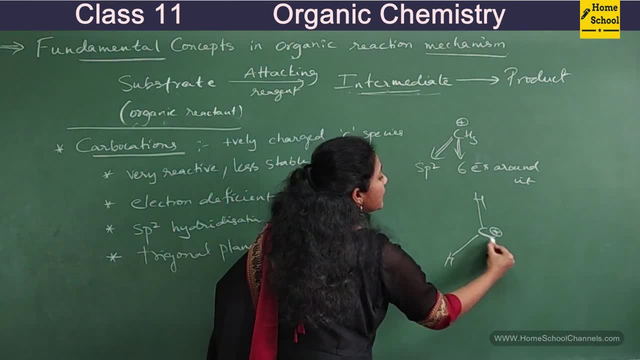 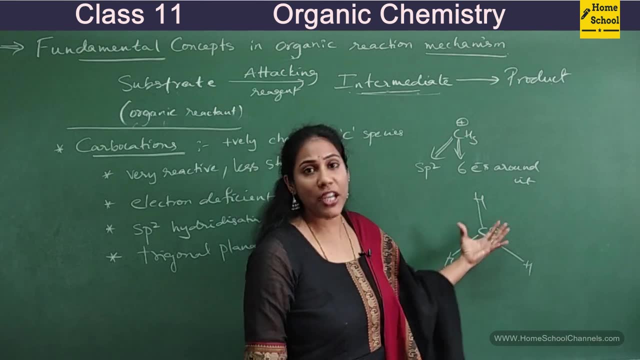 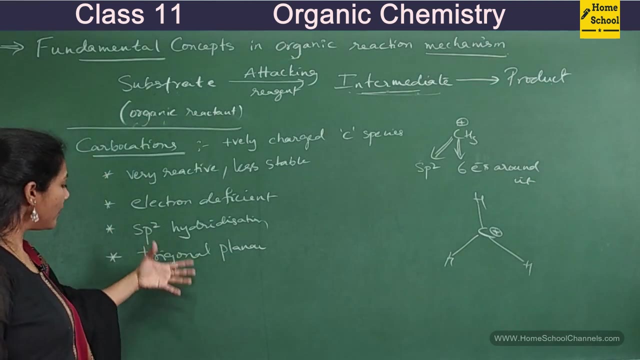 shape. okay. so here one hydrogen. so this is how. uh, the ch3 molecule has a shape, th3 plus uh, ion has a shape. okay. so anything that has sp2 hybridization will always should have a shape- trigonal planar, okay. so these are some basic. 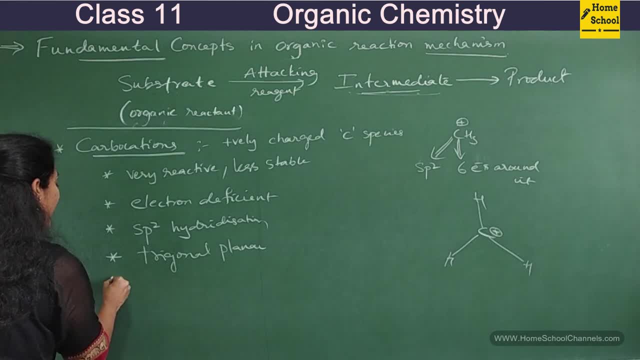 idea on carbocation and you actually have different types of carbocation. can be having different types of carbocation. they can go in different saltский, which is also hayward-decz- calculate the bases of Bachelor option. so that's a very important feature of carbocation. one and athlete is the equipped to block out the Ebond starve carbon units. tutorial and best way to start: Колег好像以. 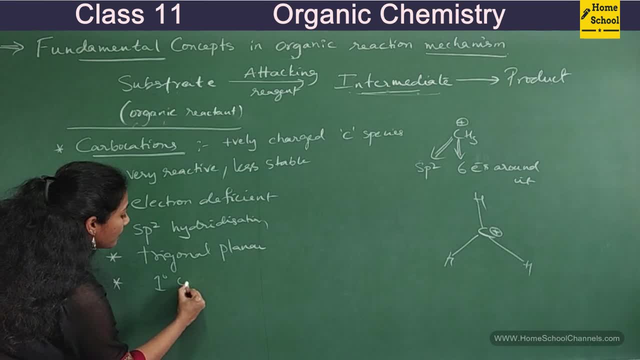 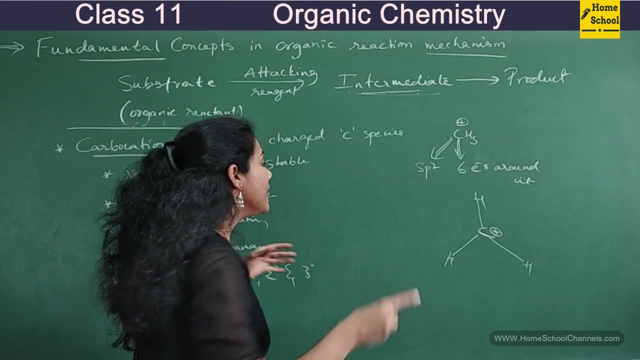 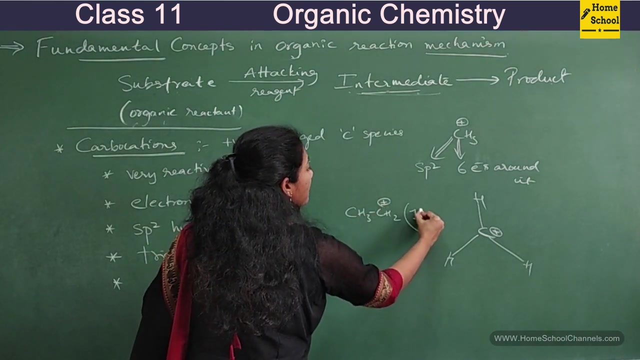 types of carbocation like primary carbocation, primary carbocation, secondary carbocation and tertiary carbocation. So how do I show primary, secondary and tertiary? here Say CH3CH2+. So this is an example for primary carbocation. What do you mean by primary carbon? 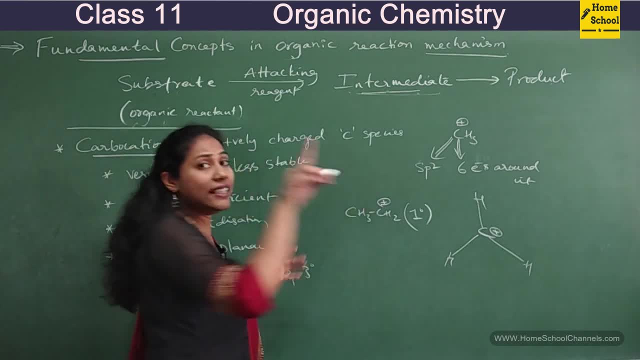 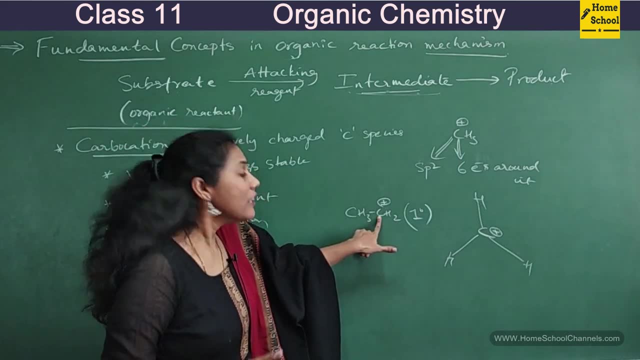 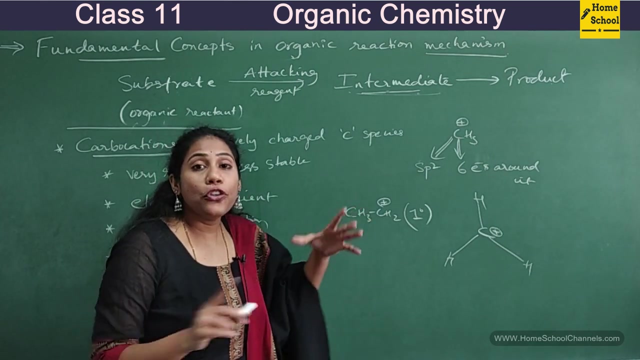 If a carbon has a bond with one other carbon around it, then such a carbon is called as primary carbon. If you look at this carbon with how many carbons it has got in bonding with With only one carbon, that is this side. So looking at the number of CC bonds, you can decide whether a carbon is. 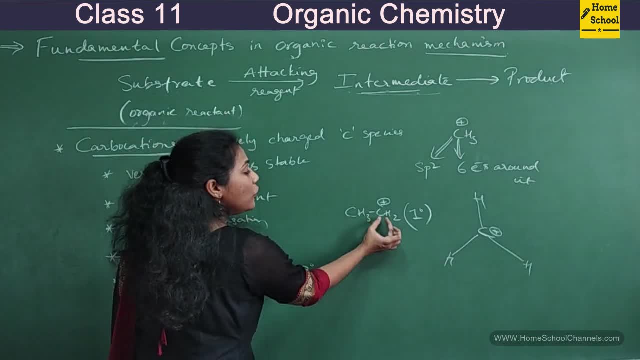 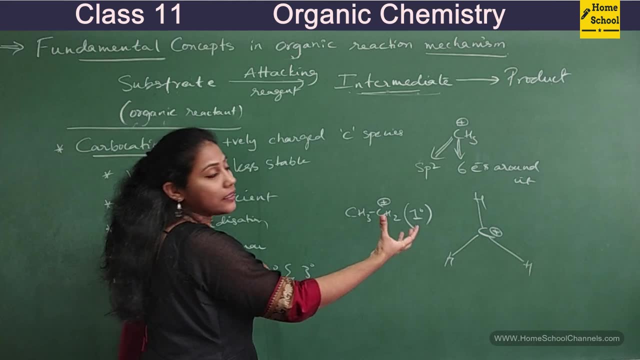 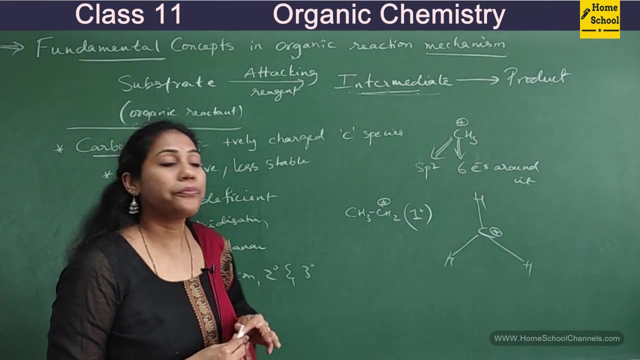 primary, secondary or tertiary. So if you look at a positively charged carbon, this carbon, it has only one bond with other carbon, So there is only one carbon surrounding it. So such a carbon is called primary carbon. So what do you mean by secondary carbon here? 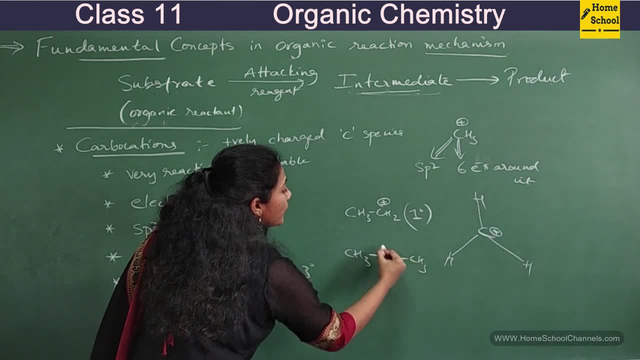 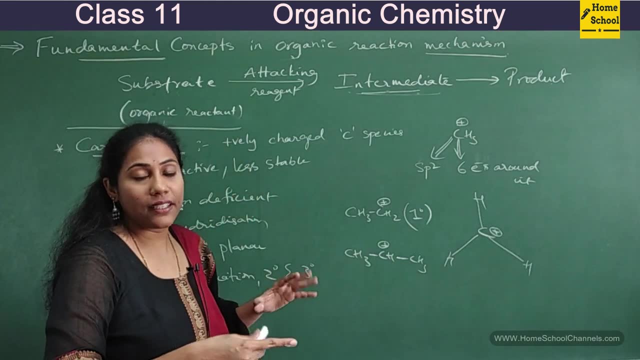 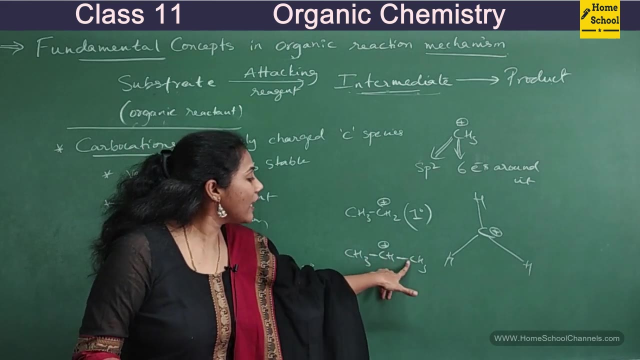 You see this, See, you can observe this carbon getting on. So this carbon around it, how many CC bonds are there? I mean, this carbon has a bonding with how many other carbons? One carbon this side, one carbon the other side. So this carbon has two CC bonds, So there are two. 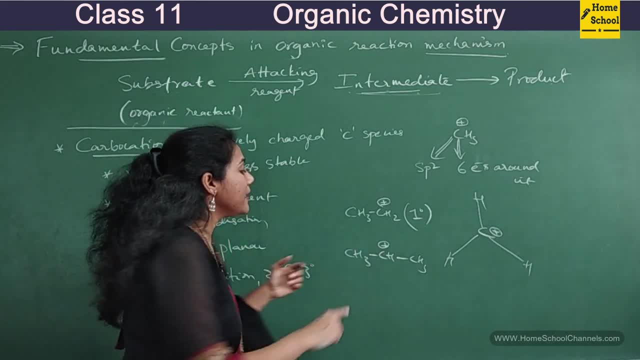 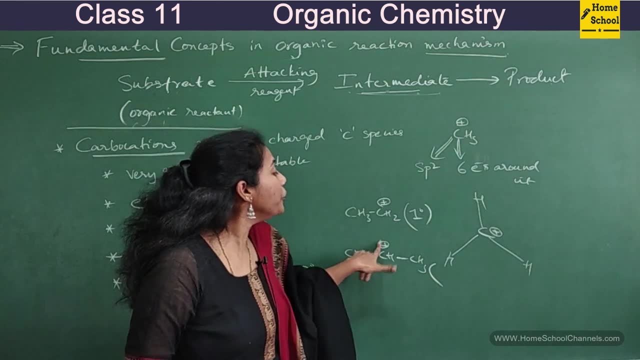 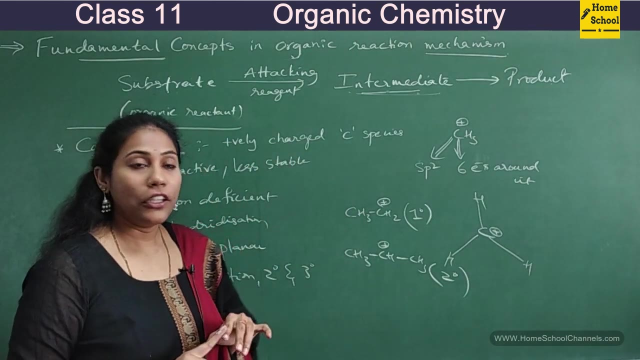 other carbons surrounding this. So such a carbon is called as secondary carbon and such a carbocation On a secondary carbon if you have a positive charge and we call that carbocation as secondary carbocation, Okay. so now look at another structure. 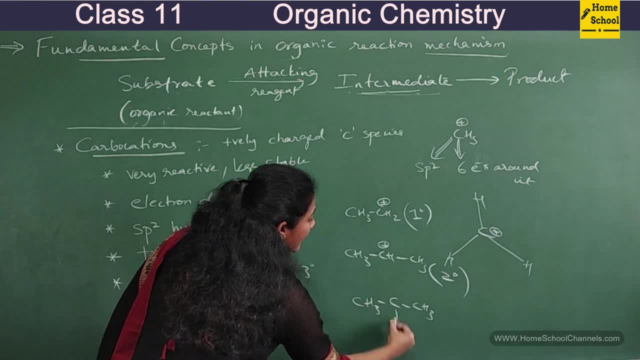 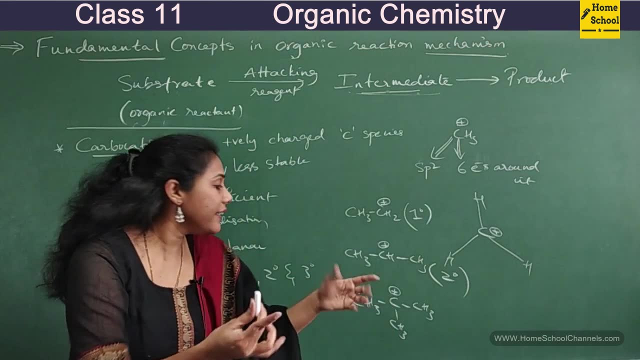 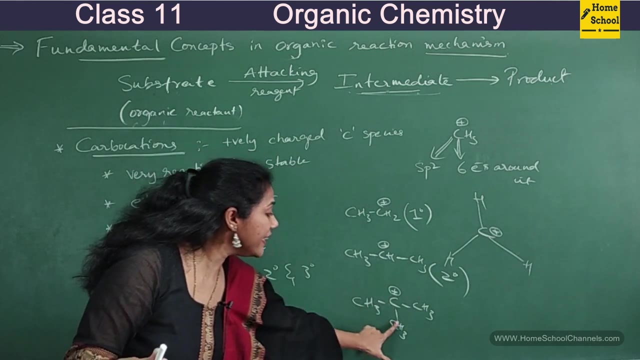 say CH3CH3CH3CH3.. Okay, you look at this carbon. Can you tell me how many other carbons are there around it? One, two, three. So this guy carbon has attachment with three other carbons around it. 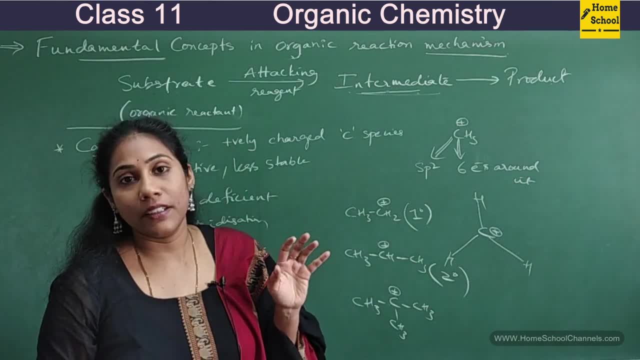 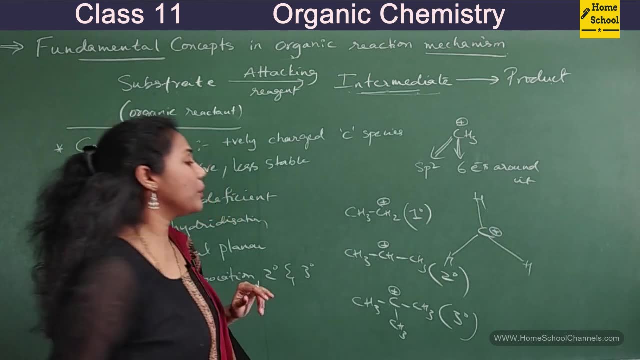 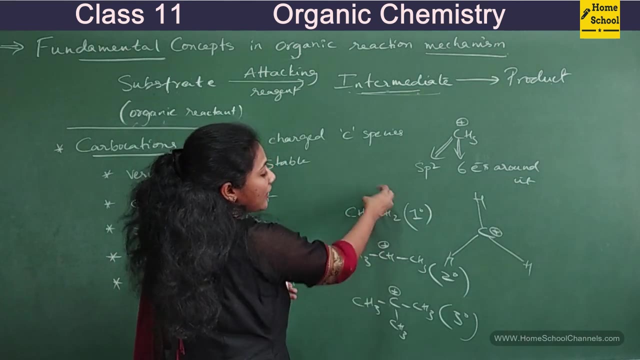 So such a carbon is called as tertiary carbon, Okay, and when you have a positive charge and tertiary carbon, you will call that as tertiary carbon. So this is a positive charge and tertiary carbon carbocation, Okay. so like this: depending on what carbon the charge is there, the positive? 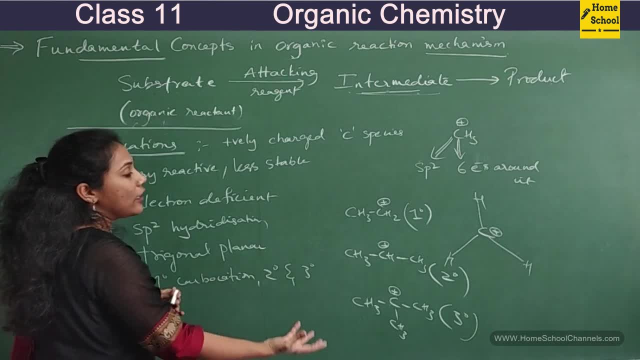 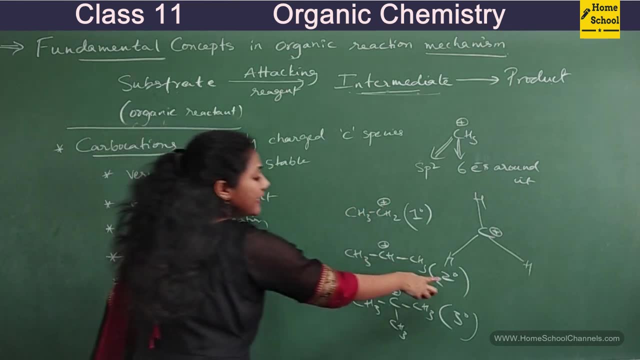 charge is there. we have three types of carbocation. that is, primary, Primary carbocation, where positive charge is there on primary carbon. In secondary carbocation, positive charge is there on secondary carbon. In tertiary carbocation, positive charge is there on tertiary carbon. 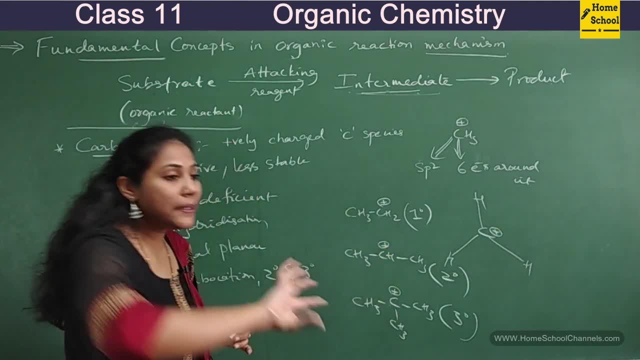 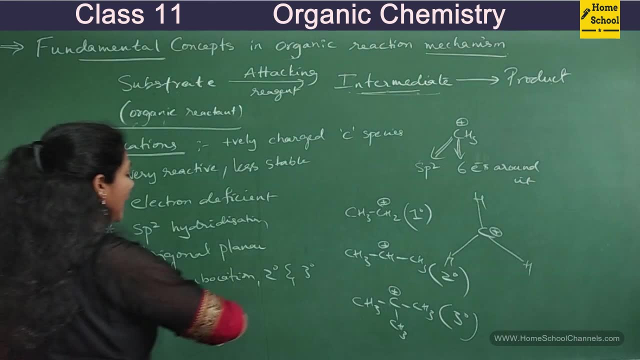 Okay, so tertiary carbon means if a carbon is surrounded by three other carbons, it is called as tertiary carbon. Okay, fine. So among primary carbon, secondary carbon and tertiary carbon, always tertiary carbocation. This is very, very important point, guys. Every time we use this. 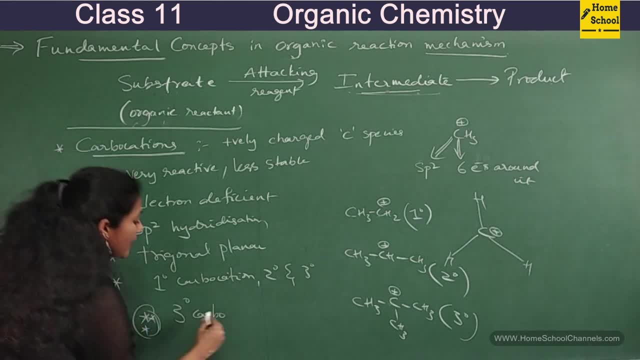 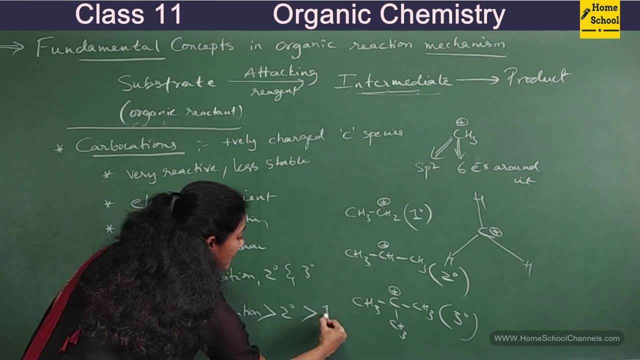 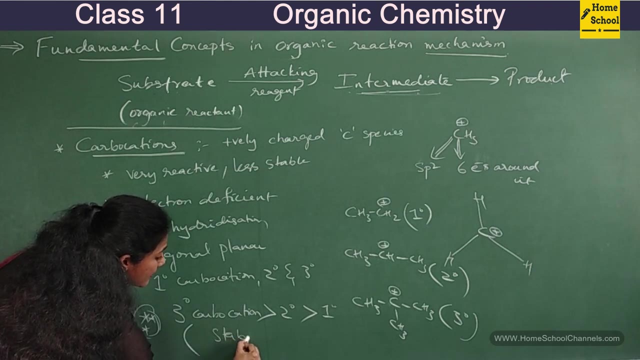 concept in our organic chemistry. So do remember this: tertiary carbocation is always more stable than secondary. Secondary is more stable than primary. Okay, so the order that I gave you is nothing but stability order. Stability order- Okay, or reactivity order- Clear. So which carbocation? 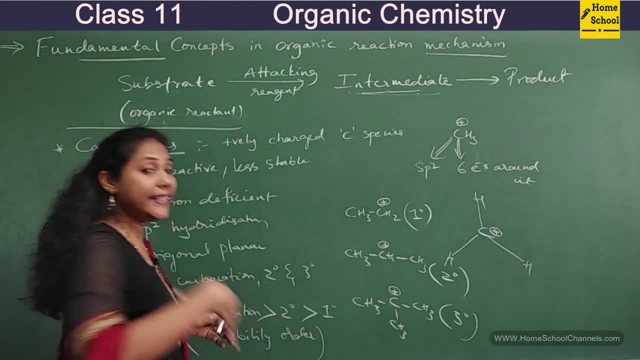 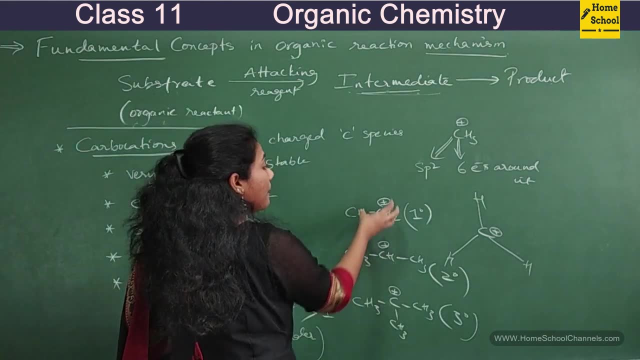 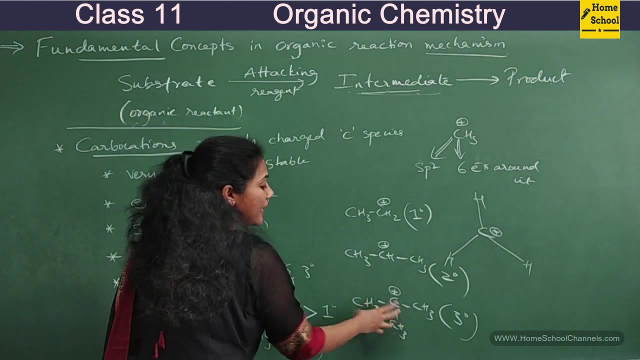 is more stable. Tertiary carbocation is quite more stable and that can be more reactive also, Okay. secondary carbocation is less stable. Primary carbocation is very, very, very less stable. stable, okay, so why? why tertiary is more stable? is because of inductive effect that we will discuss. 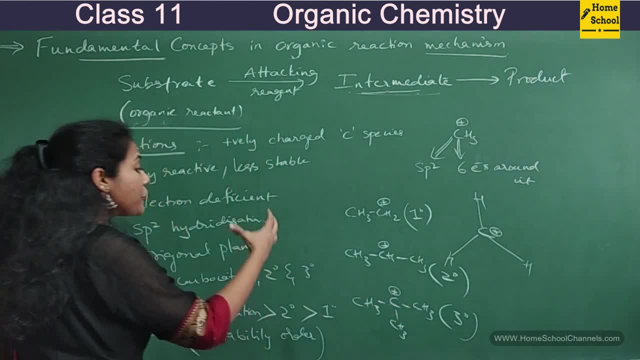 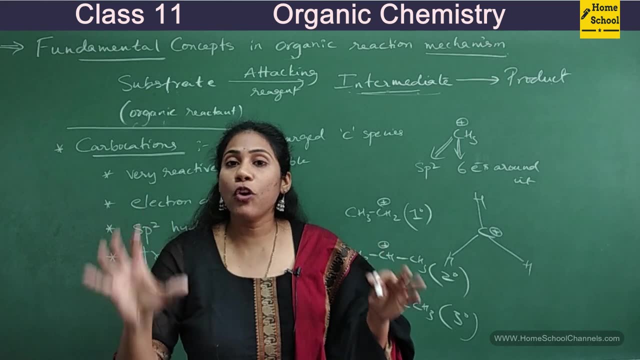 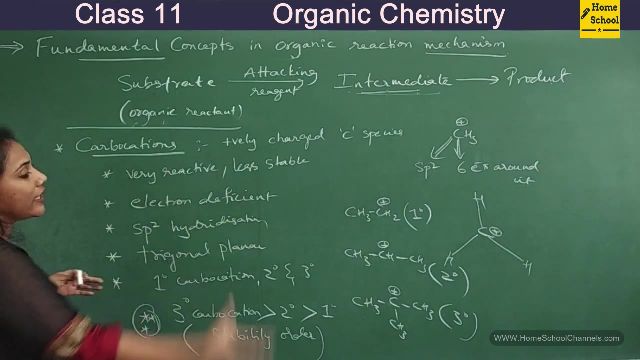 in the next video. okay, so don't worry about the reason. so the reason for this order will be discussed in my next video. that is an inductive effect. do watch that video, don't forget. okay, fine, so this is about the basic idea on carbocations. okay, now let us discuss about. 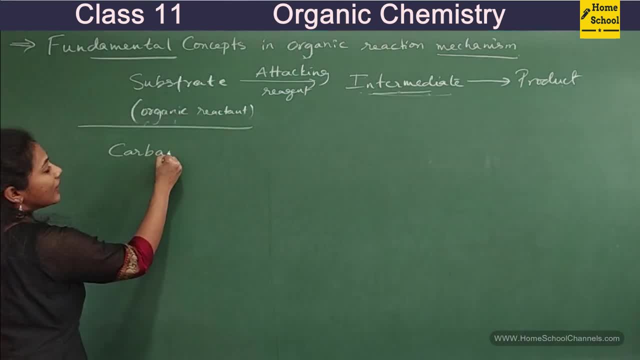 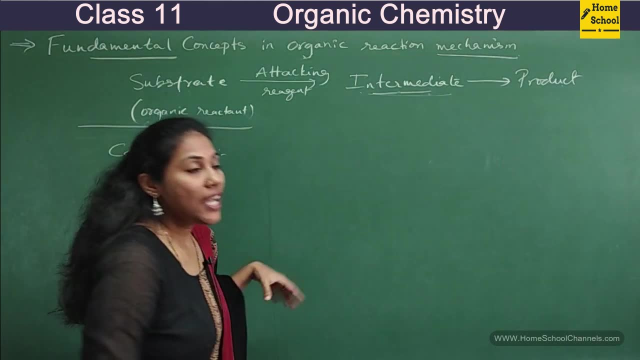 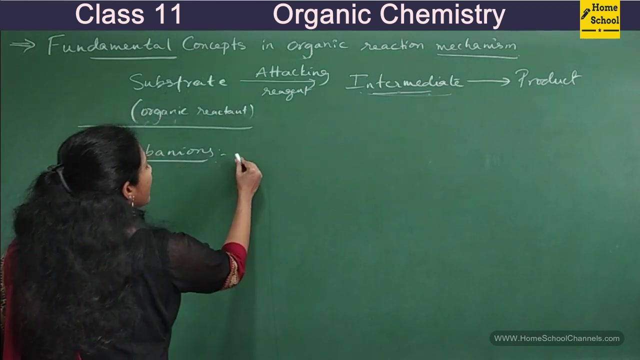 carban ions and free radicals carban ions. so what do you mean by carban ions? even they are formed during heterolytic cleavage. i mean, if the shared pair of electrons move towards carbon, then we get carban ions, isn't it? so what i can write here? negatively charged? 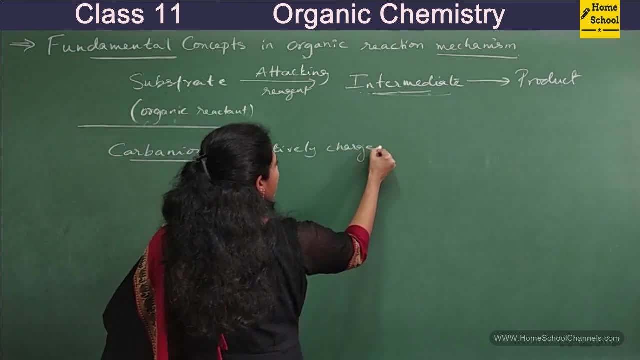 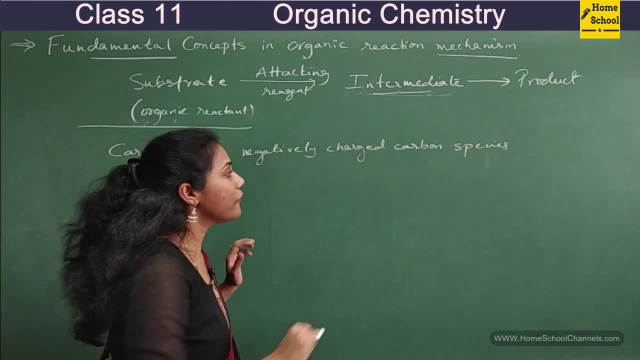 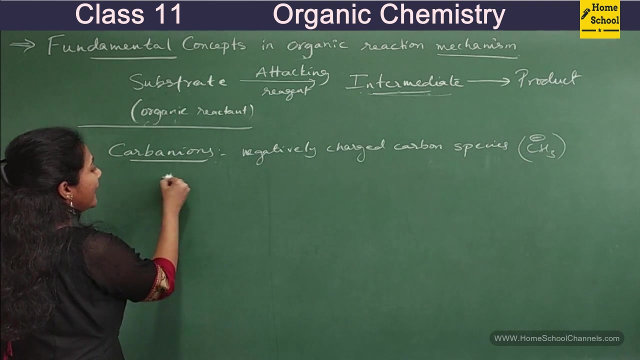 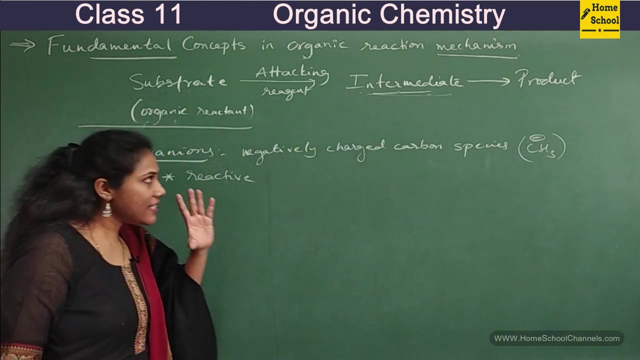 negatively charged carbon species are called carban ions. okay, for example, ch3 minus, right? okay, so even this. carban ions are very, very reactive, so they are one of the type of intermediates itself. just they are opposite to carbocations, right, so they are also very reactive. but the hybridization 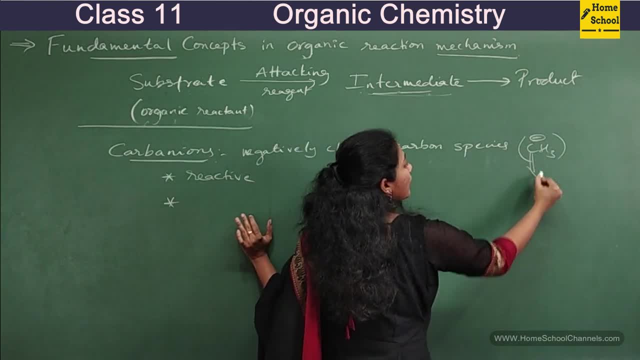 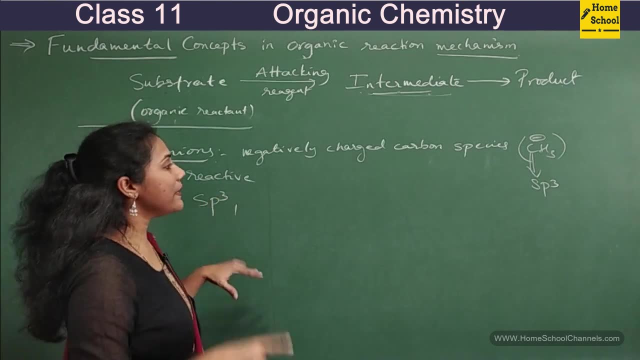 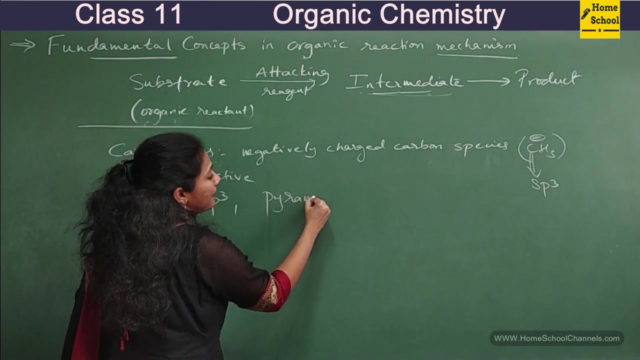 of the carban ions are very, very reactive, so they are one of the type of intermediates itself. this carbon in carbon ion is sp3 hybridization. so they have sp3 hybridization. since they have sp3 hybridization, you know, they will have- uh, you know- pyramidal structure, pyramidal structure. 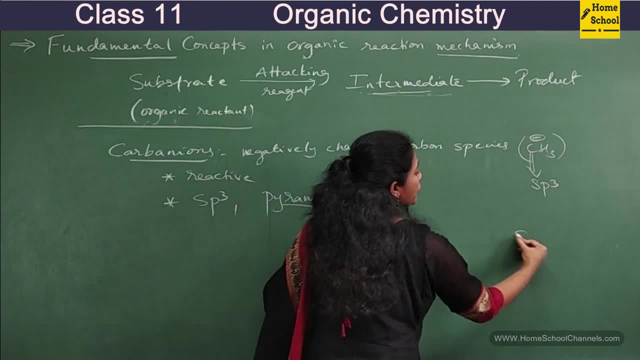 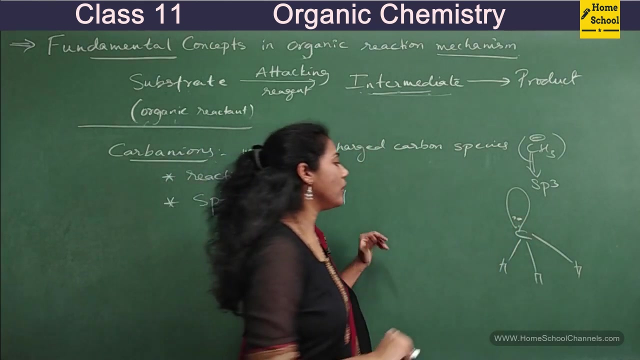 okay, so, if i have to put the structure of this, ch3 minus one hydrogen here, second hydrogen here, third hydrogen here, and there is one negative charge, right, so this negative charge, that means there are two electrons. they are present in orbitals, okay so, uh, this is what we call pyramidal. 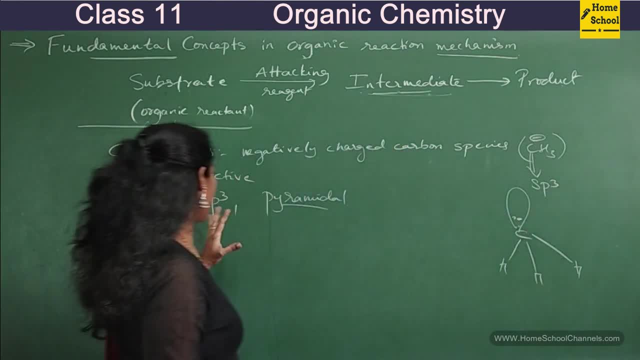 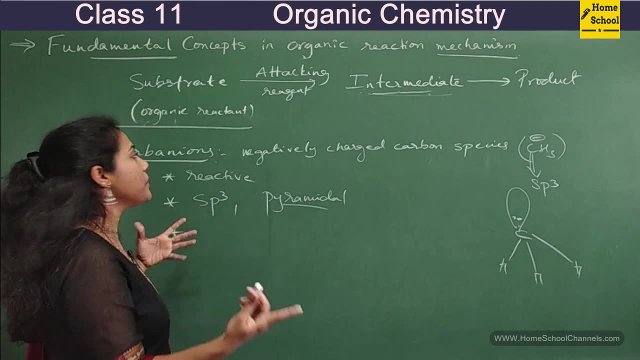 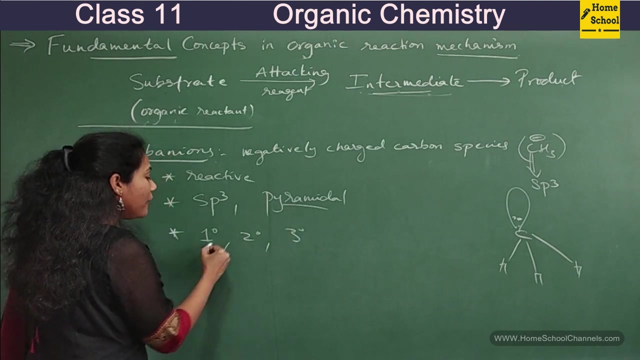 structure. so this carbon is sp3 hybridized. okay, so that is the basic introduction about carbon ion, right here. also, we have three types of carbon ions. uh, they are primary carbon ion, secondary carbon ion and tertiary carbon ion. so if i have to write the structure of primary carbon ion, you know if i 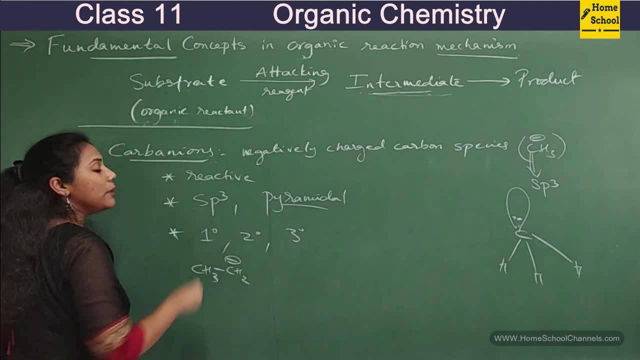 have a negative charge on primary carbon, it is called primary carbon ion. if i have a negative charge on secondary carbon, it is called a secondary carbon ion. so here it's very important to have an understanding about what is primary carbon and secondary carbon. i already told you right carbon. 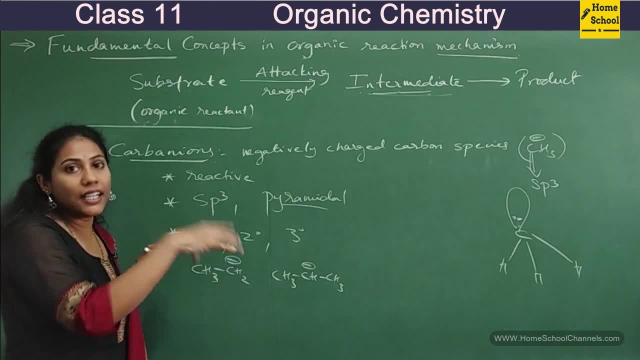 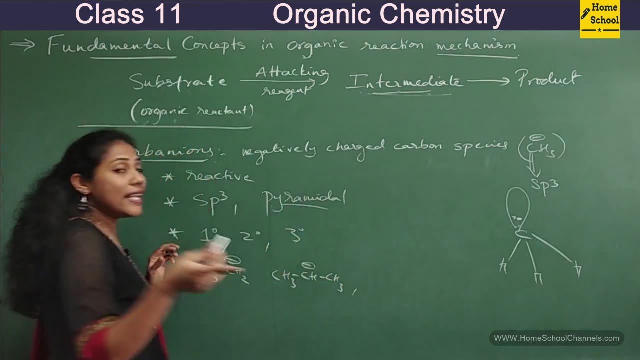 which has got only one bonding with other carbon, not with hydrogen only. you have to look at the carbon if. if a carbon has only one carbon surrounding it, then it's primary carbon. if a carbon has two carbons surrounding it, secondary carbon right. so if a carbon has 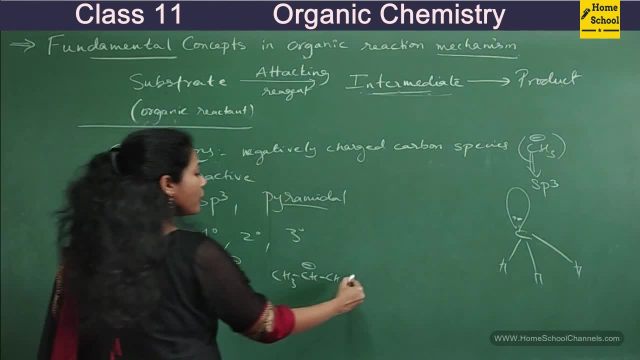 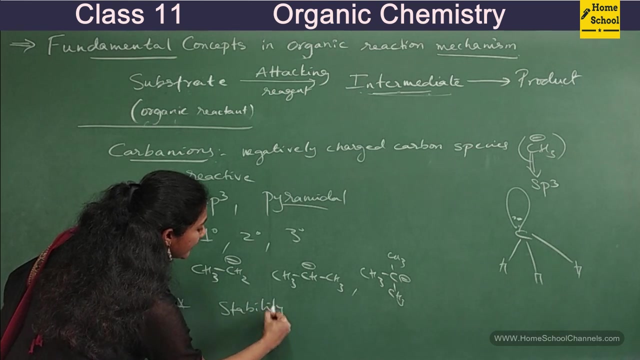 three carbons surrounding it, tertiary carbon. so when you have a negative charge on tertiary carbon, then we will call it as tertiary carbon, okay. so here, if i have to give a stability order, so observe the stability order. it is exactly opposite to carbocatagons, so here: 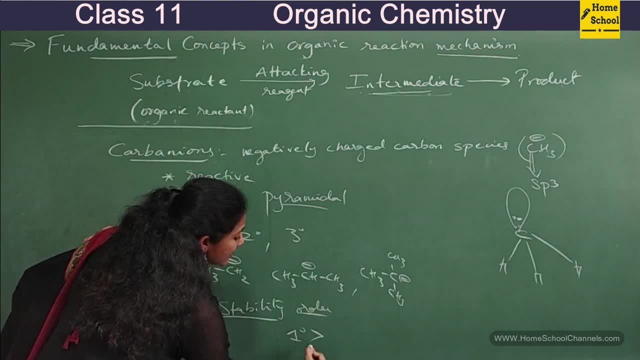 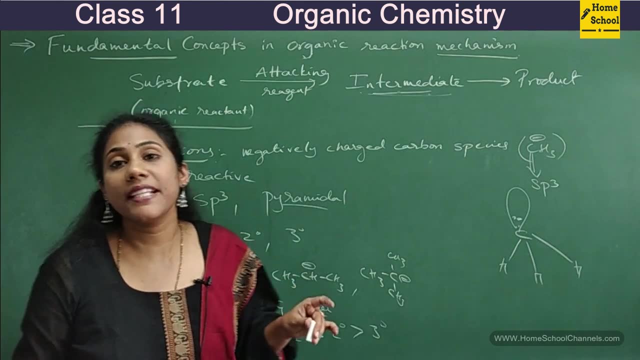 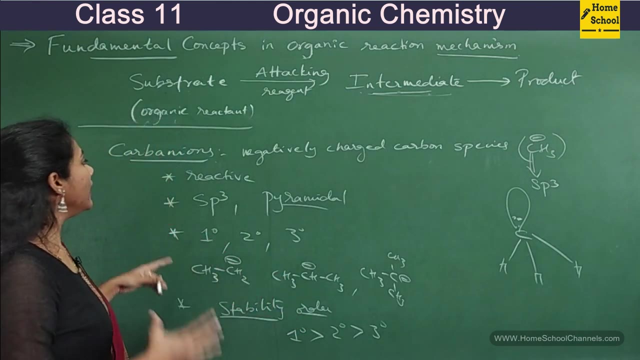 you know, primary carbon ion is more stable than secondary. secondary is more stable than tertiary, so don't worry about the reason, reason i will be explaining in the next video. okay, that is during itective effect. okay, clear. so that is all about carben ions. now let us talk some details of. 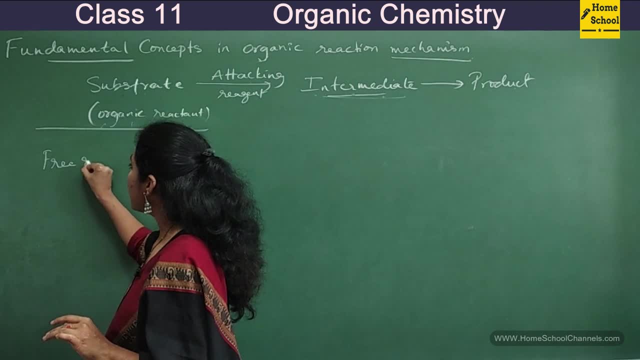 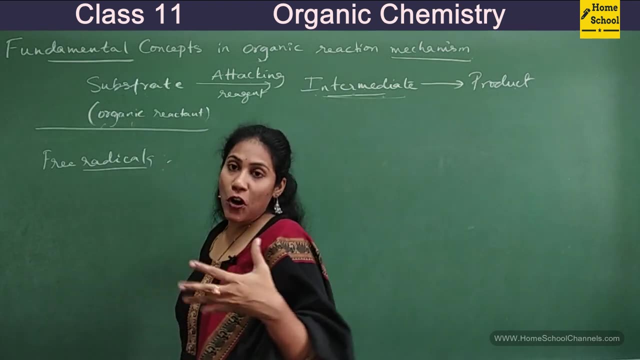 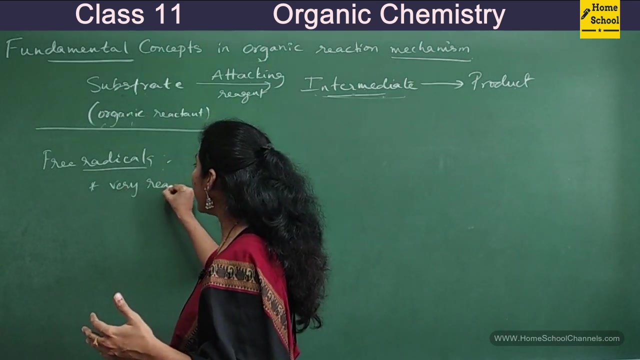 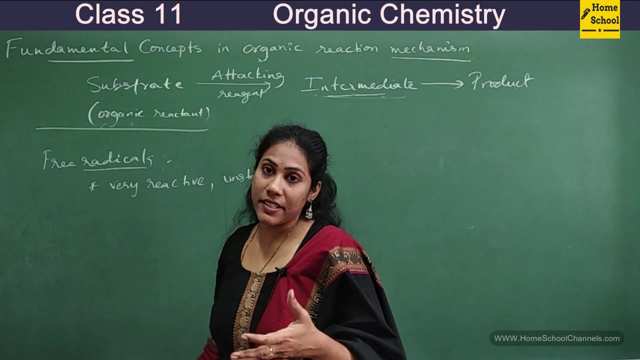 free radicals here- see guys, free radicals. they are also very, very important. uh, type of intermediates, right, and they are formed during homolytic bond cleavage, so they are very reactive intermediates. so they are very much reactive as well as very, very unstable. you know type of intermediates, okay, so, for example, CH3 with one electron. so this is. 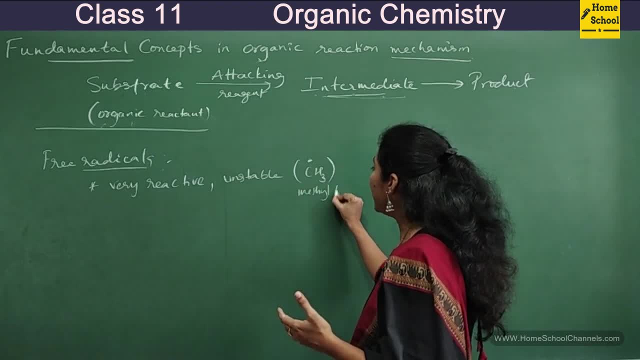 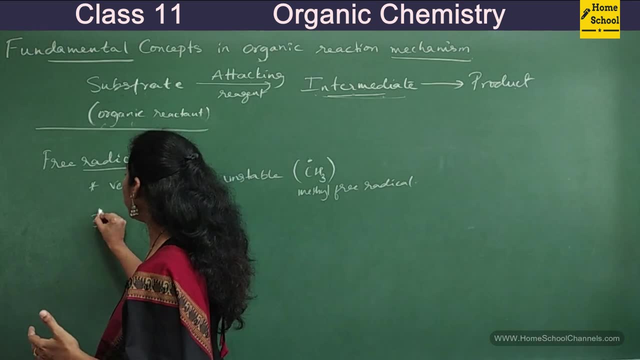 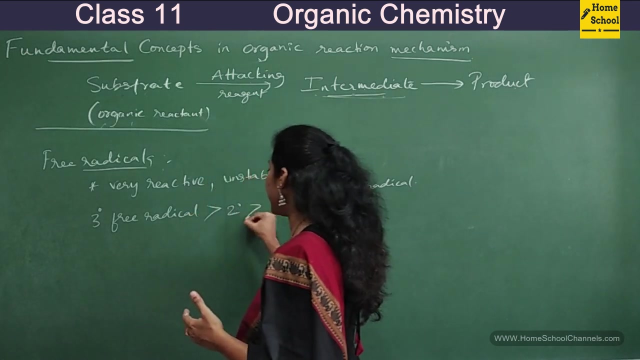 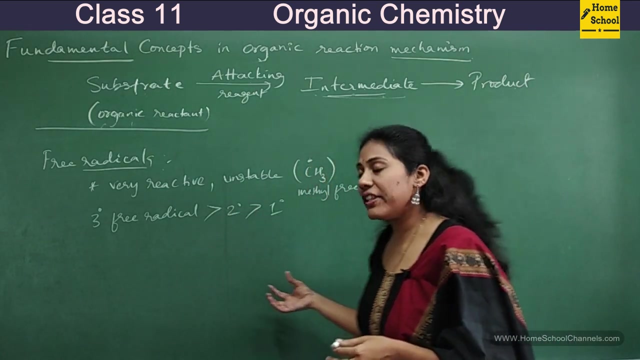 methyl free radical. we call this as methyl free radical, okay, fine. so even here, actually, tertiary free radical is more stable than tertiary. free radical is more stable than secondary. secondary is more stable than primary, just like carbocations. you have a stability order here. here also, the reason is inductive effect itself, which we will be discussing in our 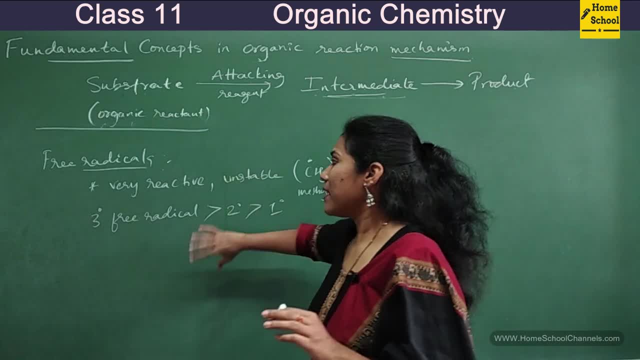 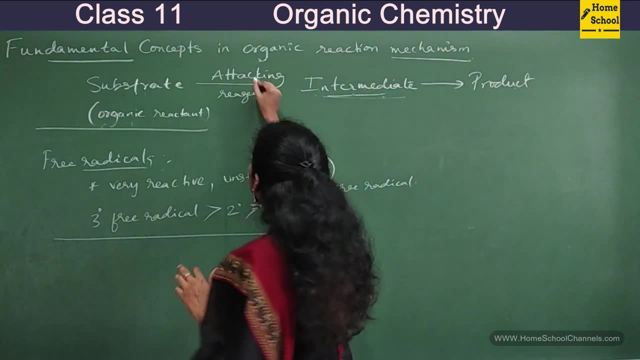 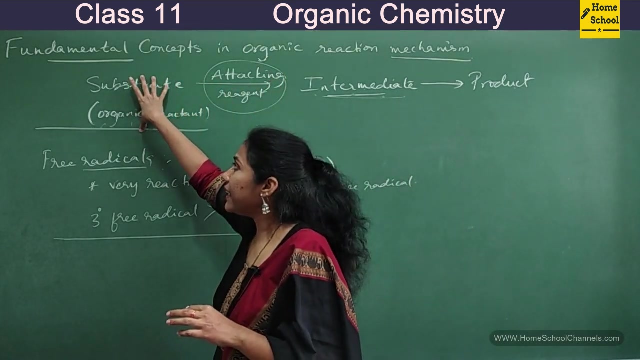 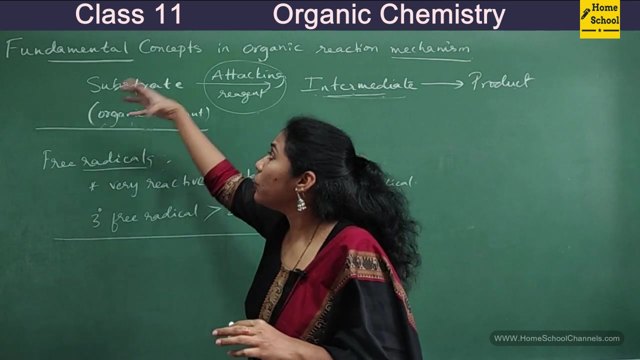 next video. okay, so that is some basic aspects of free radical. okay, so, after this much, let me discuss about attacking the type of attacking reagents. okay, see: substrate undergoes homolytic cleavage or heterolytic cleavage based on the type of attacking reagent. okay, so why do substrate? uh, is undergoing some. 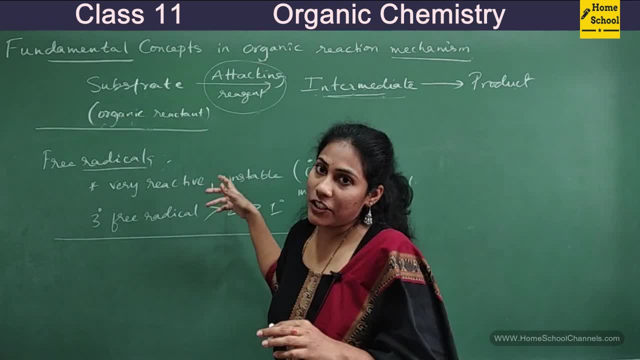 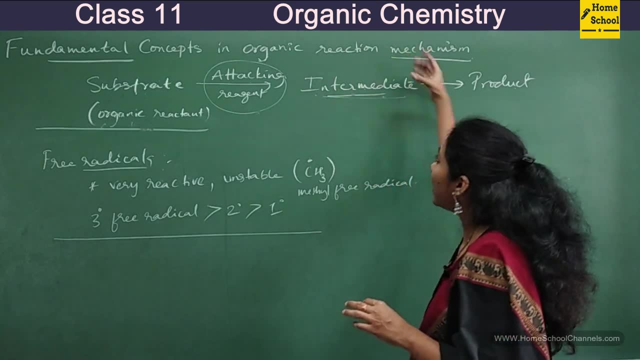 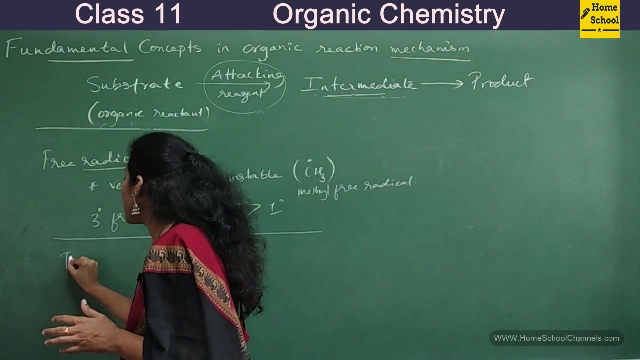 structural changes, it is due to an attacking reagent. okay, so we discussed the cleavages that can happen in a substrate and we also discussed what are the types of intermediate that can be formed. now we will discuss about the types of attacking reagent. okay, types of attacking. reagents, right. so mainly there are two types of attacking reagents, guys. one is called as nucleophiles, the other one is called with the name electrophiles- nucleophiles and electrophiles. so here, what do you mean by nucleophiles? it's very simple: nucleophiles are nucleus loving. 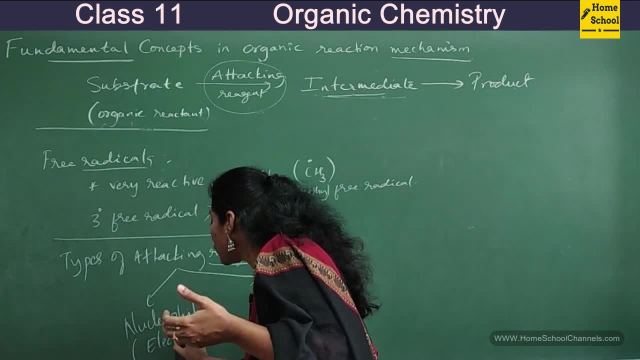 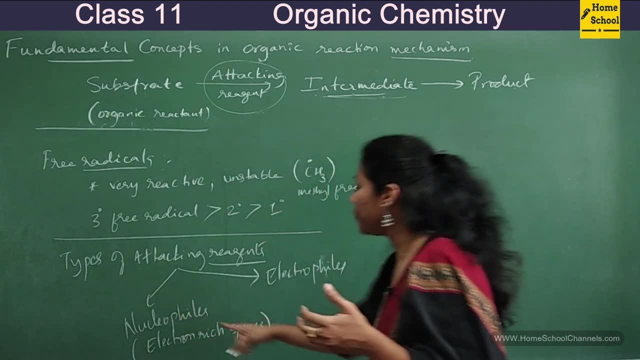 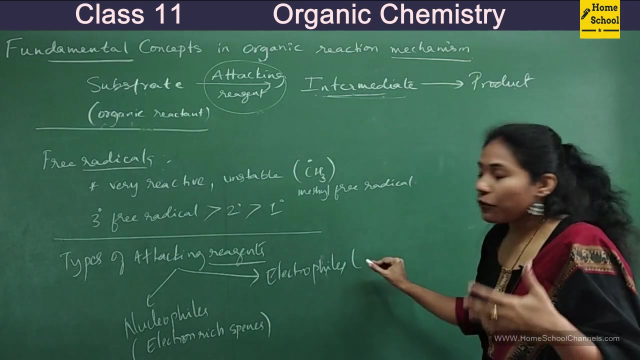 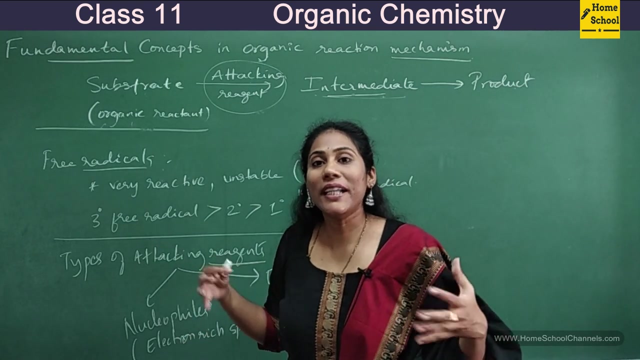 that means they are actually electron rich species. electron rich species are called as nucleophiles and electrophiles- nothing but electron loving species. like when do we love electron? when do they love electron when they do not have enough electrons? isn't it when we don't? 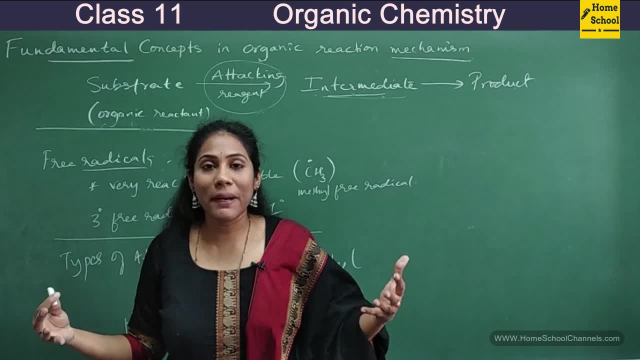 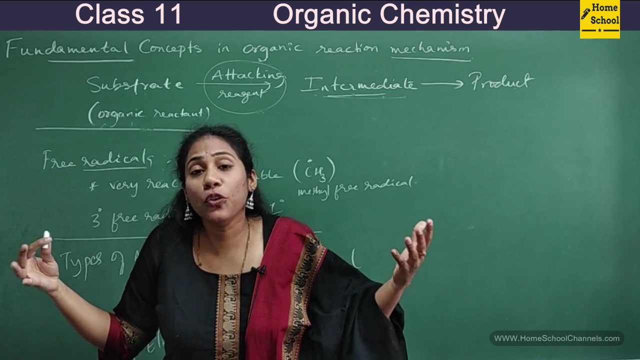 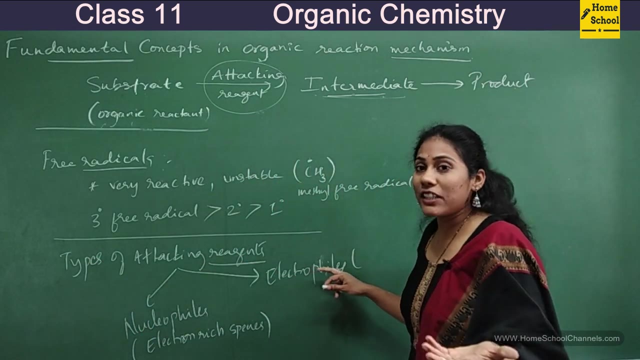 have enough money, then we allow to earn money right. we will have more power, passion towards money. So when we don't have something, we love that and we want to have that always right. So the same concept here: they are electron loving. Why do we call them as electron? 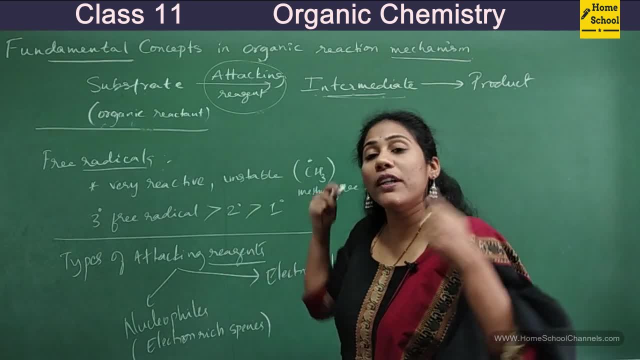 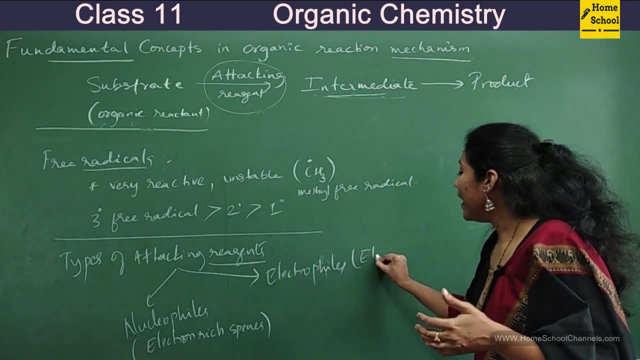 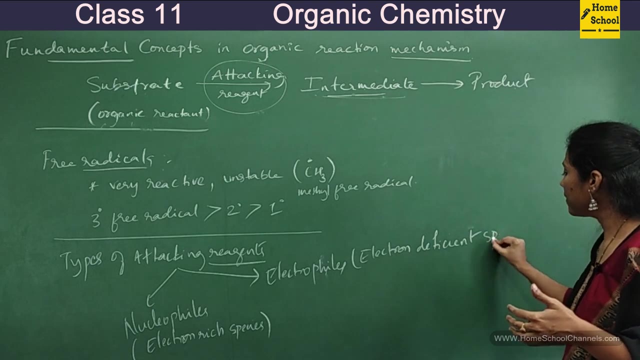 loving Because they lack electron, right? They always wanted to have electrons, enough electrons, So that is the reason we call them electrophiles. So they are electron deficient species, Electron deficient species. Okay, so these are the shortcut definitions for nucleophiles and. 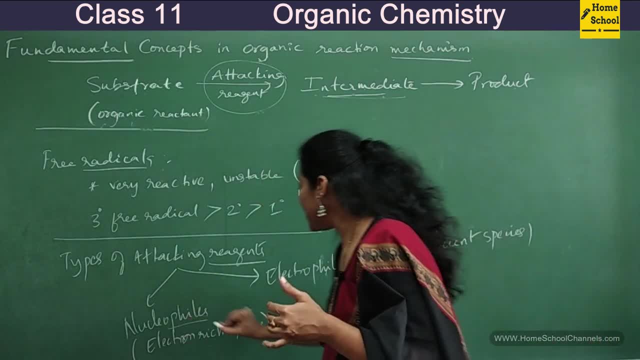 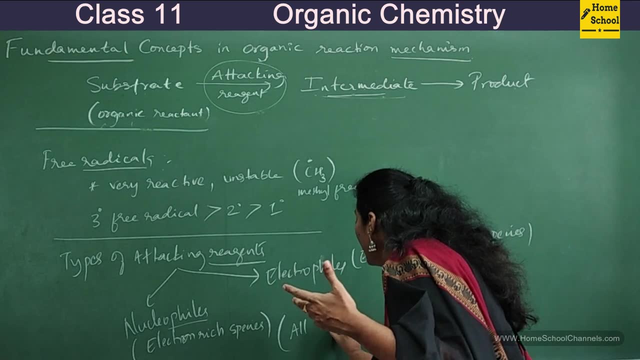 electrophiles. Let us see an example. See nucleophiles examples. all negatively charged ions can act as nucleophiles, So all negative ions. Okay, for example, you have CH3 minus right The intermediate, that is CH3.. 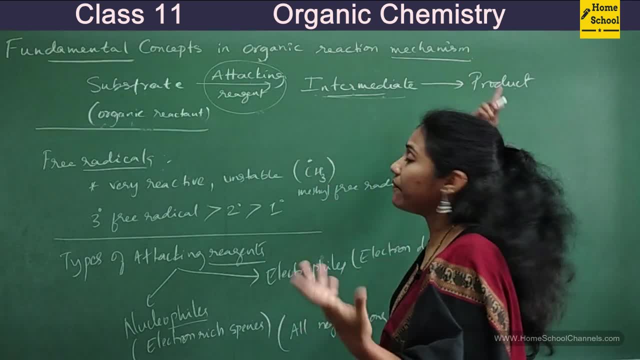 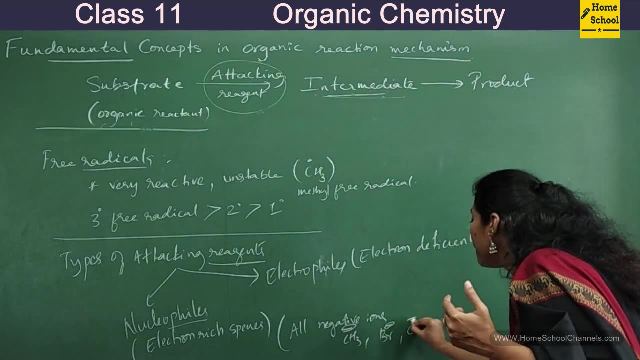 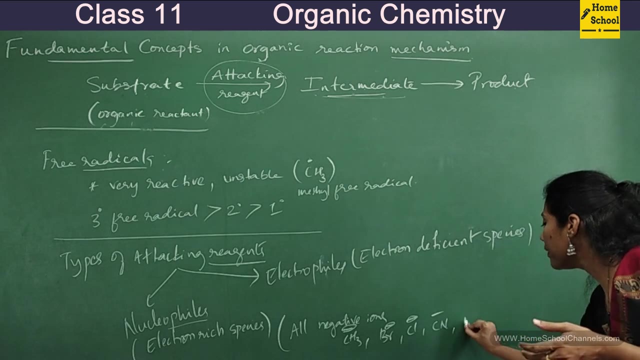 CH3 minus itself can act as an attacking reagent somewhere, right. So all negatively charged ions like Br minus, Cl minus, say you have an ion Cn minus- okay. Or any minus ion. Sometimes you may have H minus hydride ion- okay. So any negative ion can act as an electrophile. Not only that. 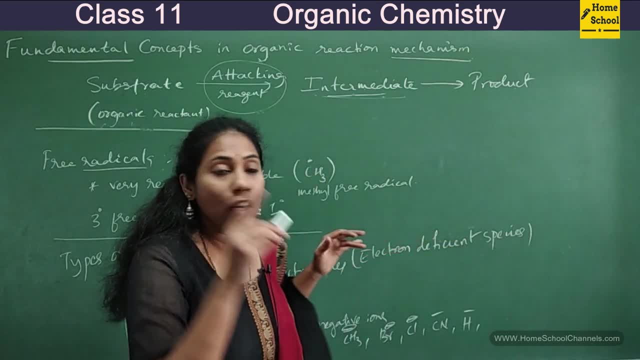 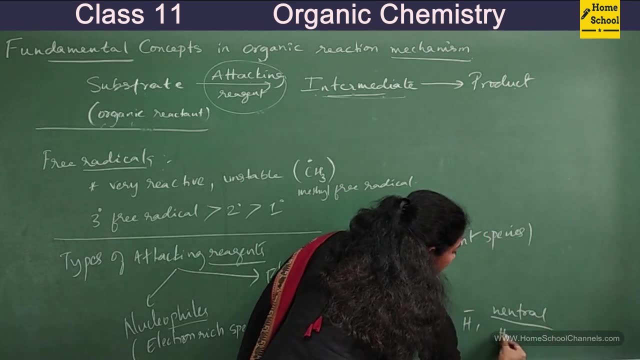 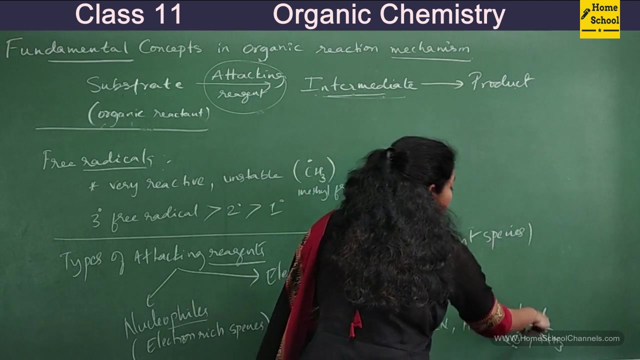 some neutral molecules with lone pair of electrons, okay Say neutral molecules which have lone pair of electrons. like H2O, there are two lone pairs on oxygen, NH3, there are one lone pair on nitrogen, right. So any negatively charged ion or any neutral molecules with lone pairs can be an example for. 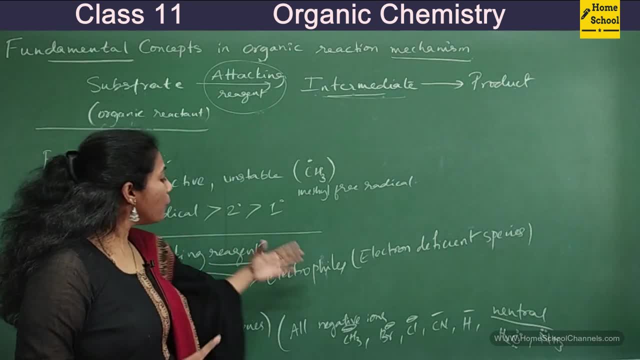 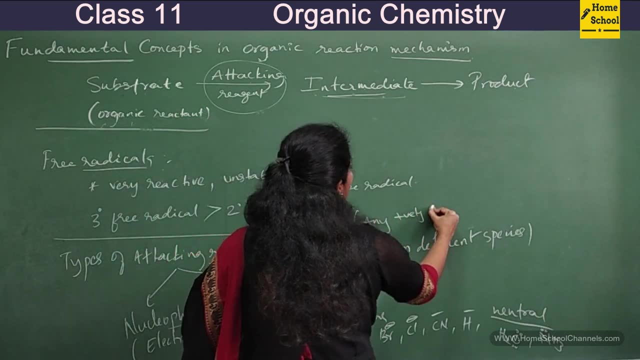 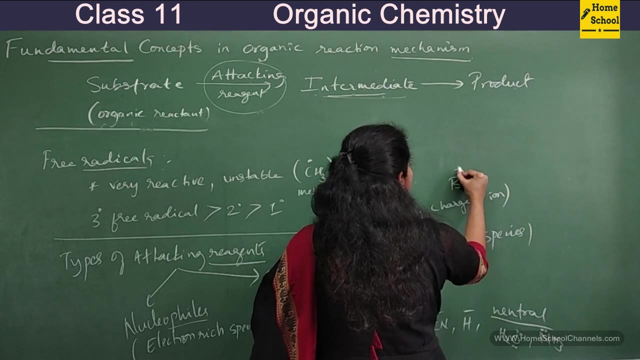 nucleophiles. So any negative ion can act as an attacking reagent somewhere, right? So any negative ion can act as an electrophile. Okay. So similarly, what can be an example for electrophile? Any positively charged ion. Any positively charged ion can be an example. For example, you know, Br plus can be an example. 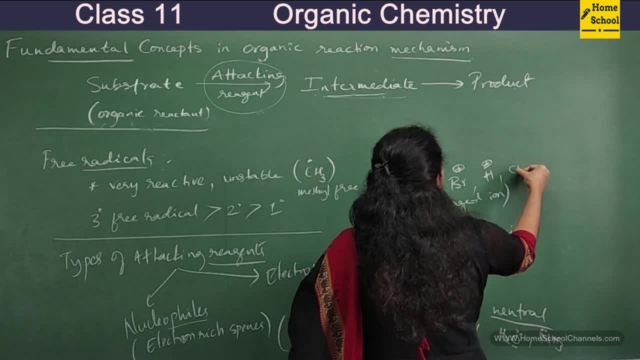 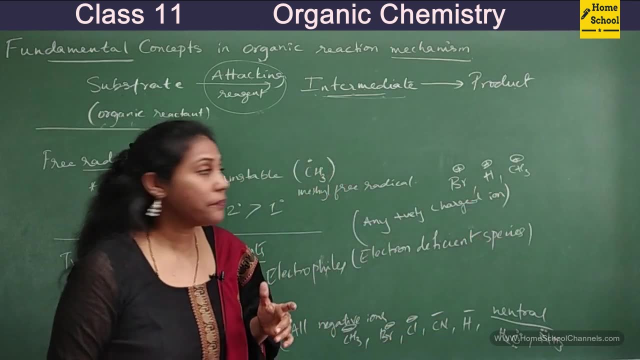 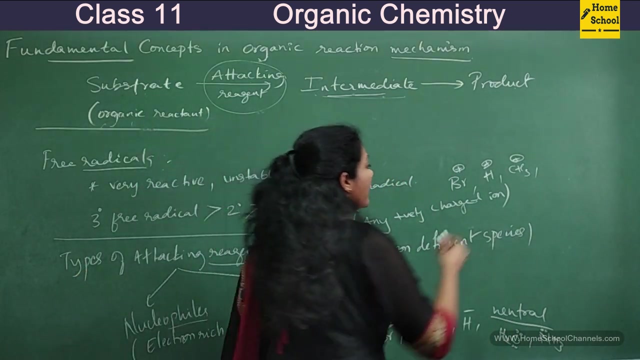 or H plus can be an example. or you have seen carbocation, CH3 plus can be an example, right? So any positively charged species. And there are some neutral species which lack electrons. You know, for example, BF3.. Can you think of how many? 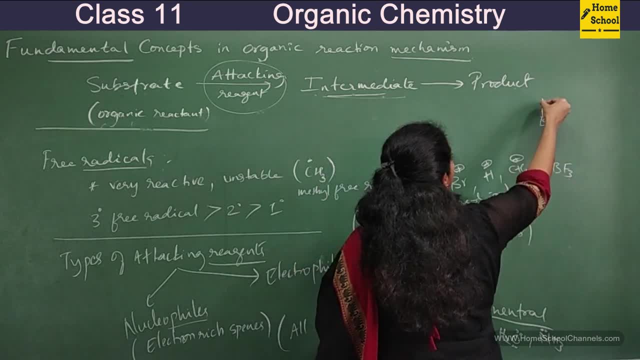 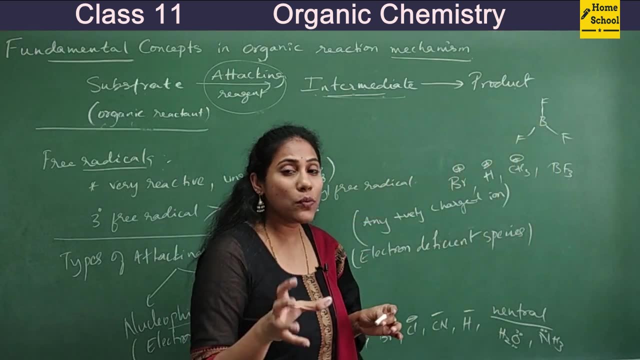 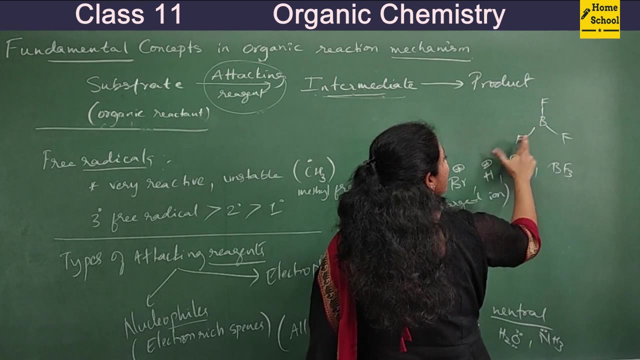 electrons are there on BF3?? You see BF3 molecule. if I have to write its structure, does boron satisfies octet rule. Octet rule in the sense, what? Having eight electrons around it, How many electrons does our boron has around it? One, two, three, four, five, six, three bonds in the sense. 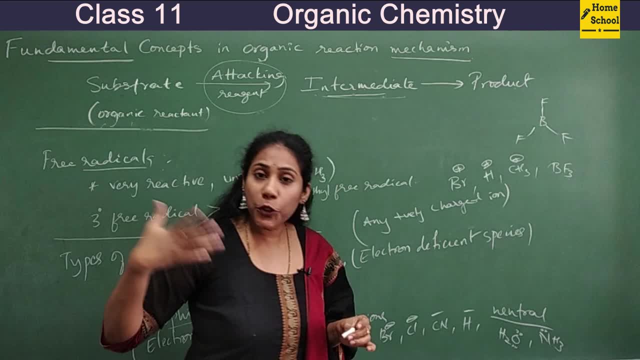 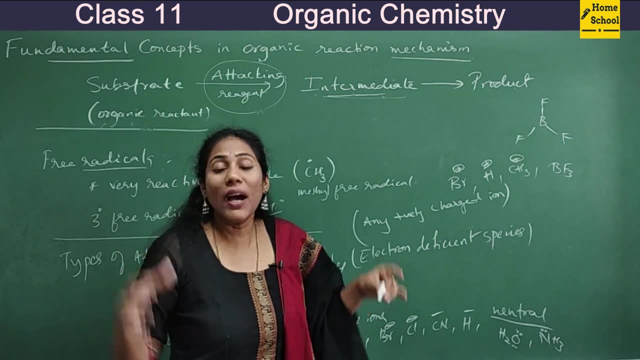 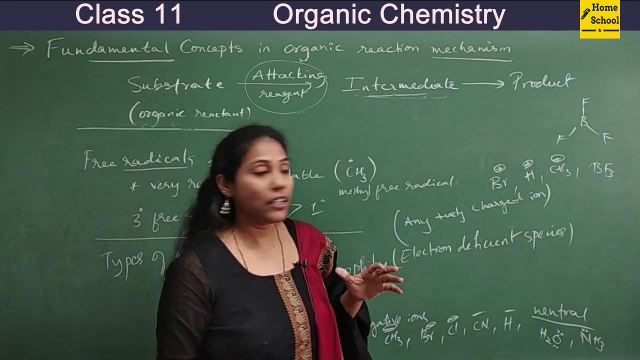 Three, three electrons are there around it, So it want two more electrons for the stability, It wants two more electrons to satisfy the octet, to have that octet around it, right? So such molecules also can be an example for electrophiles. Okay, So BF3, ALCl3, ZnCl2.. 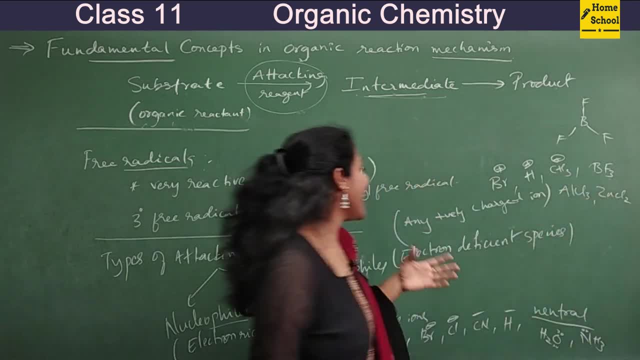 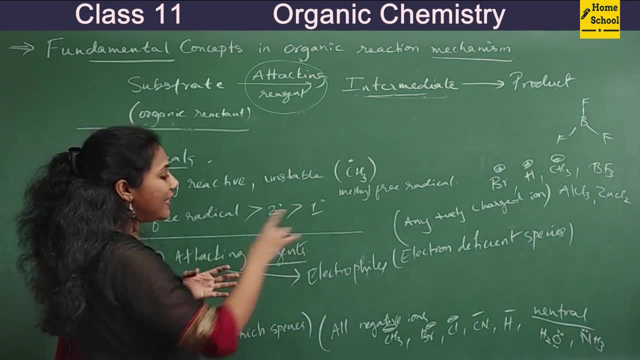 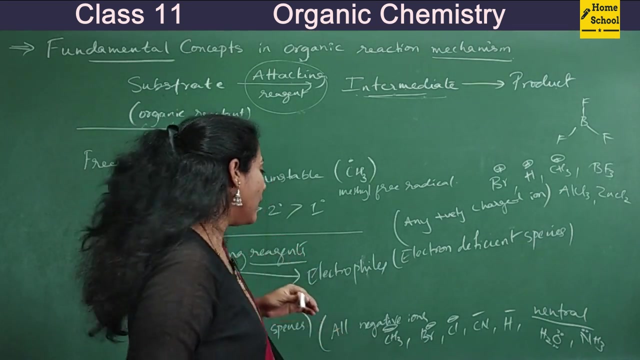 So all these neutral molecules also can be an example for electrophiles. So these are the two types of attacking reagent: nucleophiles and electrophiles. So you must able to give a differentiation, or you must able to differentiate between nucleophiles and electrophiles. That is the 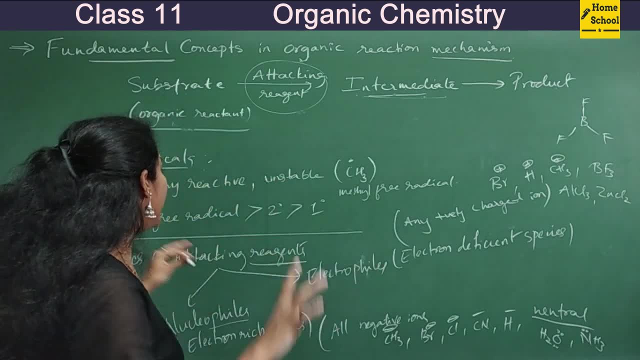 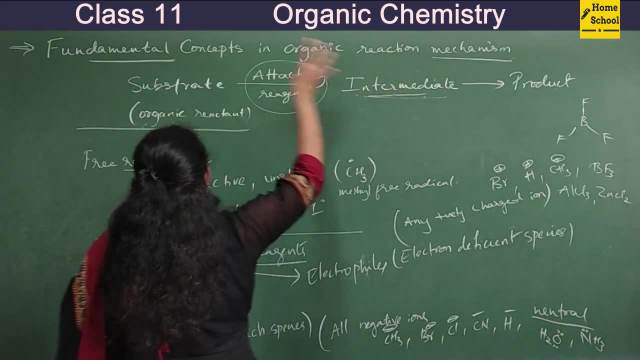 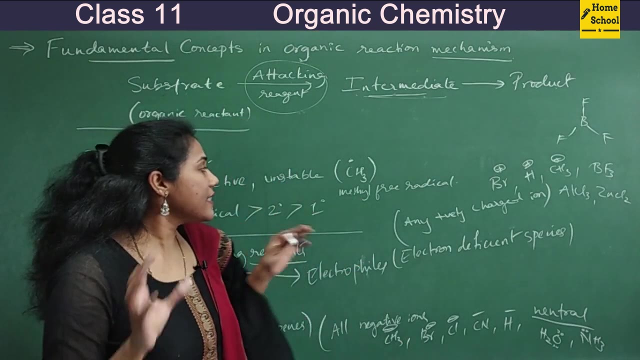 most important one, Clear. Okay, So we have discussed about nucleophiles and electrophiles. We also discussed about the different types of intermediates and we discussed about the different types of cleavages. right, So now try to understand, always whenever an organic reaction must happen. 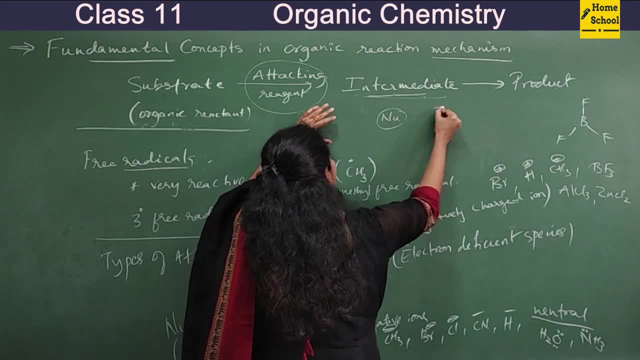 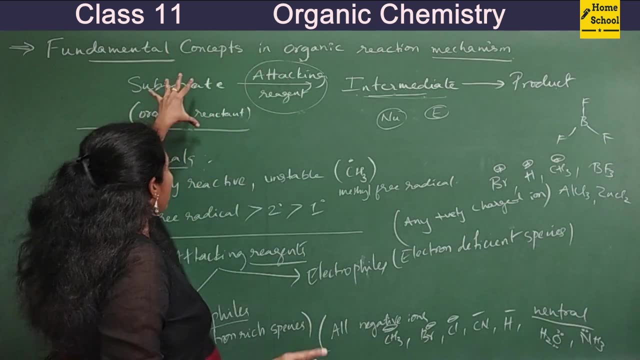 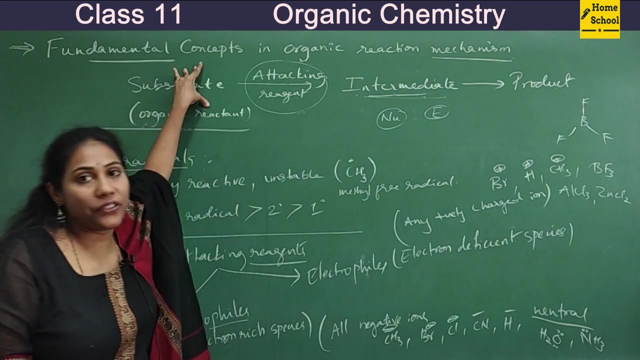 it should happen between a nucleophile and electrophile. Okay, so if the attacking reagent is nucleophile, then there must be some carbon or some atom in a substrate that must be acting as electrophilic. Okay, only then the reaction takes place. So all organic reactions are. 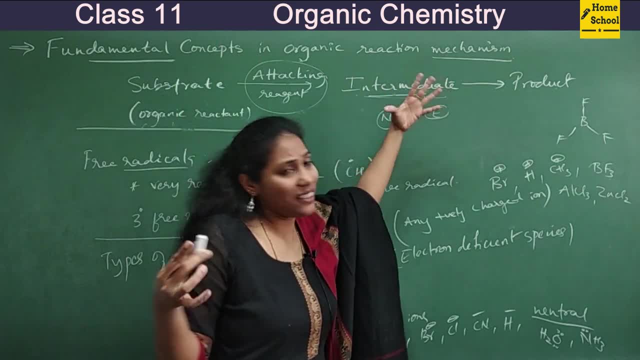 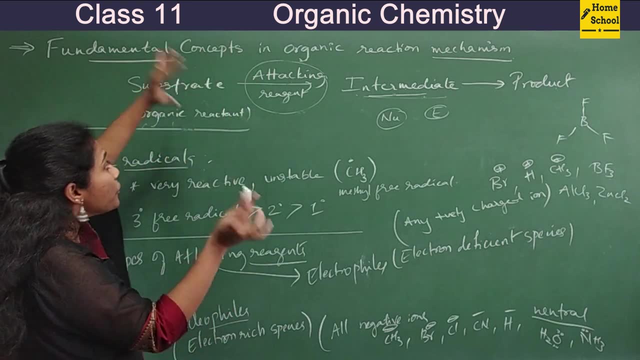 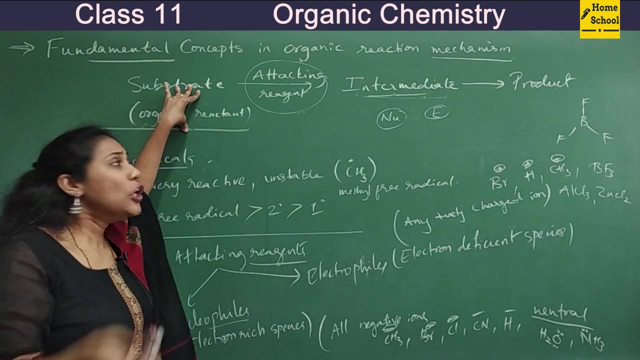 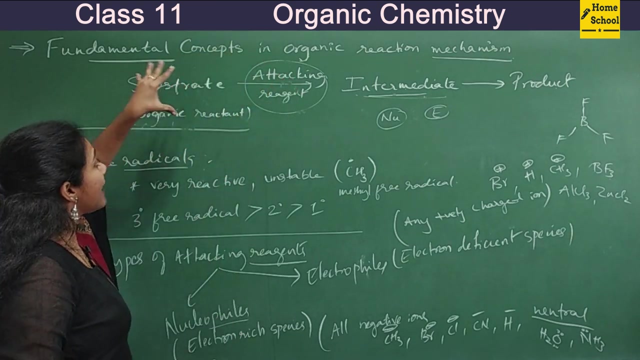 happening between some electron rich guy and electron deficient guy. okay, say, if you take some nucleophile as attacking reagent and you should have an idea that there must be some atom in the substrate that must be electron deficient, only then the reaction possible. in case, if you are taking up electrophile as the reagent, there must be some atom that is rich with. 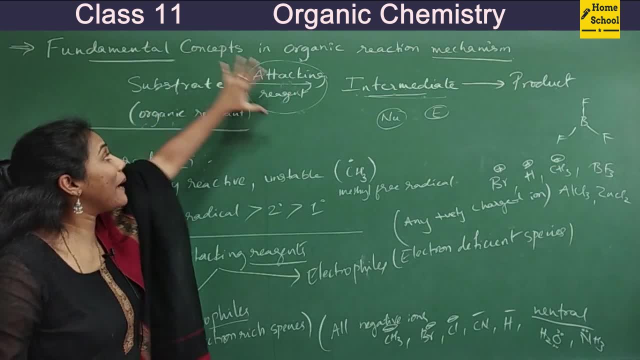 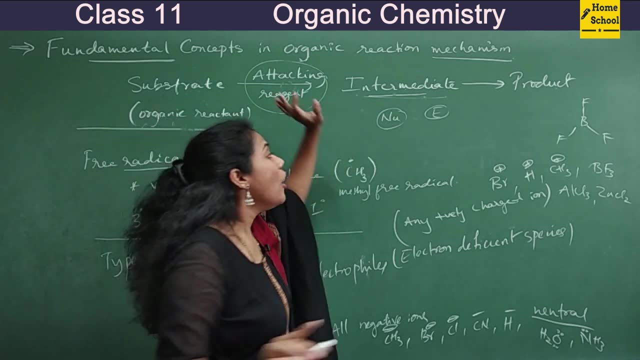 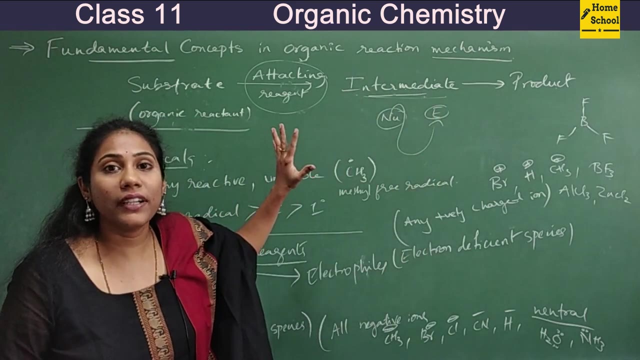 electrons in the substrate. only then the reactions would happen between them and that leads to the formation of intermediates. okay, so this is the general logic, guys. always an organic reaction happens between nucleophilic center to electrophilic center. okay, so if you take attacking 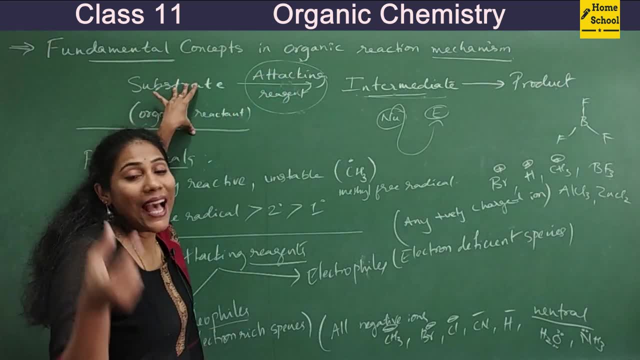 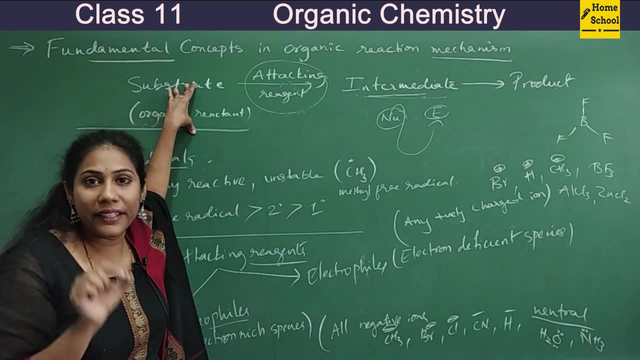 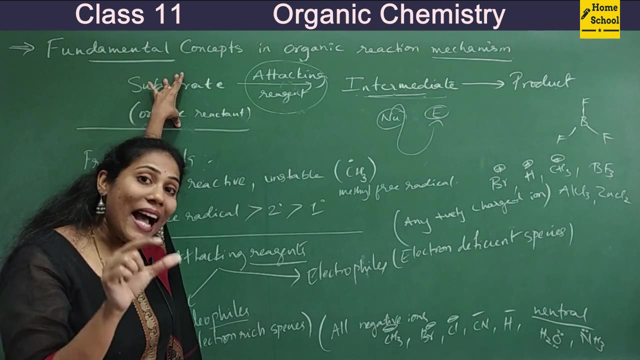 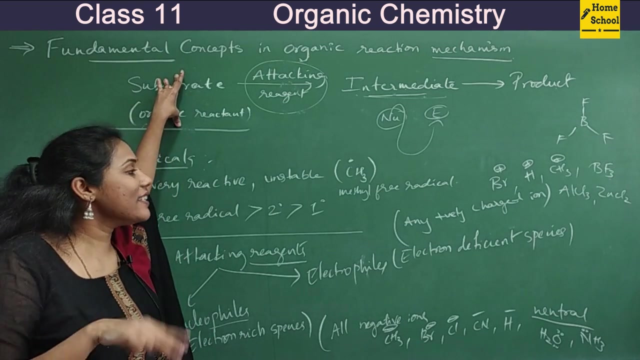 reagent as nucleophile, then your substrate must be having some electrophilic center, some electron deficient atom or a center, a point. okay. if you take up electrophile as a reagent, then our substrate must have had some atom with electron richness, okay, some atom which is nucleophilic in nature, okay, so that is how. 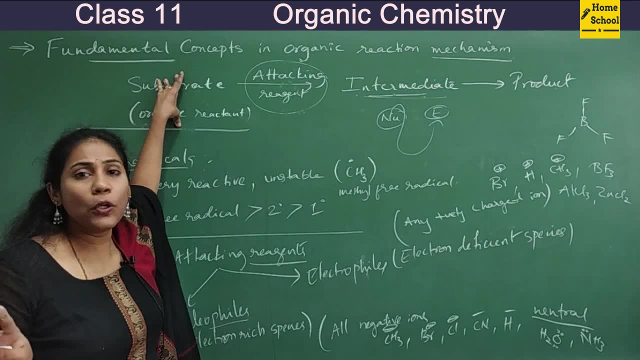 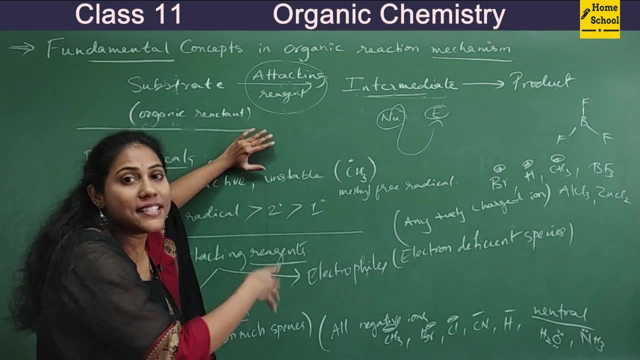 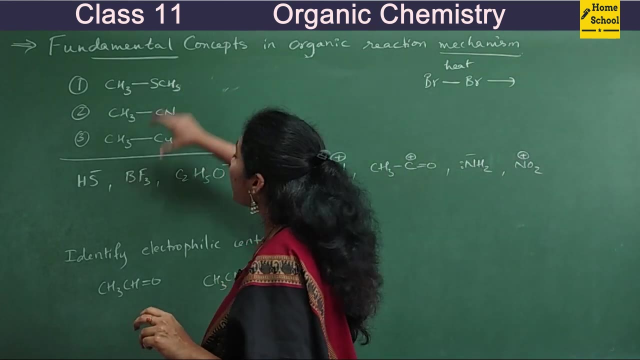 always organic reaction takes place. now let us look at few questions from your ncrt textbook so that you will have better idea on all of these that we have discussed. look at these questions, guys, see. uh, the first questions. you have to show how a cleavage can takes place, whether homolytic. 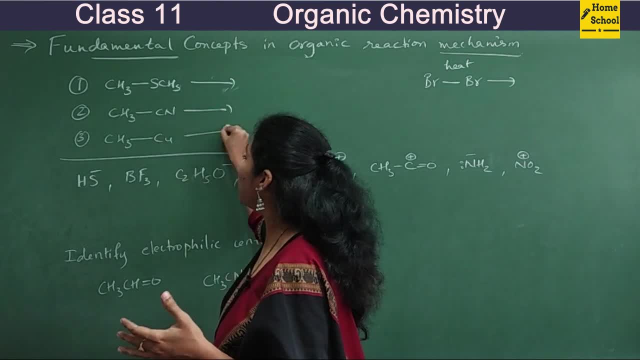 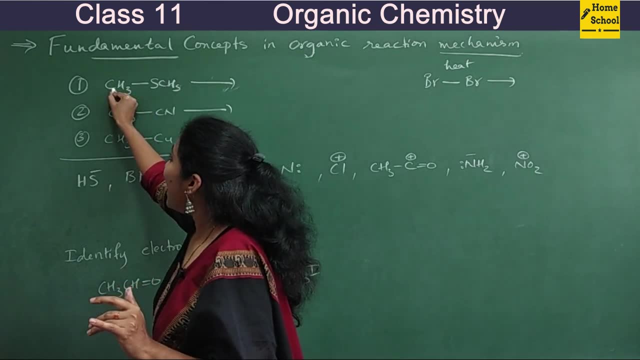 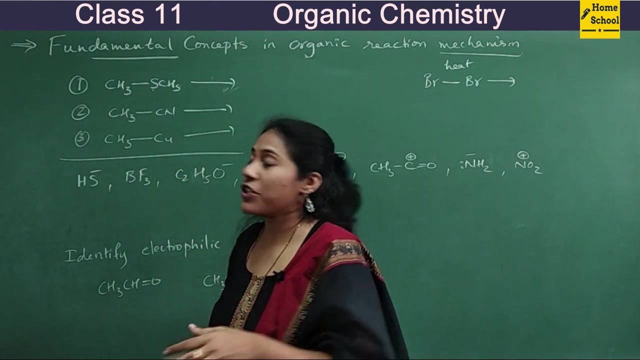 cleavage or heterolytic cleavage after cleavage. what do you get? that's what you have to do. say, ch3 bond s is ch3. compared to this, carbon s is more electronegative, right? so here you will definitely observe heterolytic bond cleavage when there is a electronegativity difference. 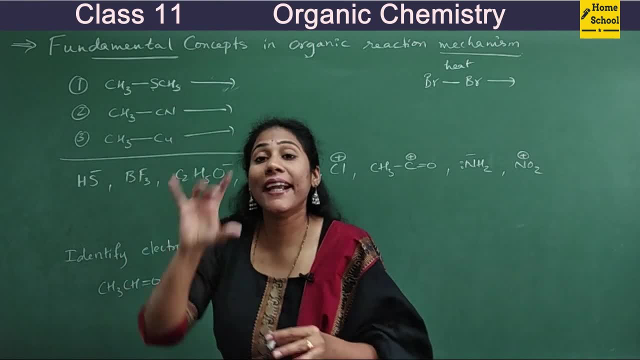 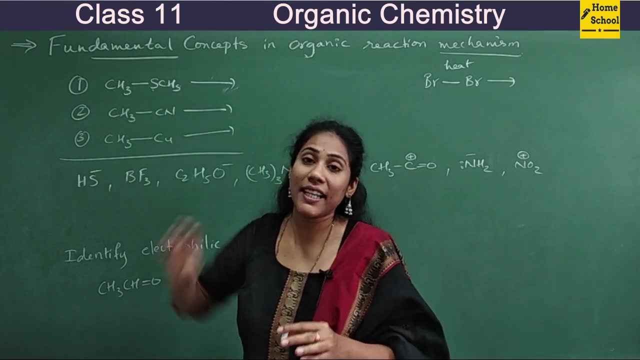 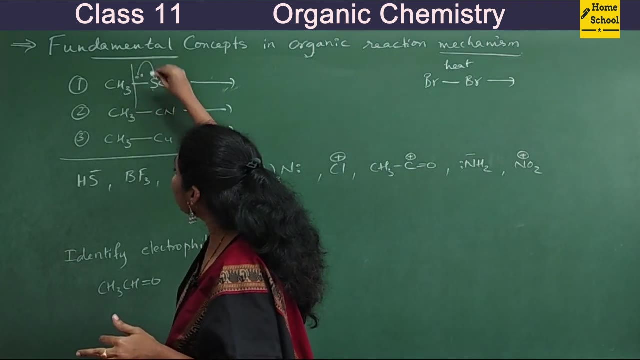 between the two bonded atoms. as we have seen earlier, the two bonded atoms are getting shifted to sulfur and correspondently heterolytic cleavage takes place, and the bonded pair of electrons always gets shifted to most electronegative atom. so here what happens: bond is cleaved in a such a way that both electrons 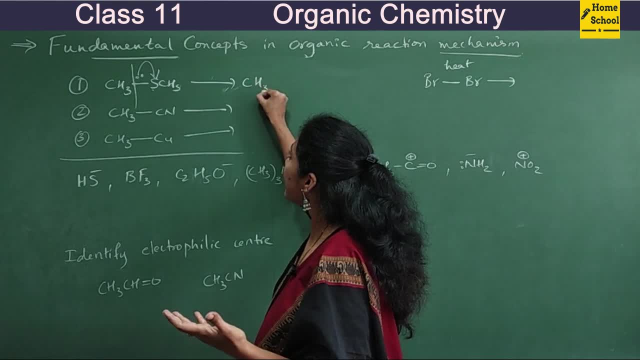 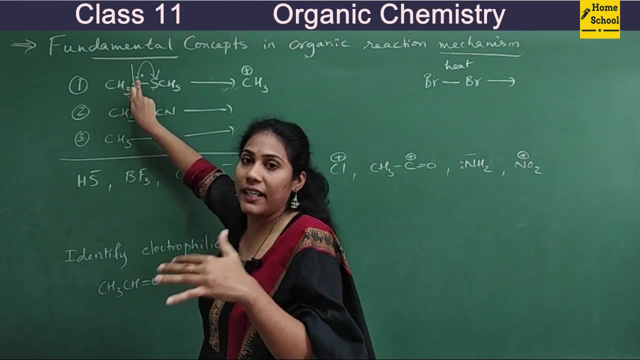 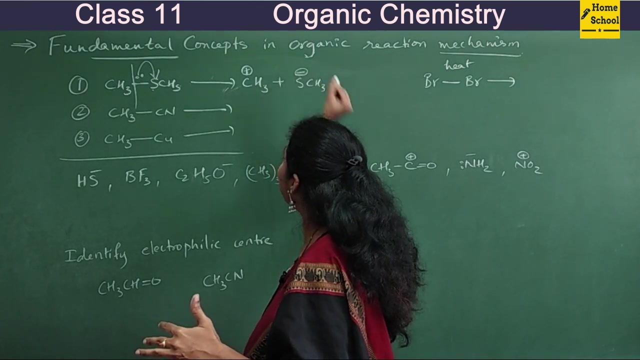 are getting shifted to sulfur, to this group. so what are the species that you will get? you will get ch3 with positive charge because this carbon, this ch3 group, has lots last its electron right. So that's why CH3 plus and you will have SCH3. on S, you will have a negative charge. 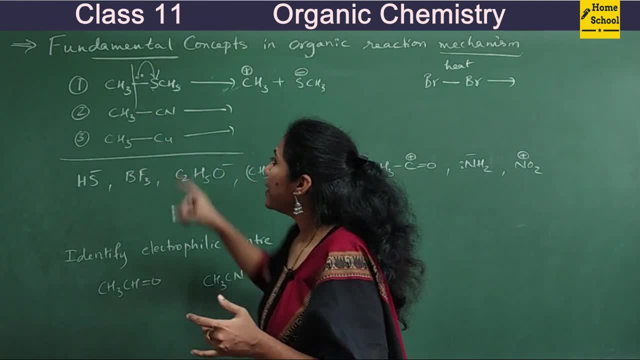 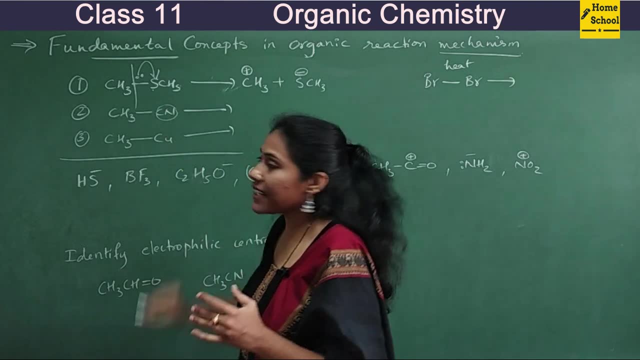 Okay, fine. So here, how does the cleavage takes place? CH3, CN, So C, C, but here C is there in the form of CN, So this is the most electronegative group. As a group it is more electronegative. 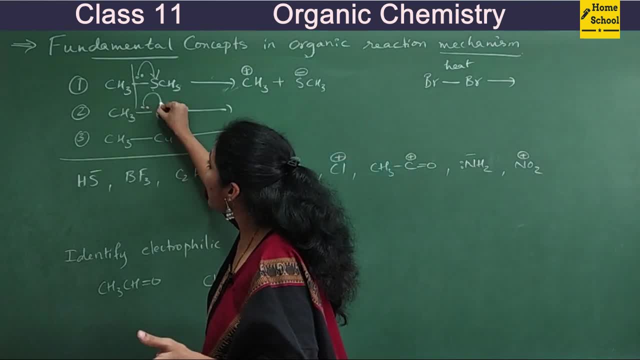 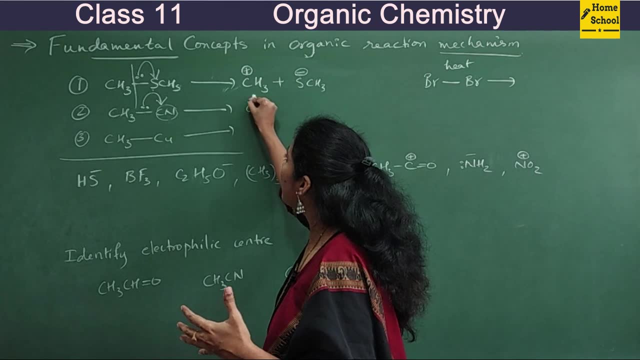 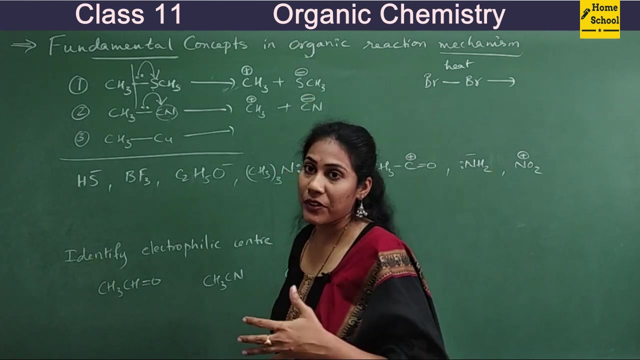 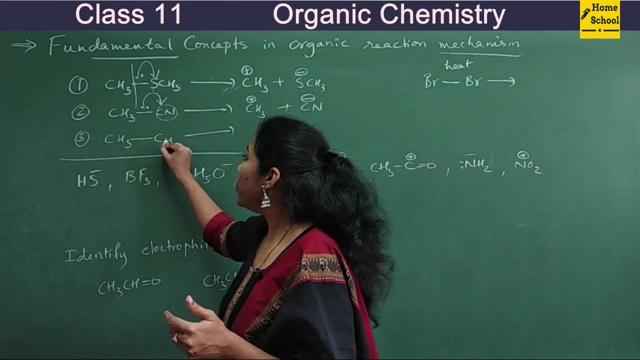 So here also heterolytic cleavage takes place and both electrons move towards CN group. So you will observe CH3 plus carbocation, methyl carbocation plus CN minus, Okay, cyanide anion. Okay. so here you observe CH3 bond CU. CU is less electronegative than carbon compared to CU Carbon. 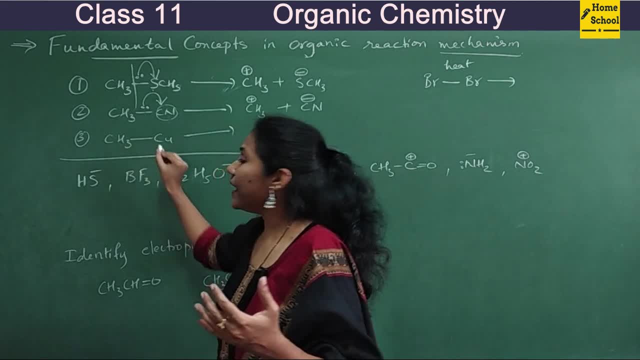 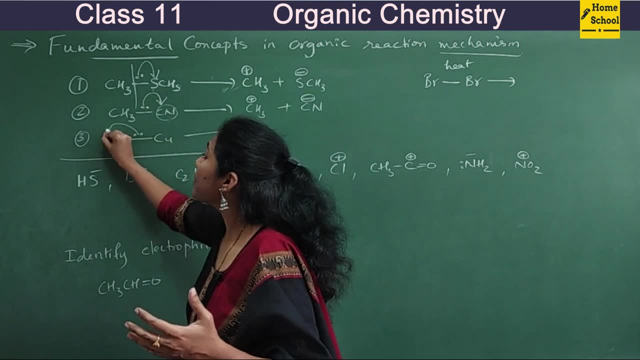 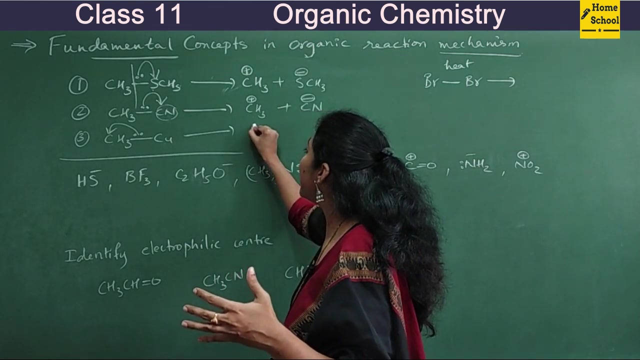 is more electronegative. So definitely there is a electronegativity difference. So the bond is cleaved heterolytically and both shared pair of electrons will move towards CH3. So you will have CH3 negative, negative charge on carbon. So here you will observe the formation of 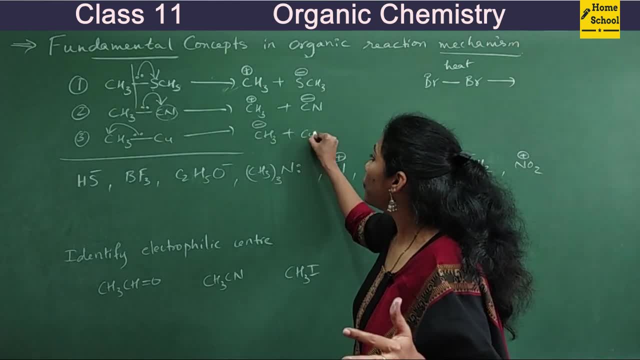 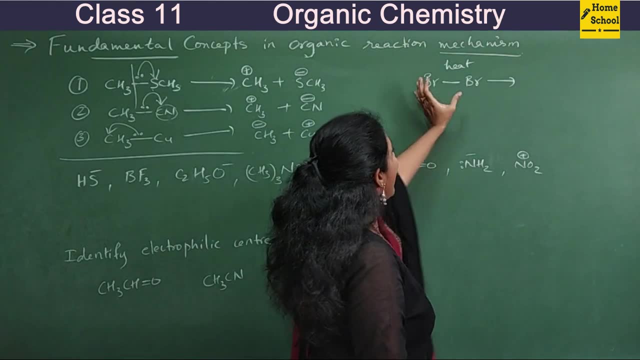 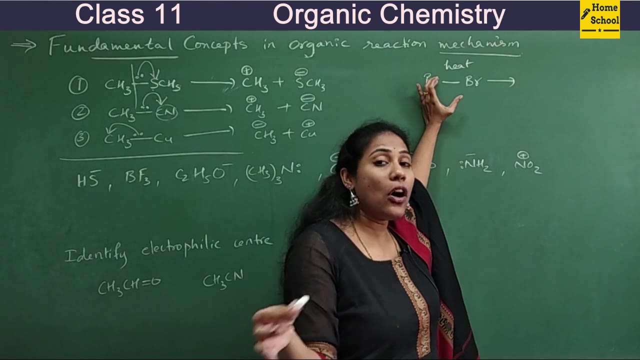 carb anion, Isn't it Plus CU on that positive charge? Okay, Coming, Coming to this, See, whenever you have similar electronegativity difference- BR, BR- there is no electronegativity difference. You can't call one BR is more electronegative, the other BR is less. 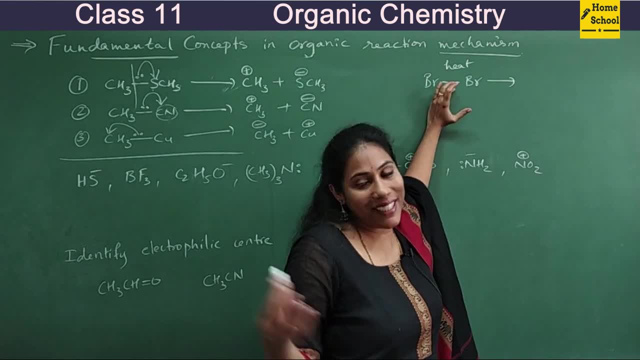 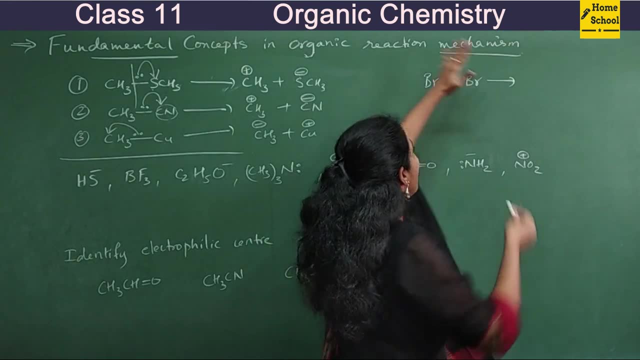 electronegative. Both belong to same element, right? They are of same type of atoms, So there is no electronegativity difference in such case. on heating: Okay, so when you heat them, or when you expose them to sunlight, homolytic cleavage takes place. 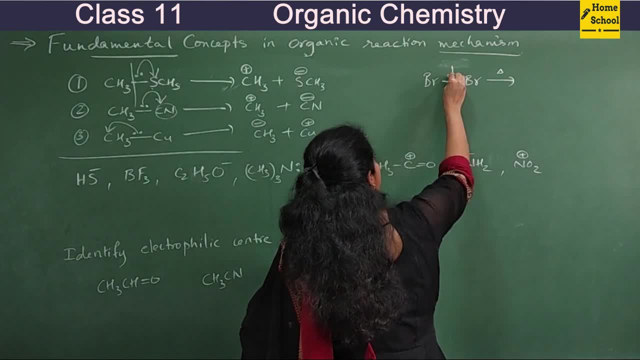 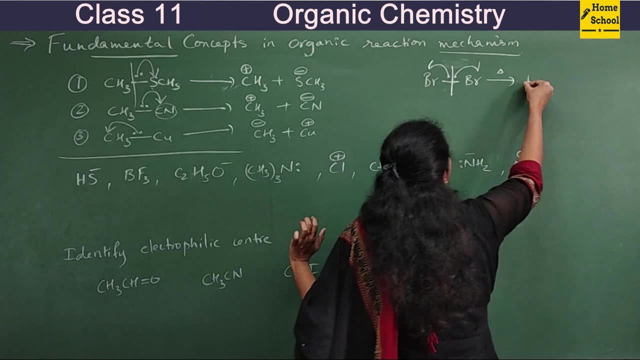 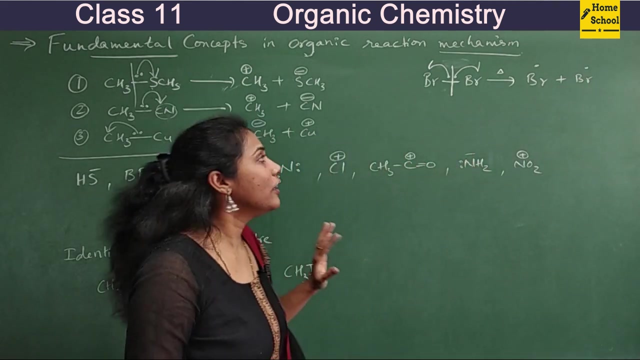 Okay, so homolytic cleavage in the sense what breaking in such a way that one electron goes to one atom, the other electron goes to another atom. So what do you get? You will get bromine free radical and other bromine free radical. Okay, so hope you understood like in which situation. 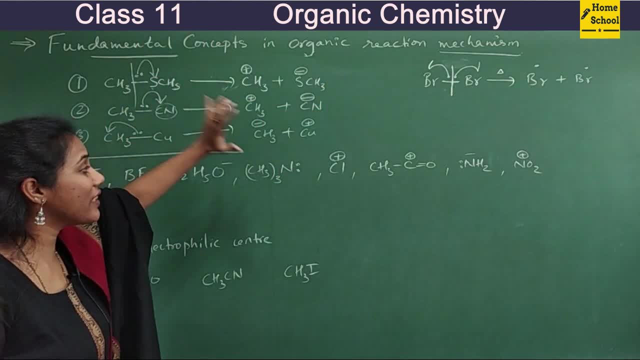 homolytic cleavage takes place and in which situation heterolytic cleavage takes place. Okay, So that is all about the first question. So see you in the next class. Bye, Bye question. coming to second question, there are certain species or ions given and you have to. 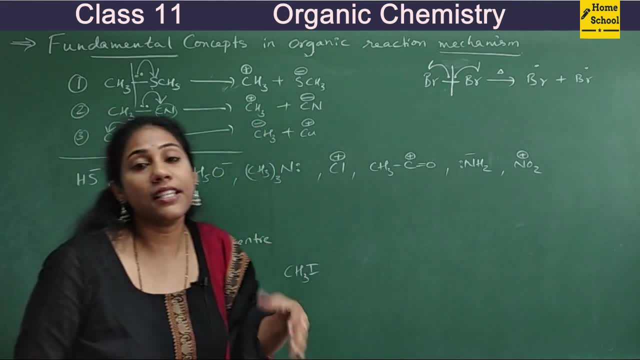 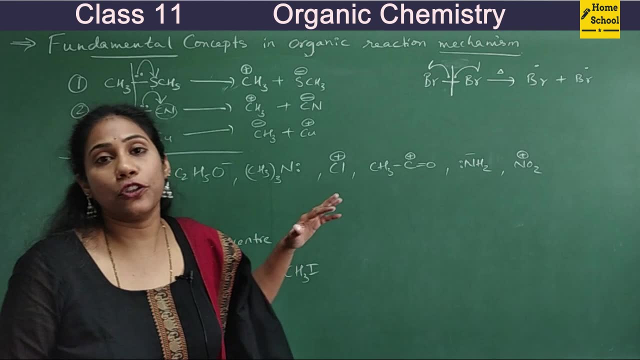 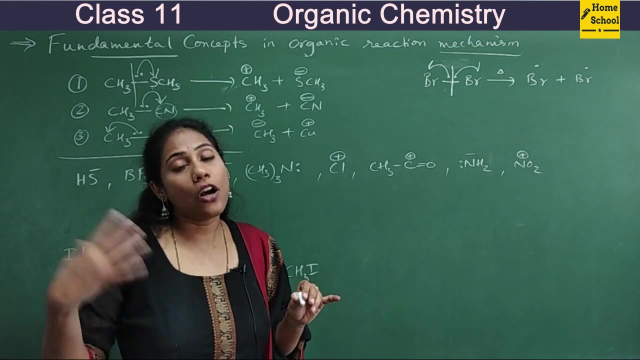 tell them whether the ion or species is nucleophile or electrophile. you should identify whether they are nucleophiles or electrophiles. so what do you mean by nucleophiles? electron rich species, negatively charged species or any neutral molecule with lone pair of electrons? what are 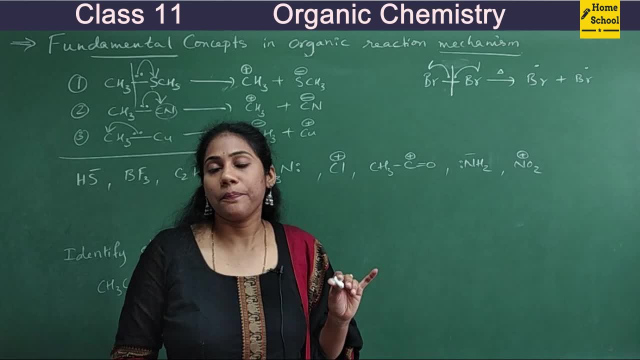 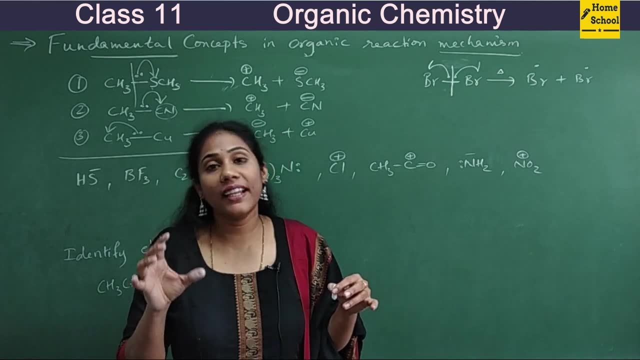 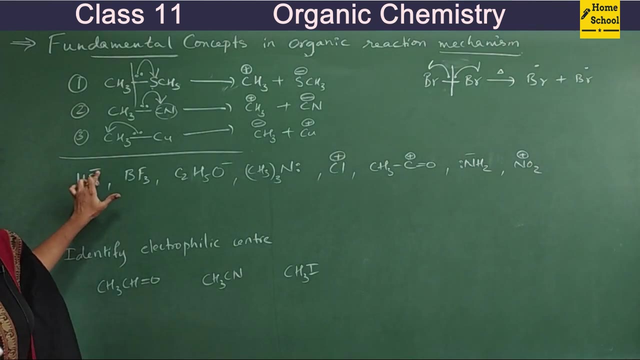 electrophiles, electron deficient species. that means any positively charged ion or a neutral molecule with electron deficiency. okay, let's identify hs minus say what i told you. negatively charged means they are electron rich. so electron rich in the sense this is negative charged ion or a neutral molecule with electron deficiency. 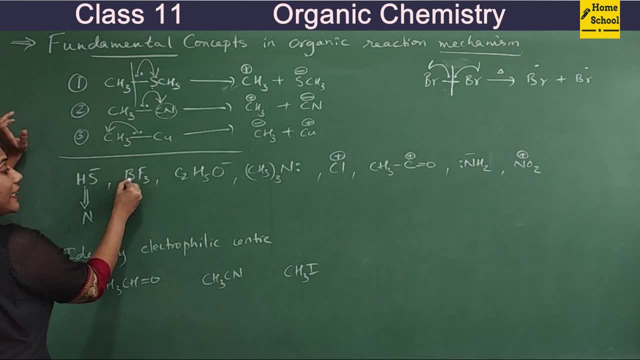 nucleophile. this can act as a nucleophile bf3 b. it has only six electrons around it. two more electrons are necessary for this guy to have an octet. so this has electron deficiency in the molecule. so i can call this as electrophile c2h5 o minus. whenever you see minus, no doubt it is a. 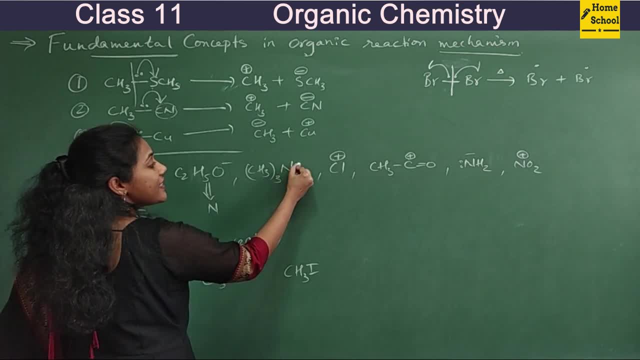 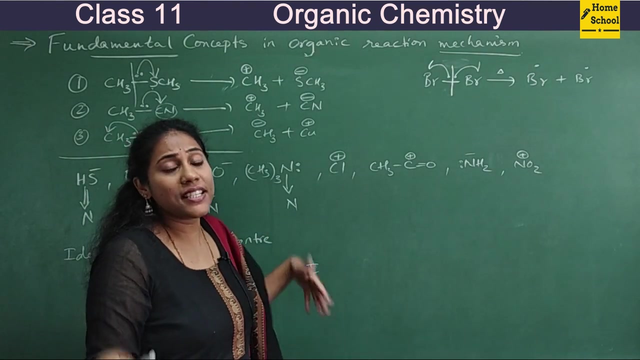 nucleophile ch3 thrice and see there is a lone pair of nitrogen. so this is electron rich guys. even a neutral molecule with a lone pair can be called as nucleophile. and what about this? anything with a positive sign means it is not having enough electrons and it is eagerly waiting for the 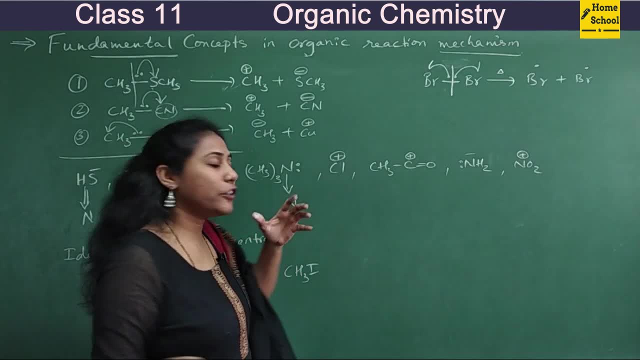 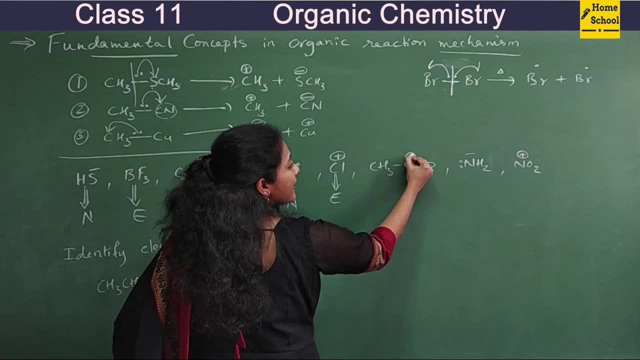 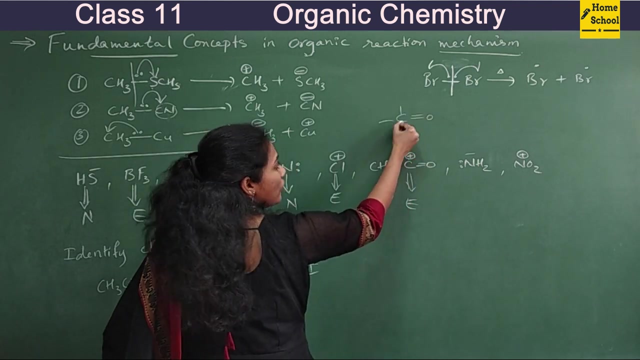 electrons to have. so such a species are called electrophiles. so this is definitely an electrophile. and this one c double bond, o positive- there is a positive charge in carbon. definitely this is electrophile. you know what, whenever you have this situation in organic molecules, you can call it. 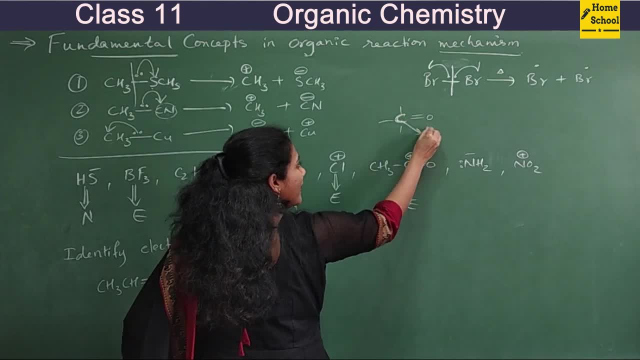 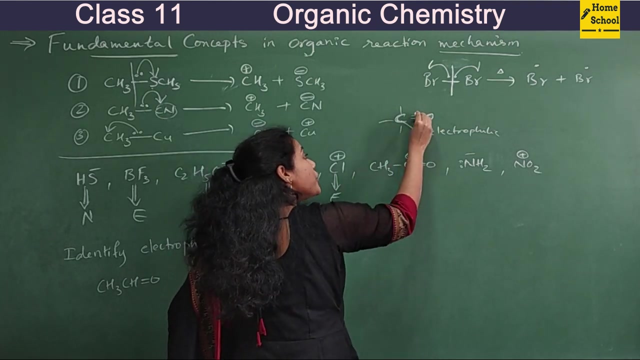 a molecule such a carbon. this carbon is always electrophilic in nature. okay, why it will act as electrophilic in nature? because it is bonded to oxygen. oxygen is more electronegative, so you have a chance of shifting this pi bond towards oxygen. okay, always one of the pi bond you know always. 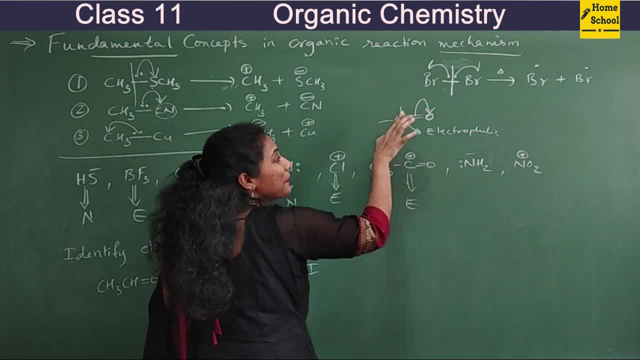 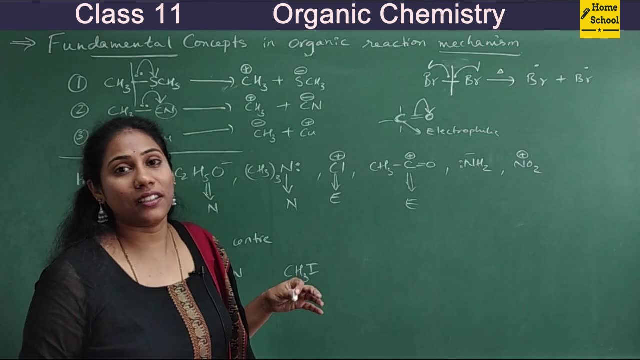 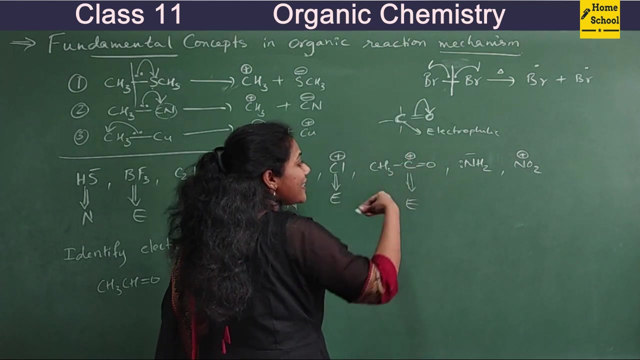 wants to move towards oxygen, so making this carbon electron deficient. So I say this carbon is electrophilic in nature. okay, So that's why, always whenever C double bond O, that particular C has a tendency to lose electrons. you know that is always electrophilic. 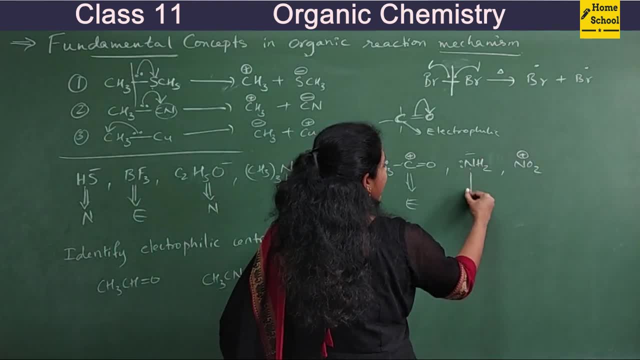 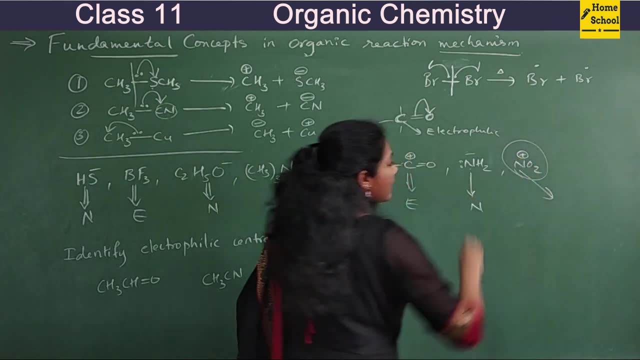 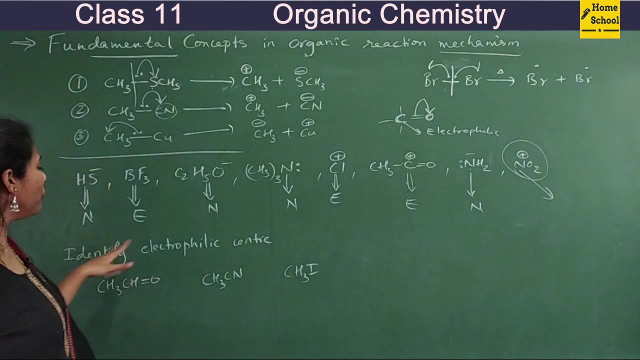 right. So this is electrophile and NH2 with minus sign it is nucleophile. So this one, tell me whether this is electrophile or nucleophile. comment your answer in the comment section. okay, Don't forget. Coming to next question, you have to identify electrophilic center. 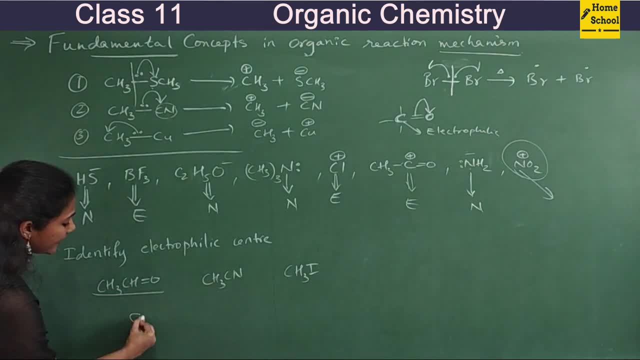 okay. So you see this compound. if I have to write this elaborately, CH3, C. C has a double bond with O and C has one more hydrogen. I'll write here. So here among the two carbons, 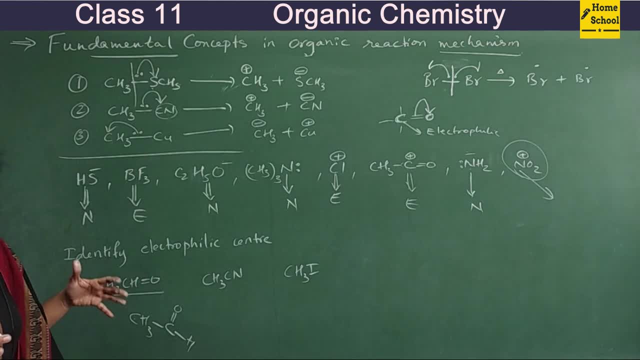 can you tell me which is electrophilic? Electrophilic means slightly electron deficient. definitely this carbon, right? Because this is bonded with oxygen. So you have a chance of moving this pi bond towards oxygen. okay, So always, oxygen attracts a bond because it is more electronegative than carbon. 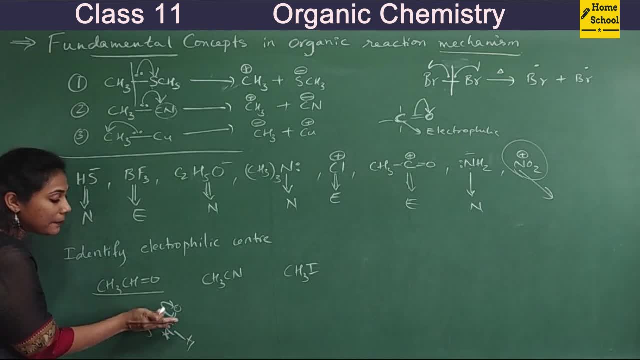 So this bond doesn't completely belong to carbon, but that is more near to oxygen. So this carbon is electrophilic, we say that means it has slightly electron deficient nature. okay, So that is why this carbon is electron deficient. And coming to this molecule, if I have to write, 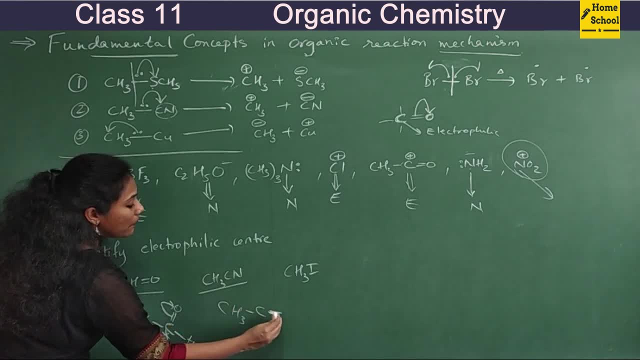 elaborately CH3, C, and you have a triple bond between carbon and nitrogen. So among the two carbons, which is electrophilic, You see again, nitrogen is more electronegative. no, So one of. 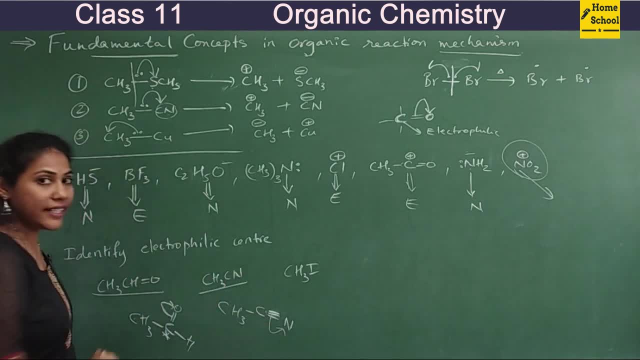 the bond has a chance of moving more towards nitrogen, making this carbon less electron deficient. So this is why this carbon is electrophilic. And coming to this molecule, if I have to write elaborately, CH3, C and you have a triple bond between carbon and nitrogen. So 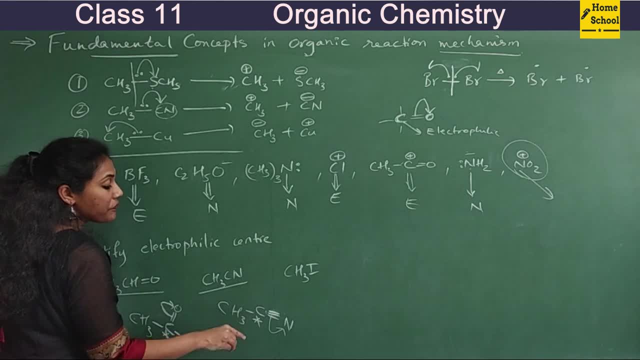 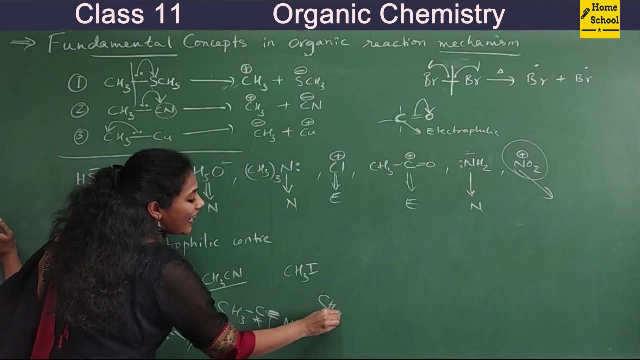 you can see that the form is定 kitten is a sort of an electron deficient. okay, Right, Less electron thing. So that's why this carbon is electrophilic. Coming to this case, CH3I, So there is a bond between carbon and iodine. Iodine is more. 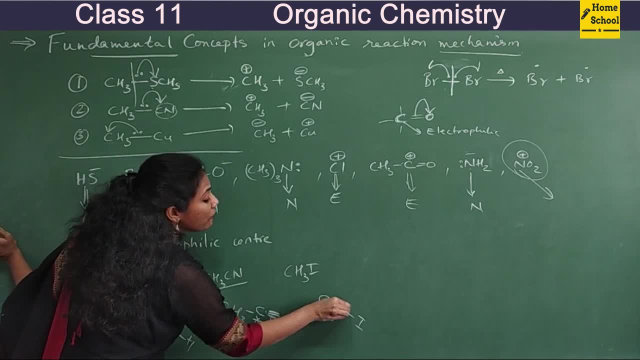 electronegative? no So slightly. the bond will move more towards iodine. If a bond breaks, the bond will move to iodine right, Making this carbon electrophilic. So if bond is cleveed atrial, 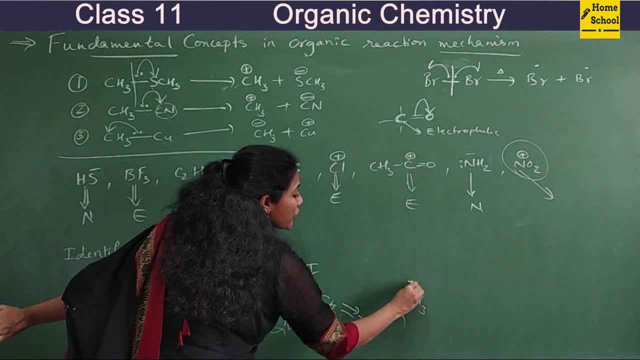 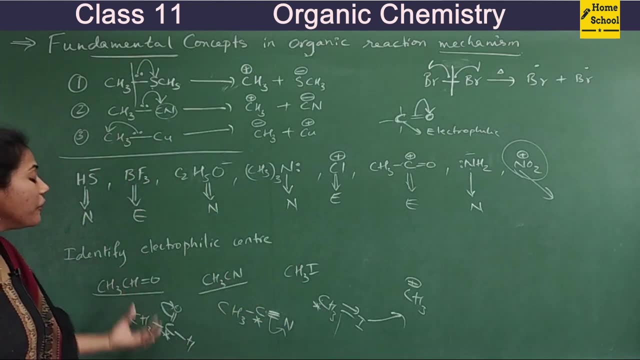 little bit. then, on the other hand, if there is a bond with barrier, it has to move toward one of the titles in the next chance. what do you get? you will have CH3 positive only. so this carbon is electrophilic in nature. okay, so identifying which carbon in a organic molecule is electrophilic is very, very. 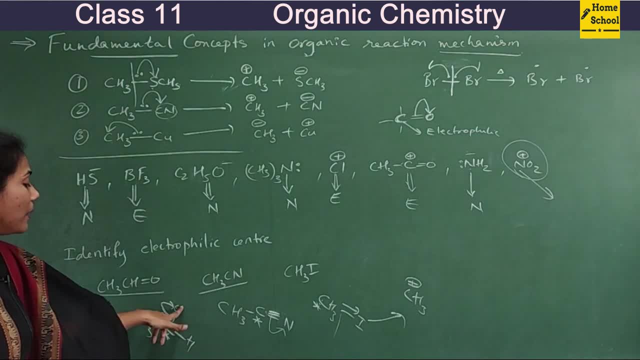 important always, when you have a carbon with double bond O, then such a carbon is electrophilic- CN- okay, nitrogen, more electronegative, so such a carbon is also electrophilic, okay, and here, in this situation also the carbon is electrophilic. so in general, what I want to tell you is: in any 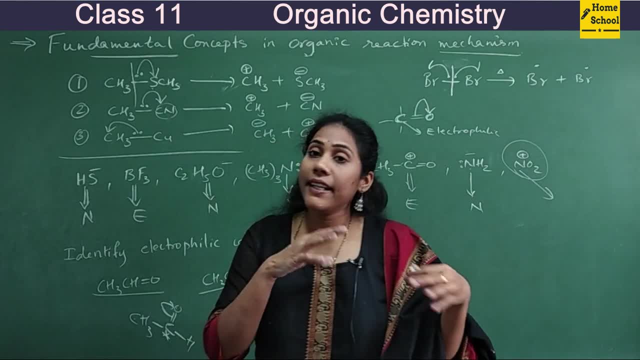 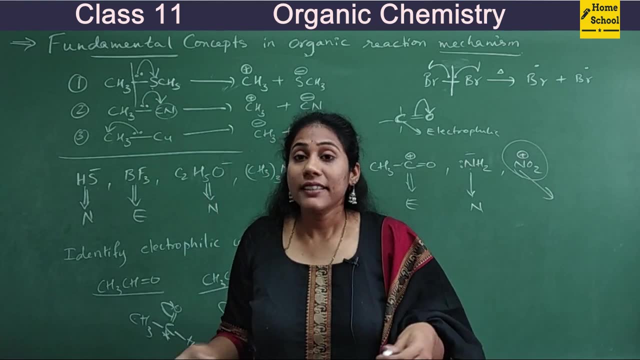 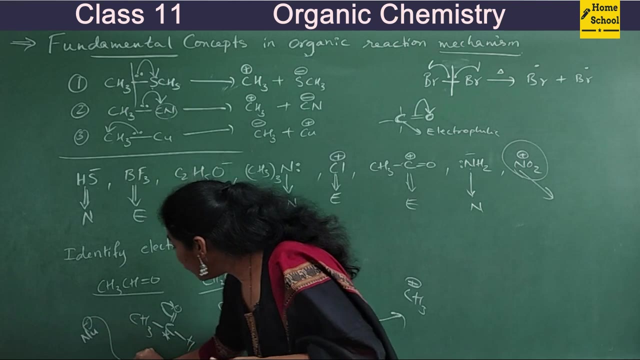 organic molecule. if a carbon is bonded to any electronegative element, then that carbon will become electrophilic, electron deficient center. that means if any nucleophile is there around this, the nucleophile where will it go and attack? it will attack this carbon because it's a nuclear. 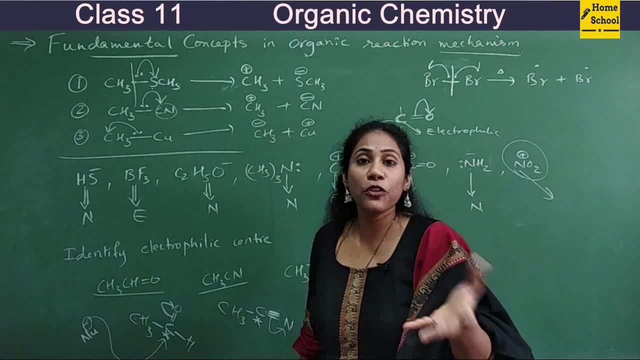 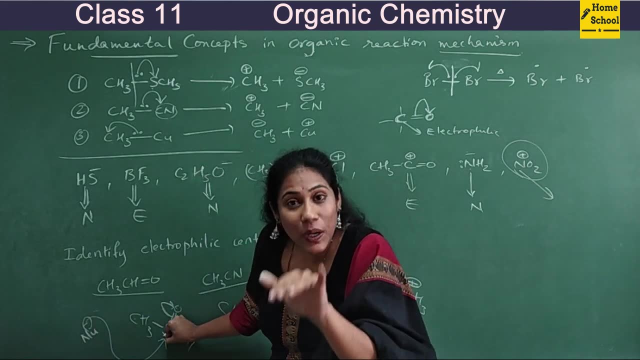 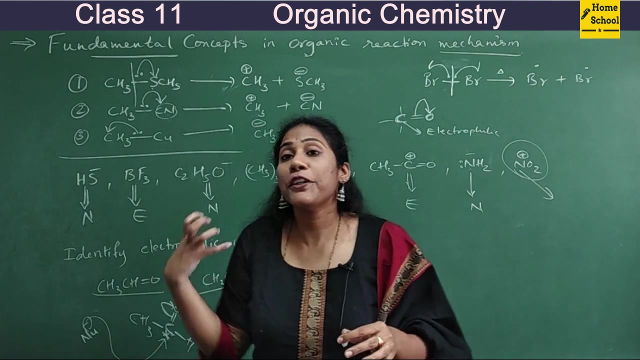 I told you, or the organic reaction is always between nucleophile and electrophile. so nucleophile is electron rich guy. where will it go and attack? it will attack electron deficient guy who is electron deficient in a molecule, this carbon. okay, so identifying electrophilicity or nucleophilicity of a atom. 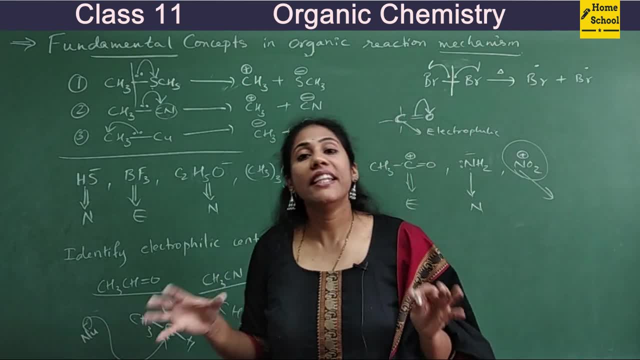 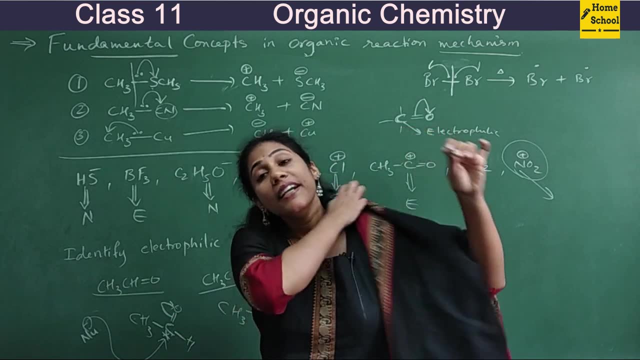 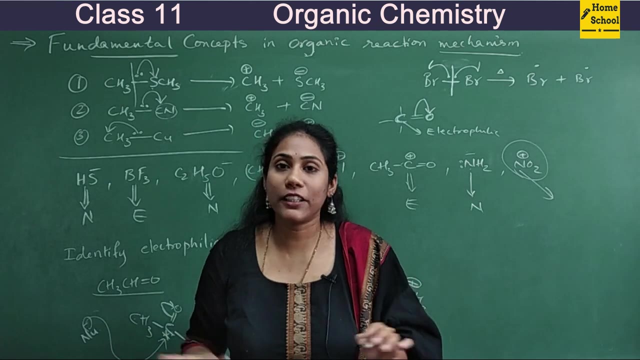 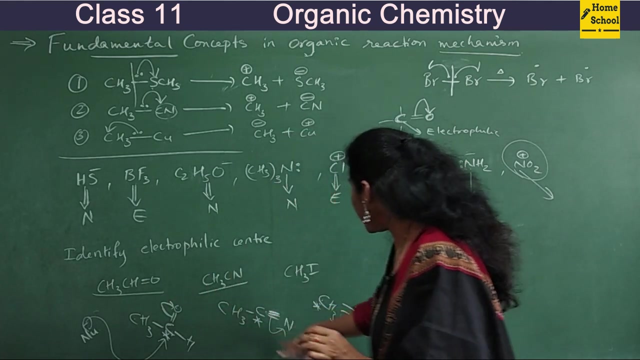 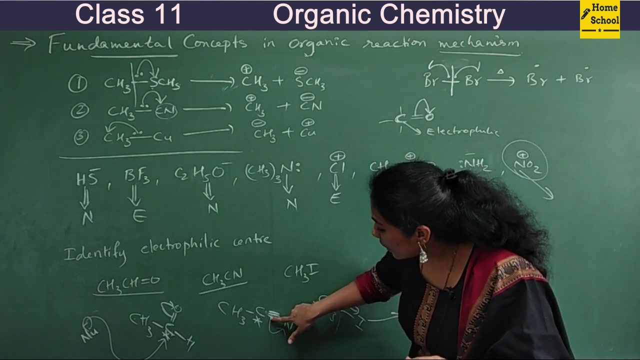